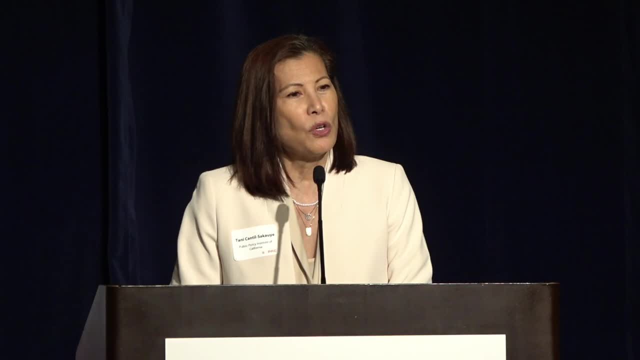 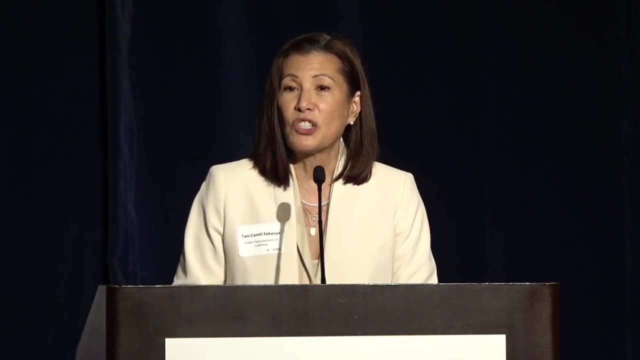 To focus on the business and the employees who drive our economy, As well as to identify realistic solutions to the challenges they face. So soon as I pointed out, you will hear a video or see a video from Dr Bone. But before we start officially, I have a few announcements. 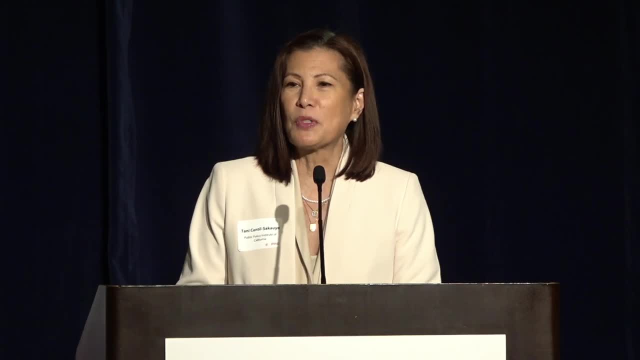 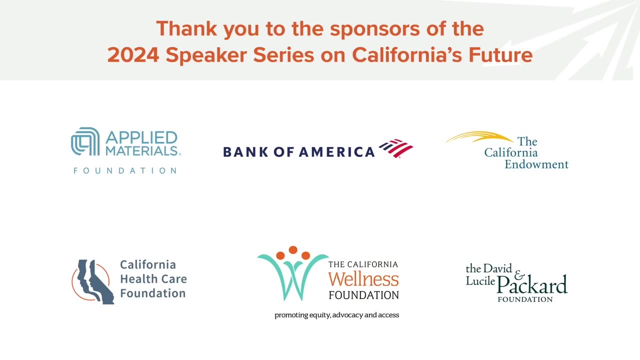 And the first is the fact that we're able to open this up to the public gratis, here in person and online is thanks to our generous sponsors, Who you'll see that are on our screen as well as on a list on your table. 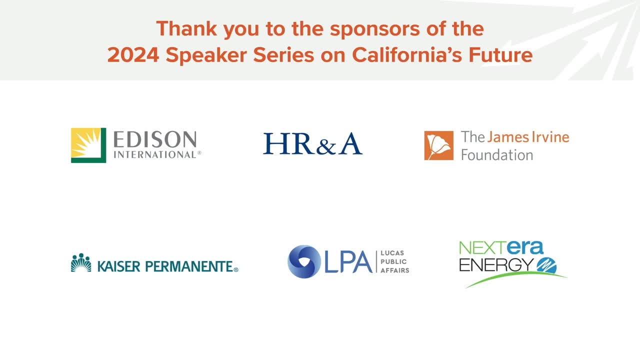 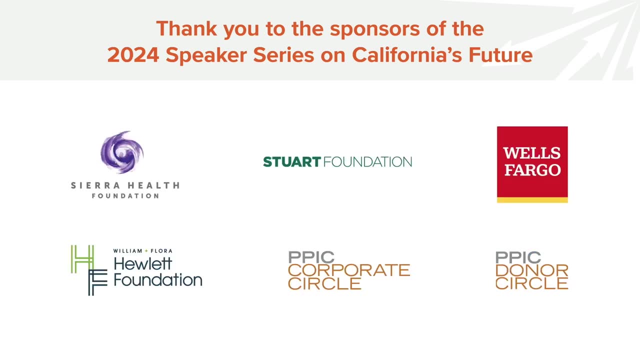 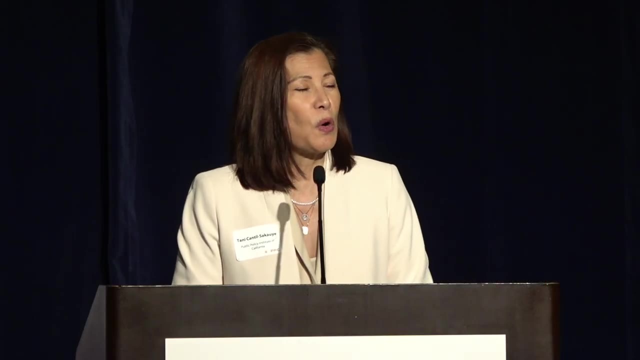 We also have support for the Speaker Series event from our donor circle and our corporate circle, And these sponsors and donors truly understand the need for objective data that informs the policies of California. We thank them. We invite you to go to our website to see the full list. 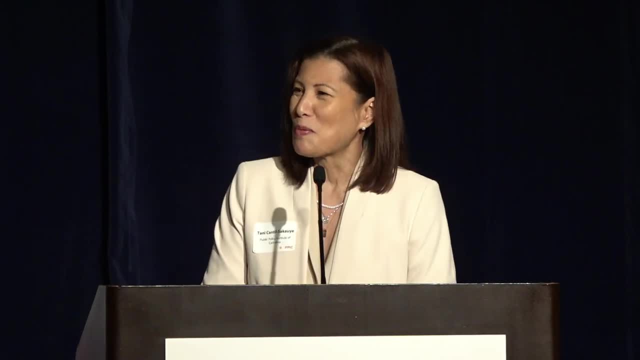 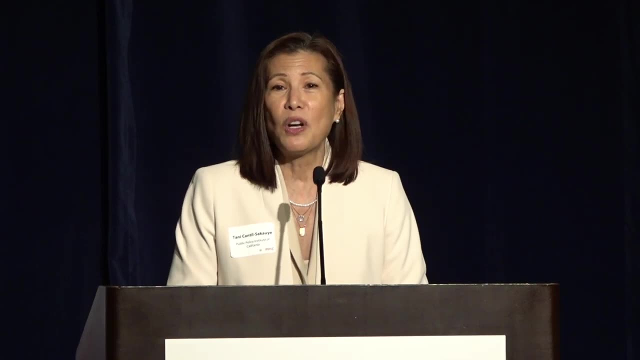 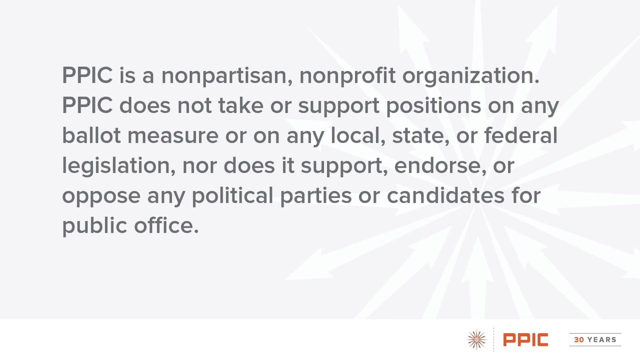 And to consider yourself as a sponsor or donor or supporter of PPIC. Also, PPIC is a charitable trust And that basically means we do not endorse, support, lobby for ballot initiatives, specific pieces of legislation or persons running for office. 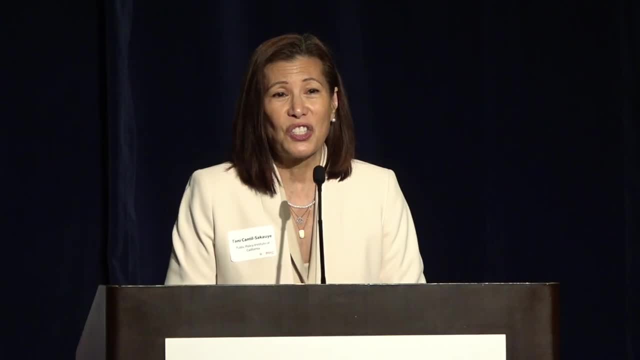 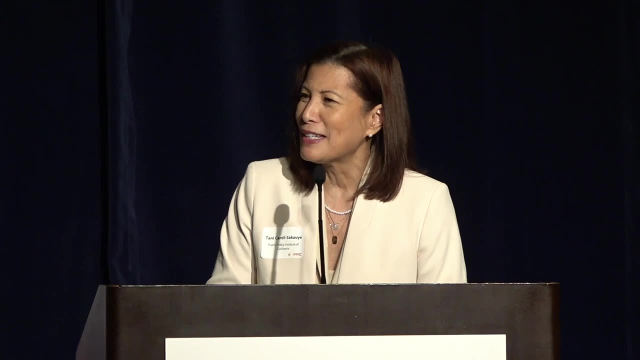 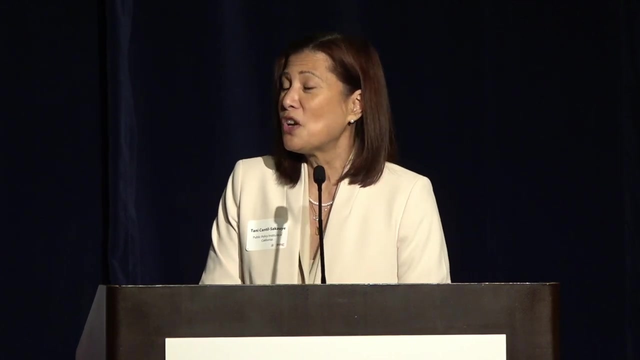 So today, while we all have time with this distinguished panel, we also provide an opportunity for a little democracy: 45 minutes of Q&A from the audience and from our online audience, And so we ask that, when you do wish to speak, raise your hand, state your name and your organization, if you have one. 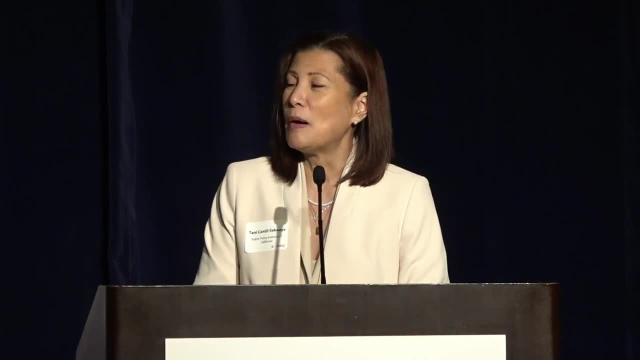 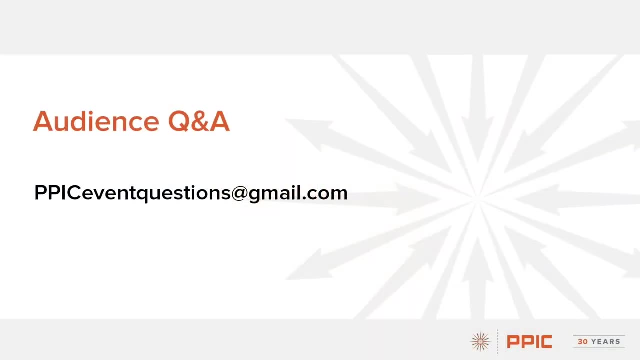 and a member of our PPIC staff will provide a microphone for you to ask your question. Also, for those of you online, please send an email. You'll hear it from me, you'll see it on the screen and we'll remind you later. 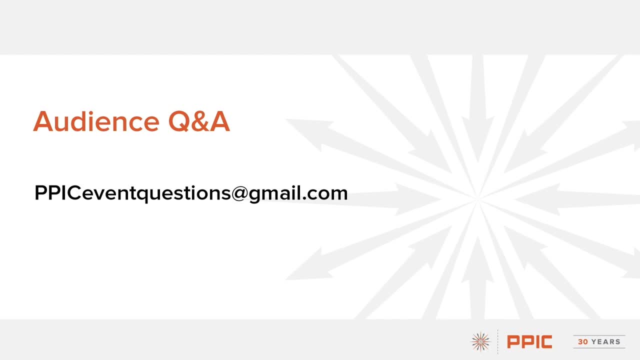 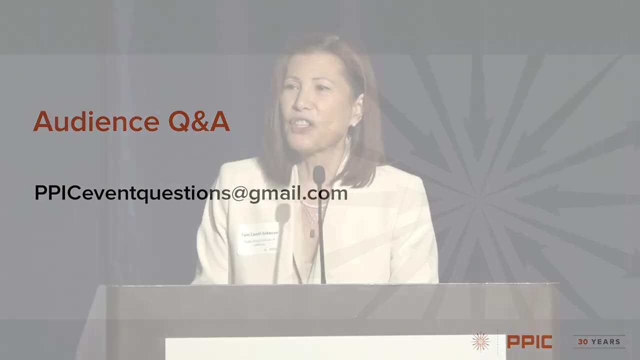 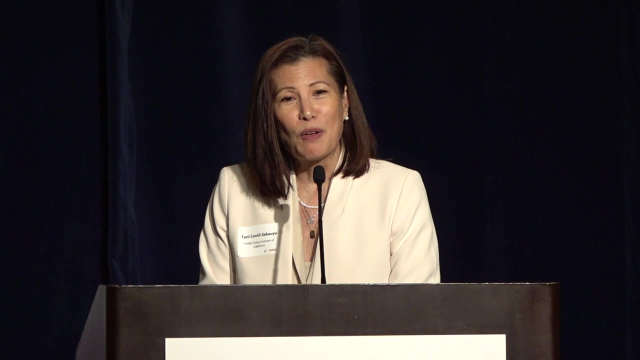 It's at ppiceventquestions at gmailcom. Also, please include your name and organization, if you are, if you have one. Lastly, you hear this everywhere. Please silence your cell phone Now. I am about to show you this short video from Dr Bone, our director. 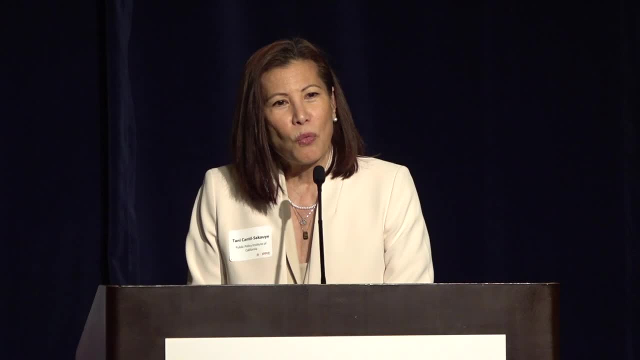 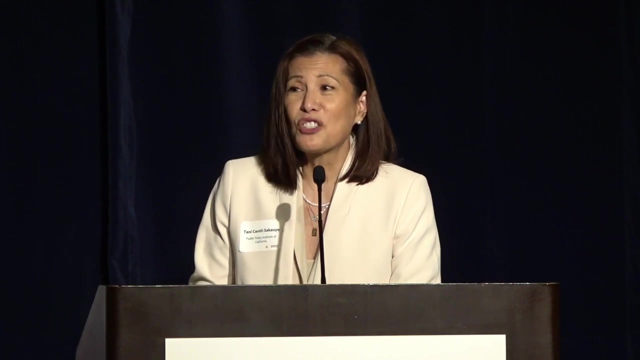 but I do want to say something about our distinguished panel. We have are lucky to have leaders in their fields, people who talk and influence and study our economy in California. We are also delighted to have Kai Risdahl of Marketplace Now, because this is a diverse audience of different ages. I'm just going to tell you. 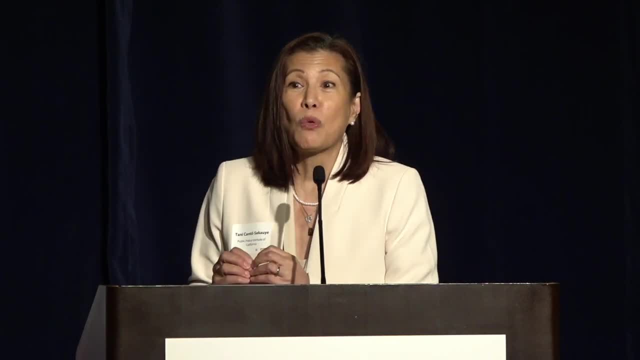 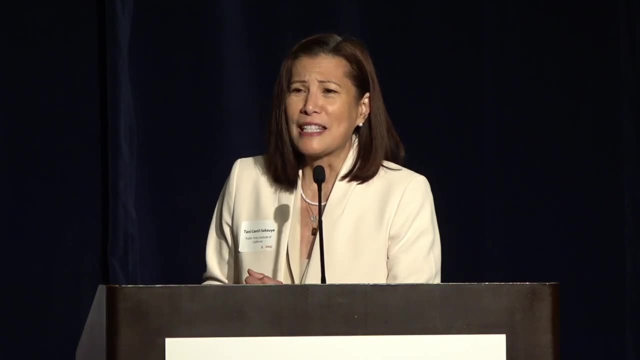 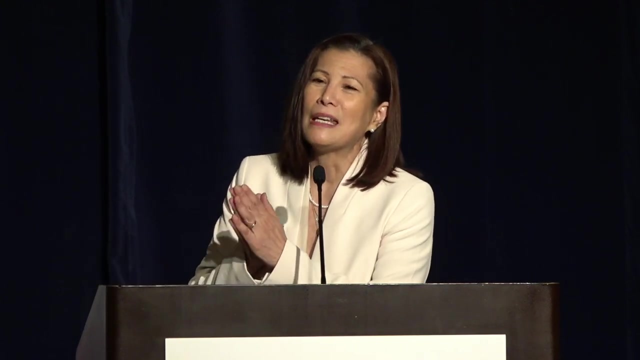 Marketplace is the radio and podcast that will make you feel smarter than you are. You don't need an econ degree as it's advertised. Kai Risdahl has been the host and editor since 2005.. Emmy award winning, really public figure in business and economy in the country. 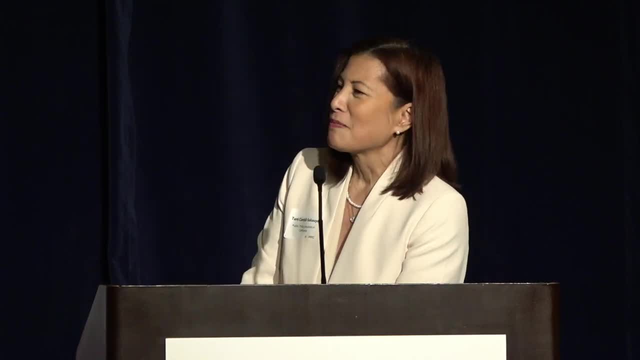 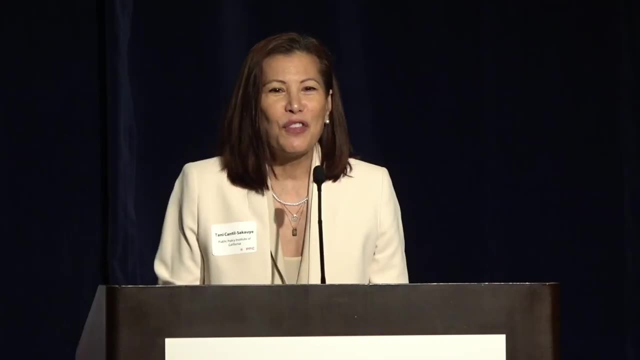 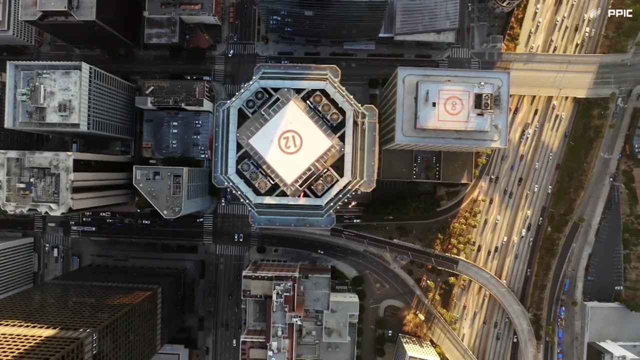 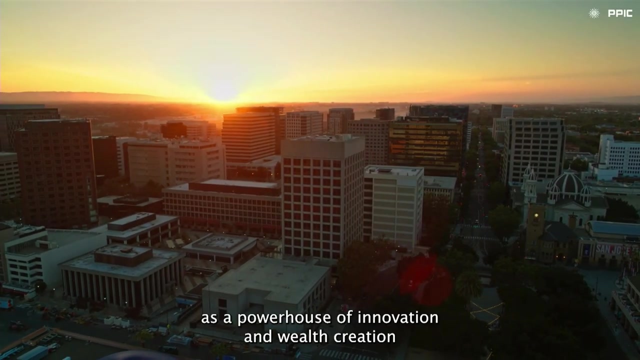 We are delighted and pleased to have you, sir. Thank you, And now the video. Over the past century, California has established itself as a powerhouse of innovation and wealth creation, and we have great potential to address the changes facing our state's economy. 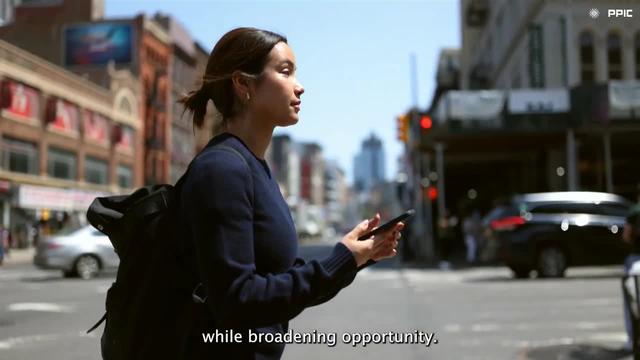 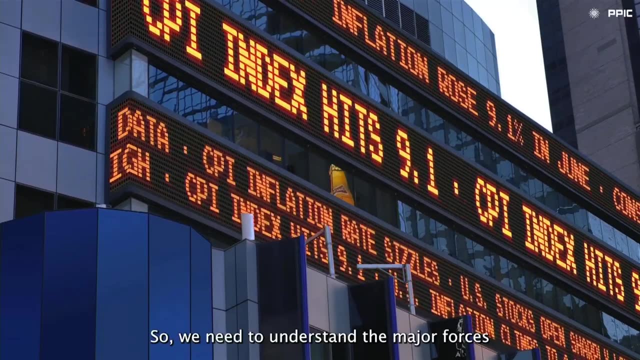 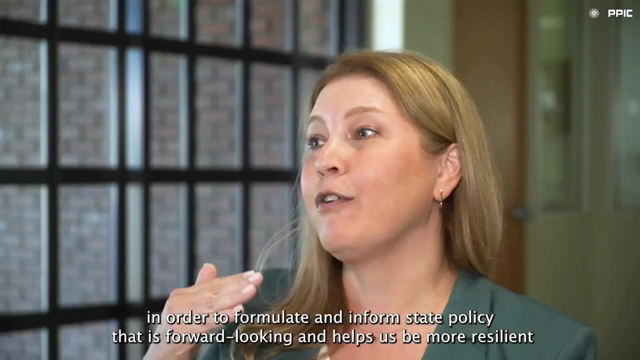 while broadening opportunity. The reality is we've weathered a lot economically speaking over the past few years, So we need to understand the major forces that are reshaping economic opportunity in the state in order to formulate and inform state policy that is forward-looking. 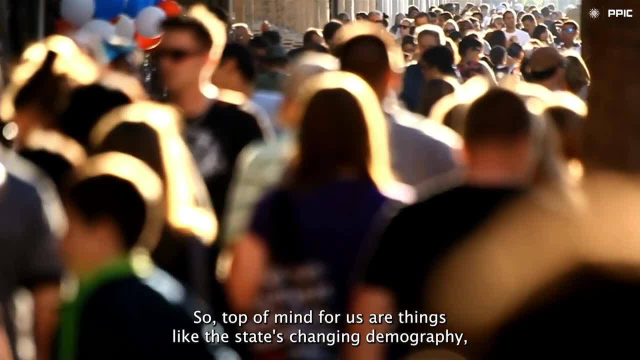 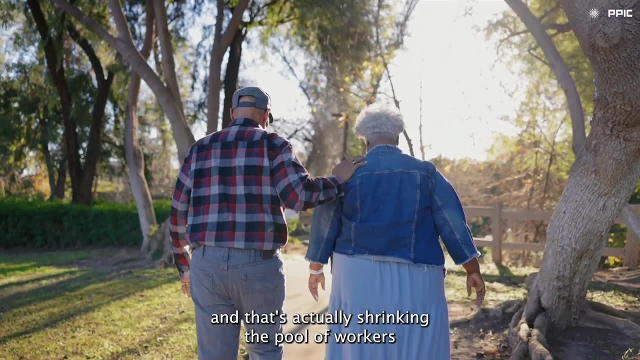 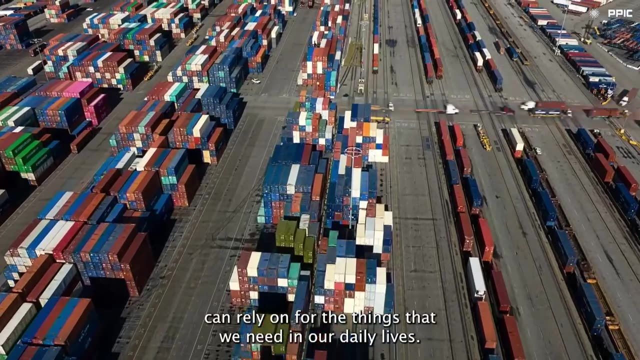 and helps us be more resilient going forward. So top of mind for us are things like the state's changing demography, the fact that we're aging and that's actually shrinking the pool of workers that businesses have to draw from and that we, as Californians, can rely on for the things that we need in our daily lives. 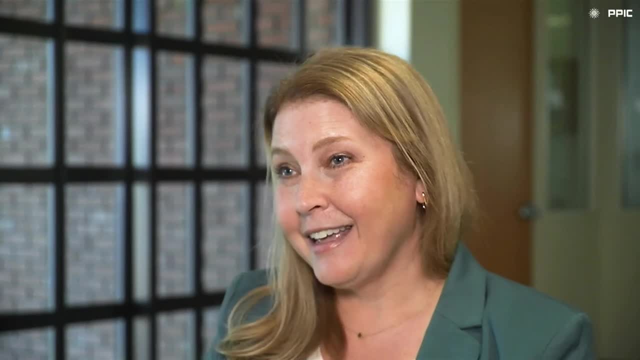 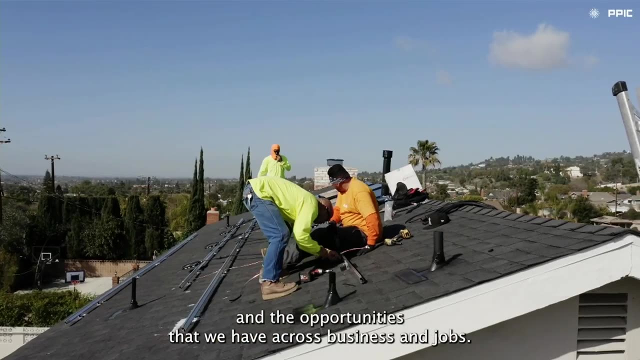 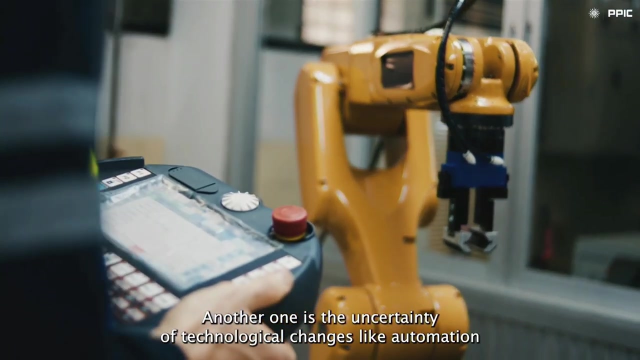 Another major force is the role of climate and how the increasing likelihood of major climate events affect economic activity and the opportunities that we have across business and jobs. Another one is the uncertainty of technological changes like automation and AI. The pandemic changed how a lot of people work, where they work. 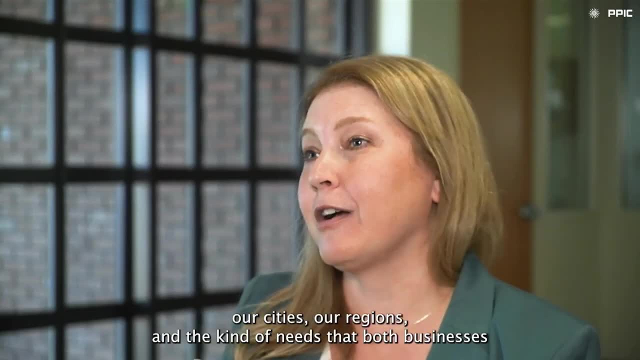 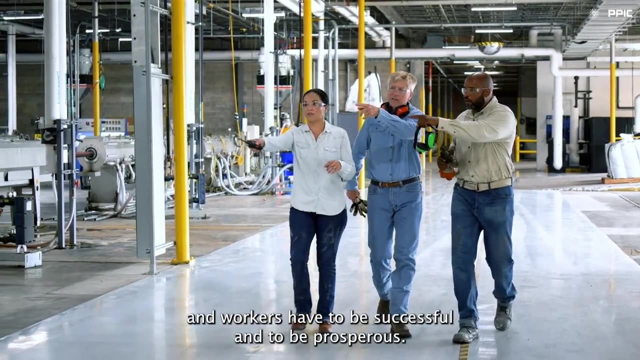 and that's going to have implications for our labor market, for our cities, our regions and the kind of needs that both businesses and workers have to be successful and to be prosperous. These are all real forces that California's families, its businesses. 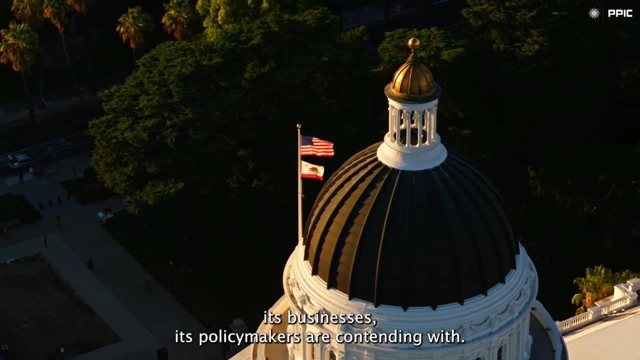 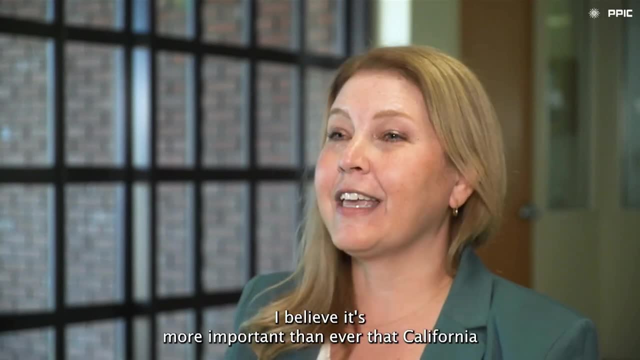 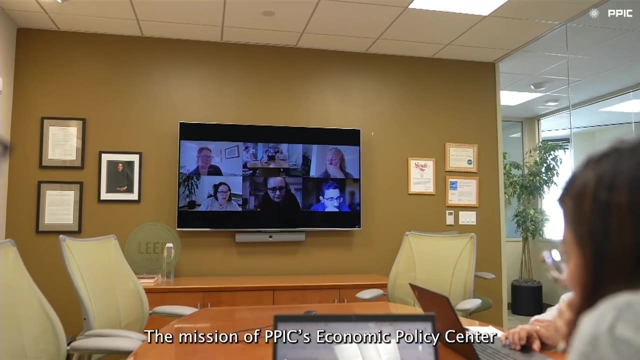 its policymakers are contending with. With the present economic challenges, as well as new ones on the horizon, I believe it's more important than ever that California ensure that all of its people can thrive economically. And that's where we come in The mission of PPIC's Economic Policy Center. 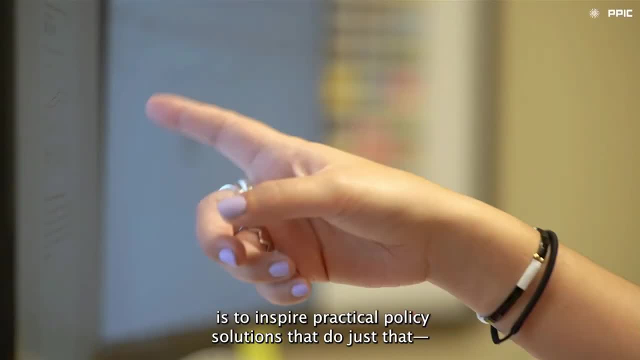 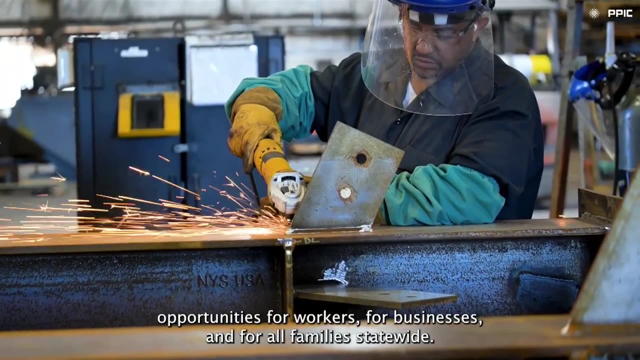 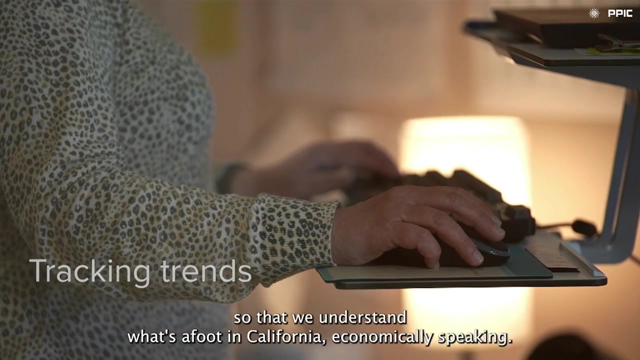 is to inspire practical policy solutions that do just that, that help create a robust, resilient economy that increases opportunities for workers, for businesses and for all families. statewide, We will be tracking trends so that we understand what's afoot in California economically speaking. 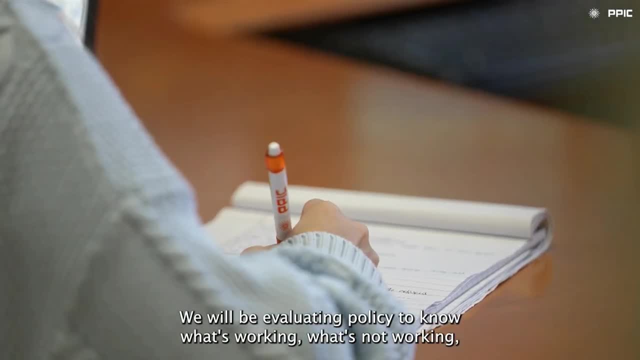 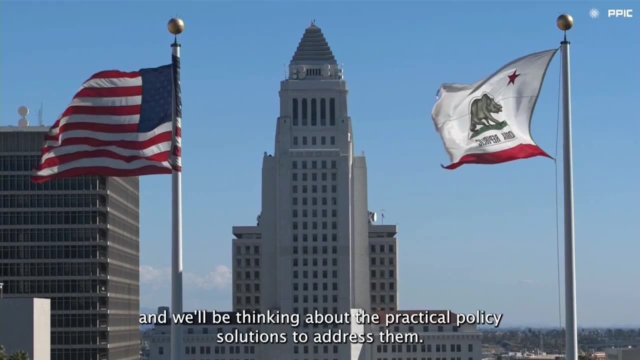 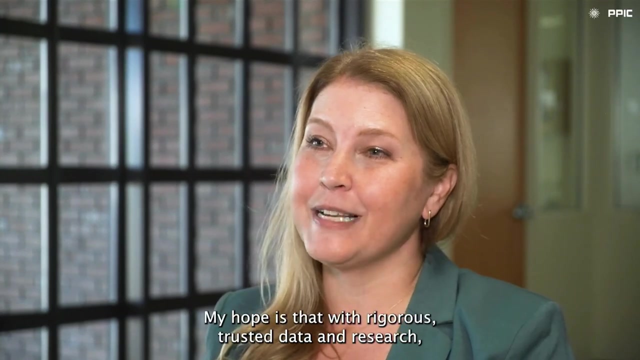 We'll be evaluating policy to know what's working, what's not working and what potential solutions are out there, And we'll be identifying barriers to advancement And we'll be thinking about the practical policy solutions to address them. My hope is that with rigorous, trusted data and research. 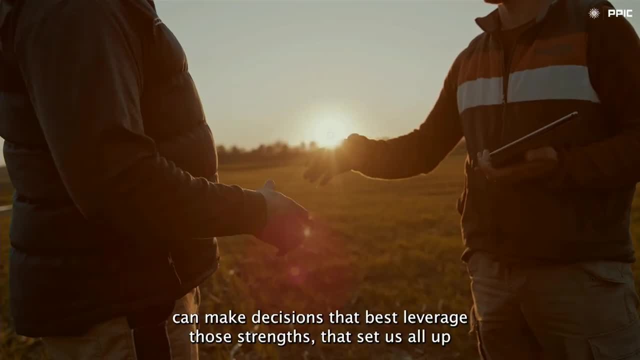 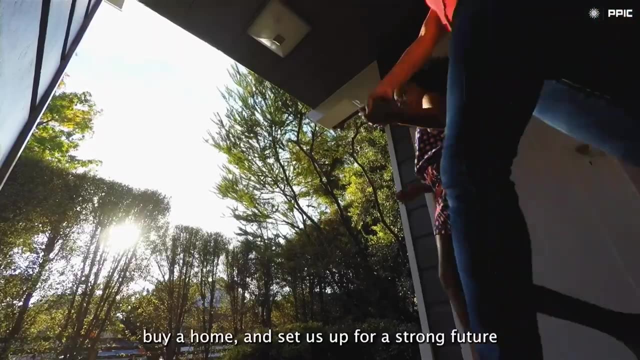 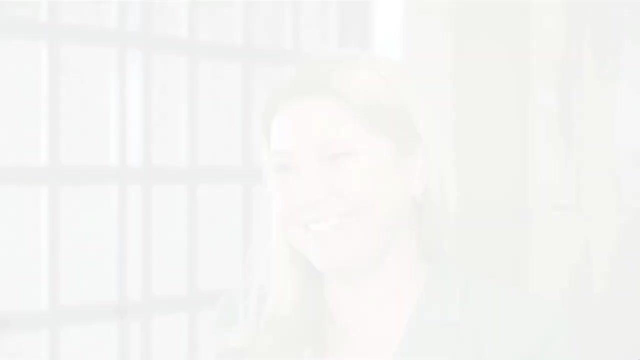 the state's leaders and its people can make decisions that best leverage those strengths that set us all up to secure that good job, build a successful business, buy a home and set us up for a strong future where all can thrive economically. Thank you, 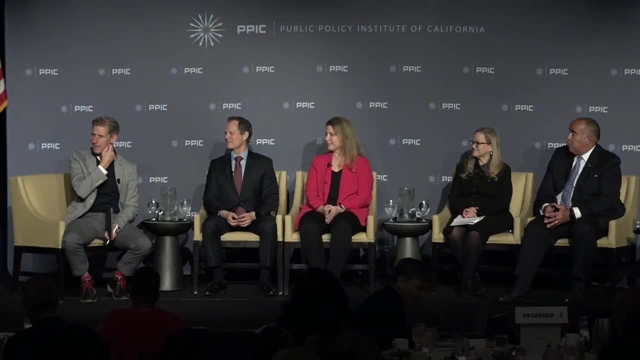 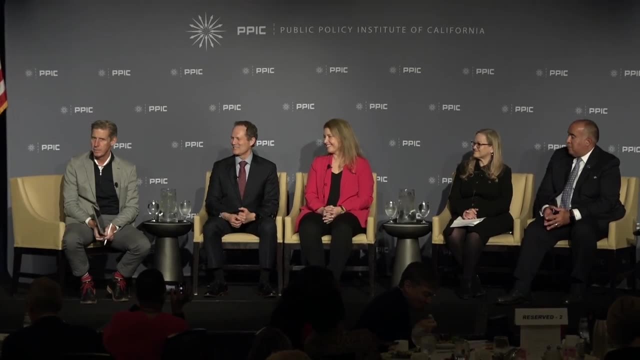 Thank you all for coming. I appreciate you taking time out of your busy days on a day, frankly, where it's colder in Sacramento than it is in Los Angeles. you know whatever to participate in this really important panel, And when I say participate, there will be a chance at the end. 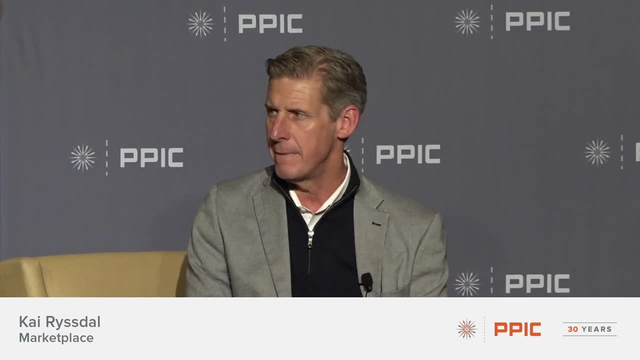 We're going to go half an hour, 40-ish minutes, and then I'm going to open it up. There will be, as Tawny said, mic runners. They will come to you, They will hold the mic, so don't get carried away. 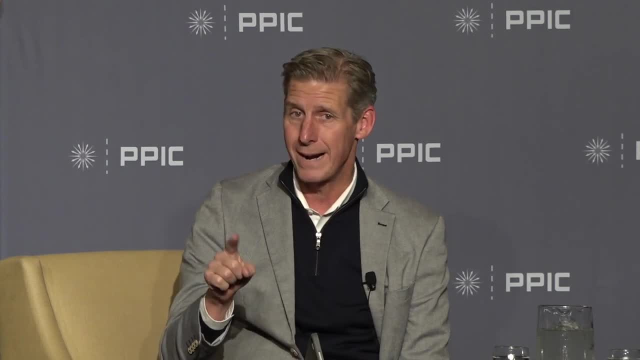 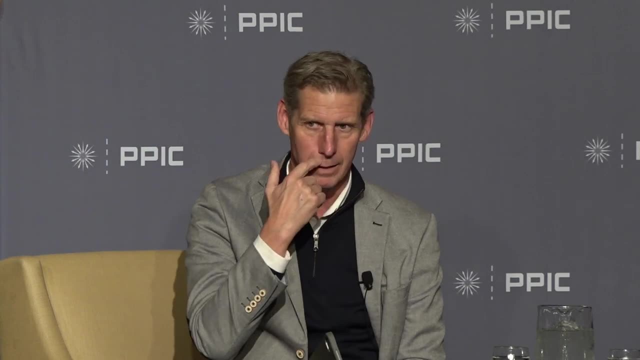 Also, I would encourage you that questions from the floor end actually in a question right, And let's keep them brief so that we can get as many people in as we can. That applies online as well. We'll do a very brief introduction. 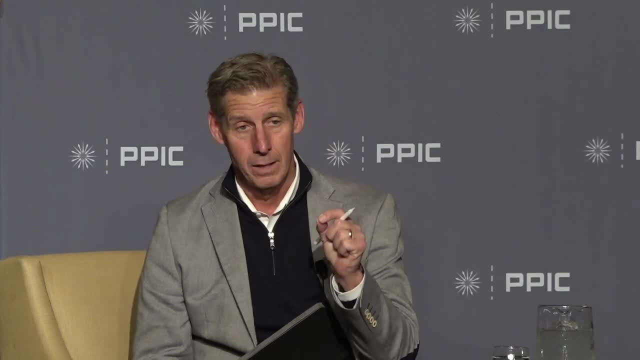 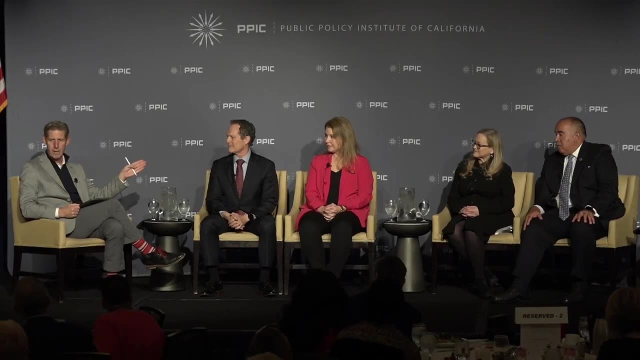 and then we're going to get going because we have a lot of ground to cover and not a whole lot of time. Ruben Barrales, Senior Vice President for External Relations at Wells Fargo, also formerly of the San Diego Chamber of Commerce via the George W Bush administration. 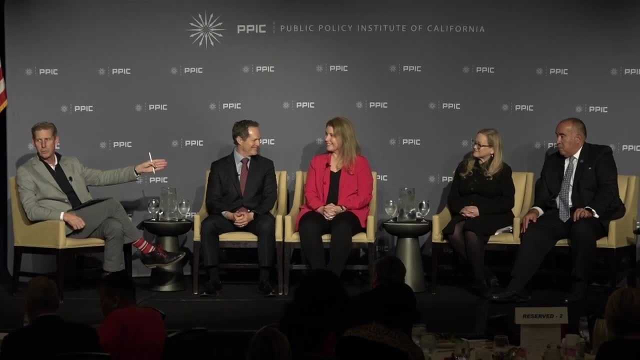 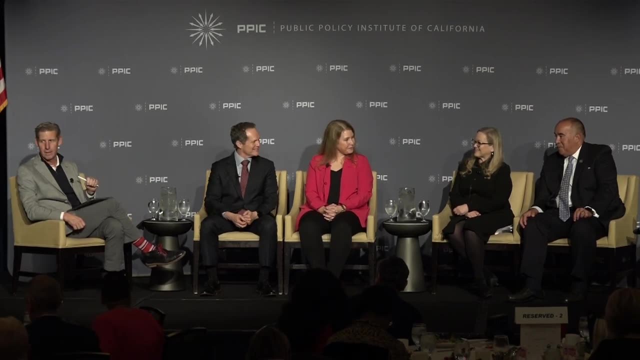 the George W Bush White House. Sarah Bone is the actual economist on this panel, so if you have actual economic questions, direct them to her. Cindy Chavez from the Santa Clara County Board of Supervisors. Before that, the San Jose City Council. 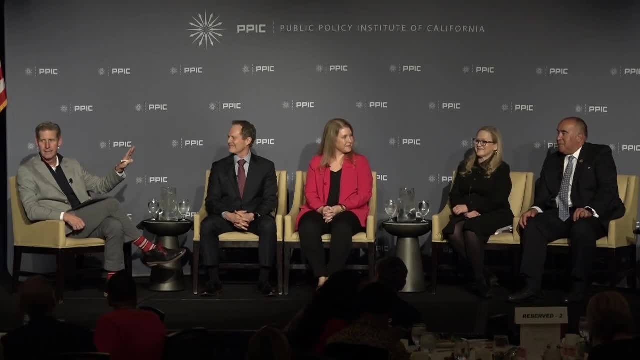 Before that, the Vice Mayor. She's done everything in politics that you can do at the local and county level. And then, of course, Paul Granillo from the Inland Empire Economic Partnership doing regional work- so important down there Quickly because we have a lot to get through. 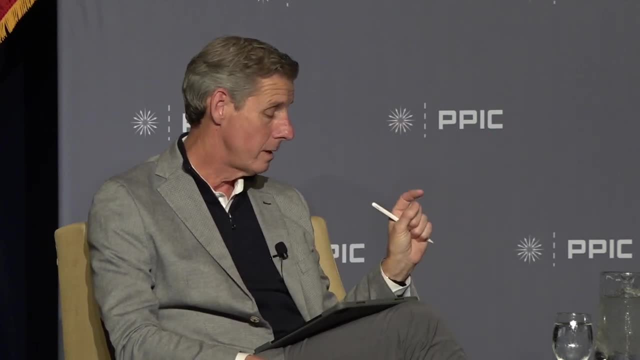 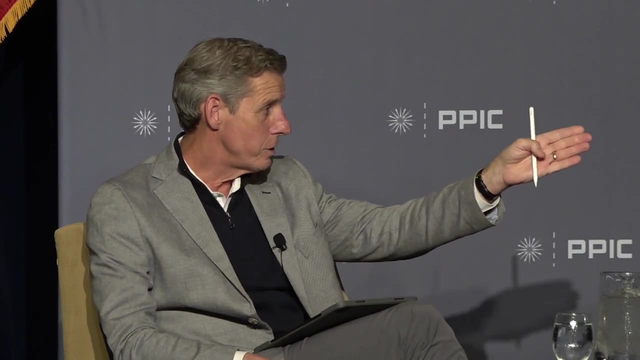 and this is the only time I'm going to go in a row, except Sarah, I'm going to leave you for last. In your area of expertise, which is to say business, government and regional issues define the California economy right now, as you see it. 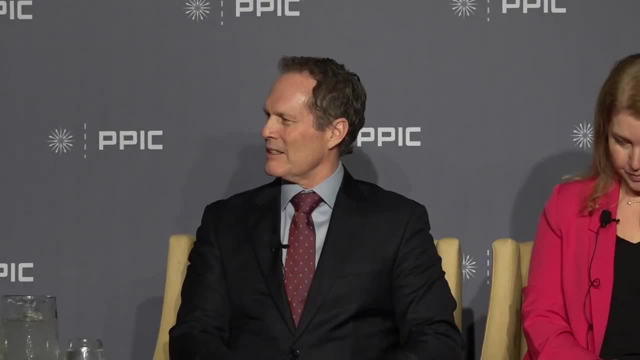 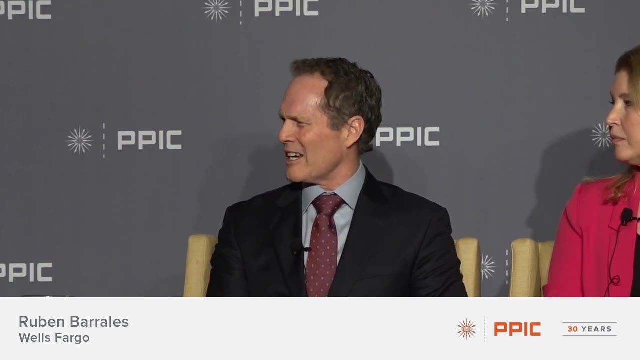 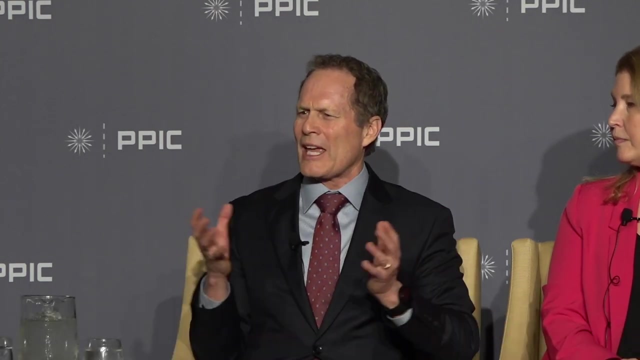 A lot of opportunity and a lot of challenges. It is as dire as some say the California economy is. it's the largest state economy in the country. I mean it's a driving force, And so it's such a large market you can't ignore it. 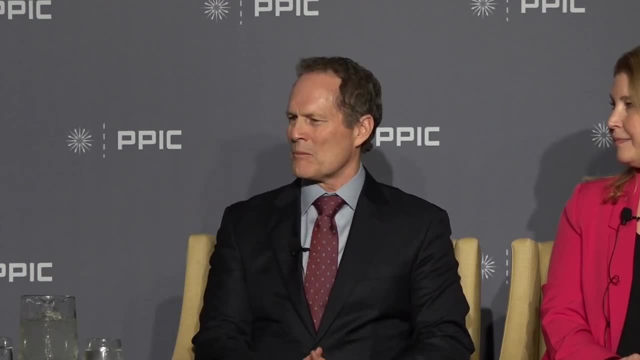 And business has to be here, small and large. So it's an incredible opportunity in terms of a large market And I'm sure we'll go through the challenges. but the top on my list is housing affordability or lack of it. Okay, Cindy. 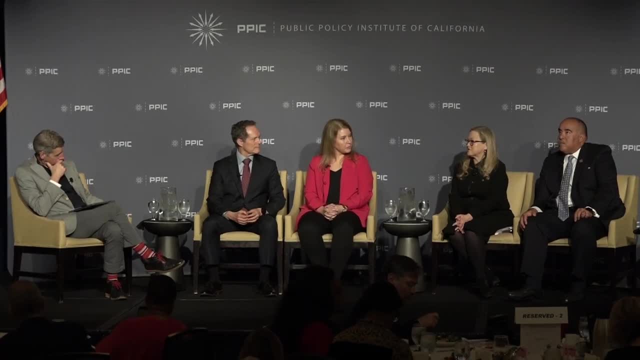 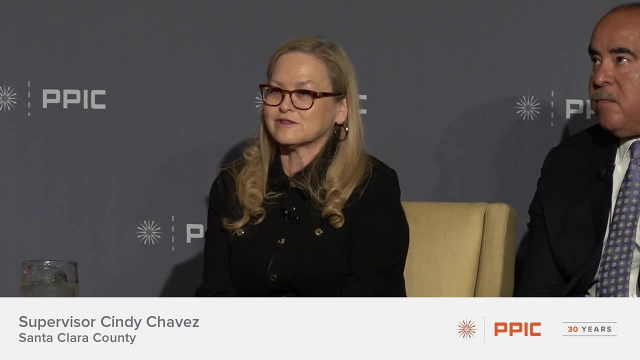 I would say for low-income families. it's a treacherous time And in the community that I represent, I'm in the heart of Silicon Valley and I represent some of the poorest people in the state And we're looking at a place where we have a third of the people in Silicon Valley own their homes. That used to be two-thirds. We only have, of that population, only 13% of the Latino population and 9% of the African-American population own their homes, And Santa Clara County is about 40% Asian. 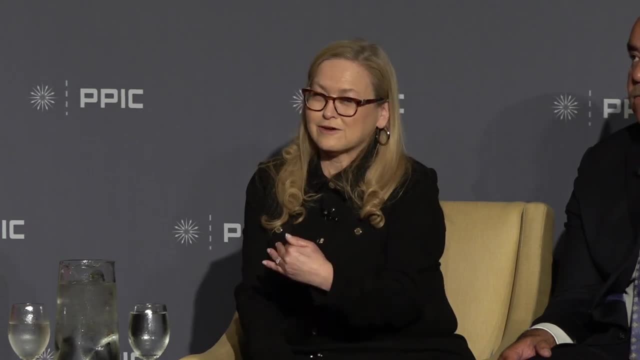 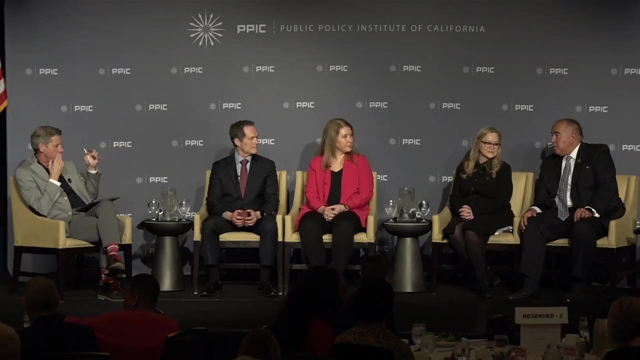 30% Latino and about 25% white, And so what I would say is that we have a lot of work to do. Paul Bifurcated. It's like today, You know, it's Valentine's Day. 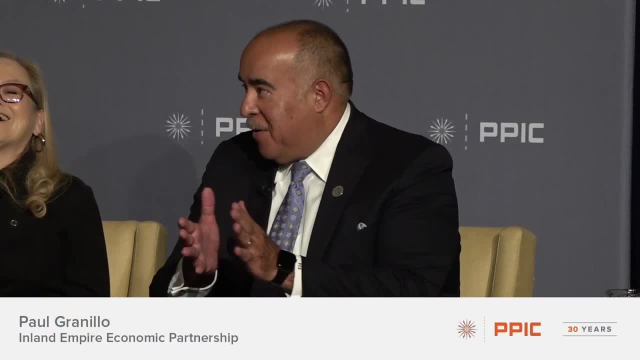 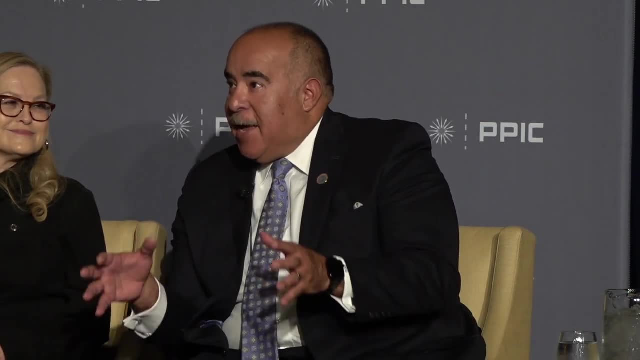 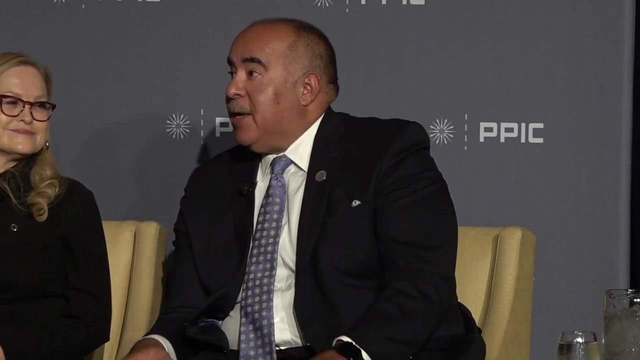 and it's Ash Wednesday, right Bifurcated. And so when I look at the Inland Empire, I have to look at a very, very young region, a growing region and a region that's very vibrant, but the economy is bifurcated. 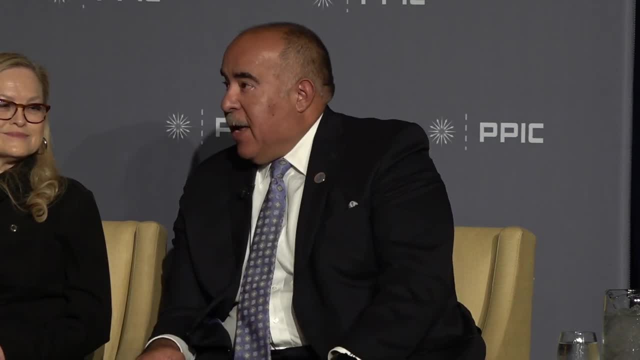 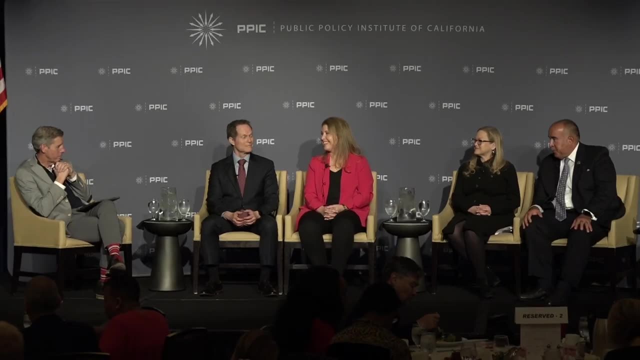 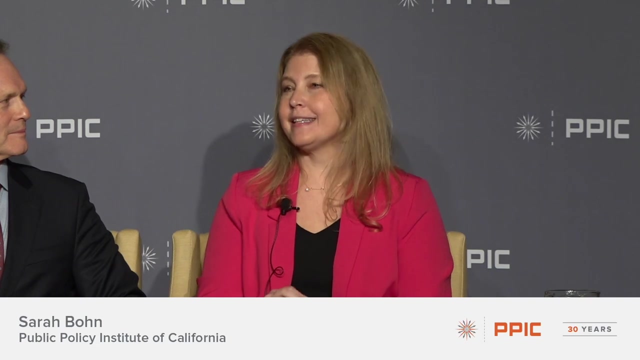 And the opportunities that we have aren't what they need to be, And so that's the word that sticks out for me. All right, economist, Go ahead, I will. The word resilient comes to mind. We've actually been surprisingly resilient in recovery. 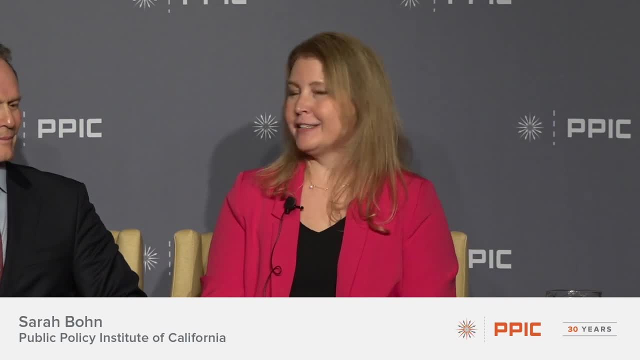 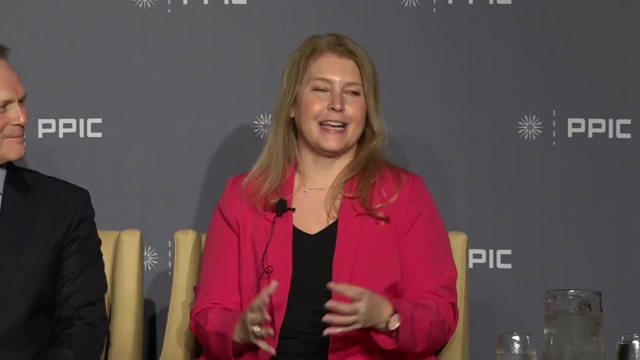 and the macro indicators are surprisingly good. in ways that you know, everybody became a dismal economist, I feel like, or a dismal scientist, over the past couple of years and prognosticating about a recession, but we're not seeing that yet. 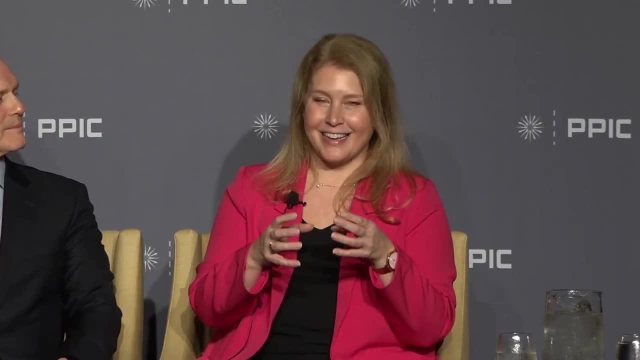 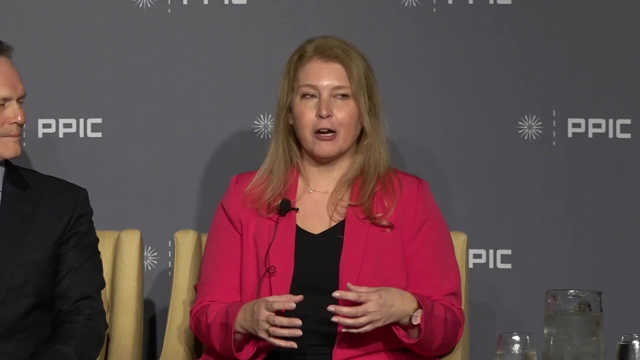 That's a sign of resilience, But real resilience would be that if it feels resilient to each family in California- and that's to echo Paul, where we see a lot of disparity and difference in access to opportunity, So resilient on the whole. 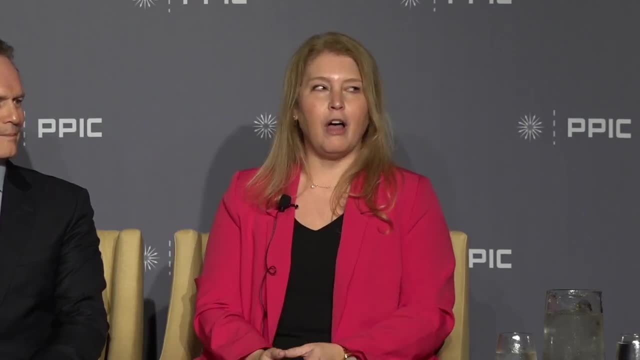 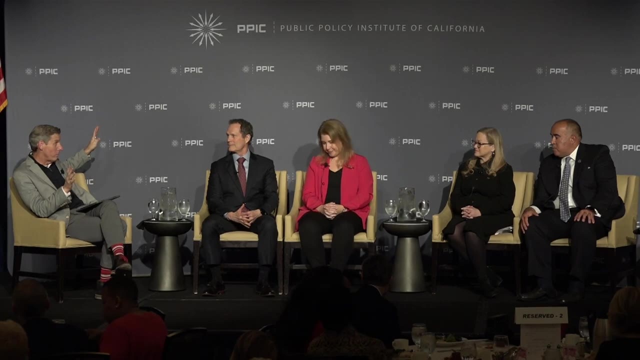 which is a good place to start from, but with a lot of, with a lot of challenges at the family level, Not unlike, we should say, the national economy right, Which is doing well on the macro level. You read the headlines. 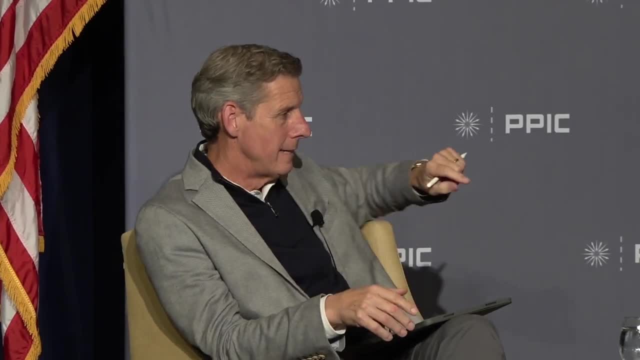 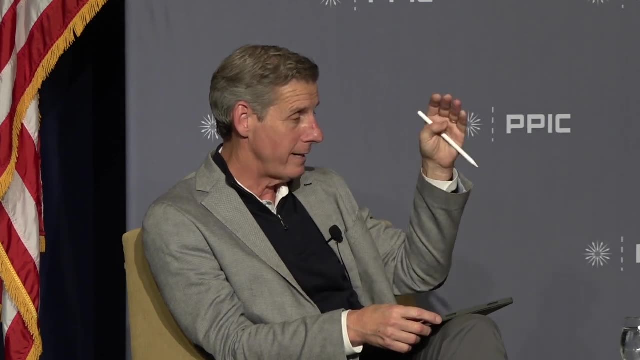 but then you get in there and you talk to actual people and they're not feeling so great. Let me stay with you, Sarah, for a second and ask you about the changes we are seeing and have seen right In all of the 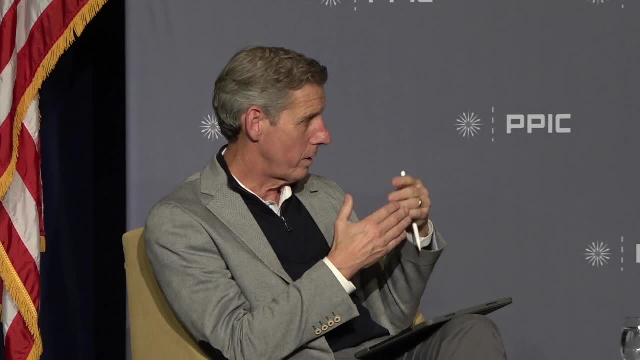 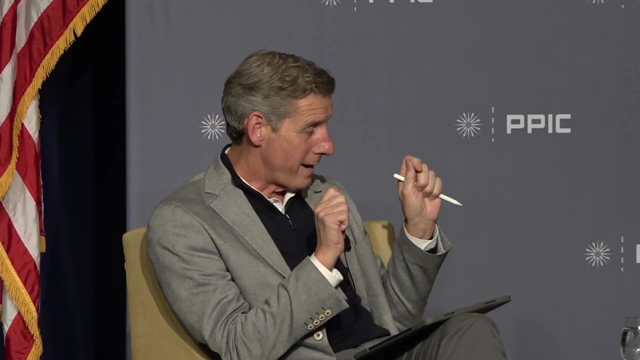 And I'm sure you've got them at your tables right- The booklet on the introduction of the Economic Policy Center, which, for the record, is a fabulous idea. You talk about how California has been resilient for decades and generations. Here's my question, though. 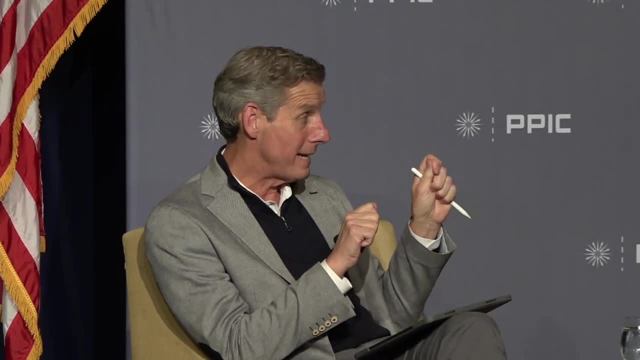 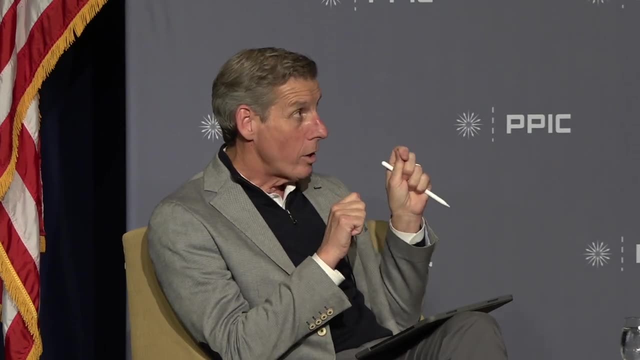 It is different this time. It is different now. right, The pandemic has changed things: the wealth, inequality, the bifurcation, the treacherousness, the direness of it. Are you confident that we can be resilient again, Not to keep going on the downer? 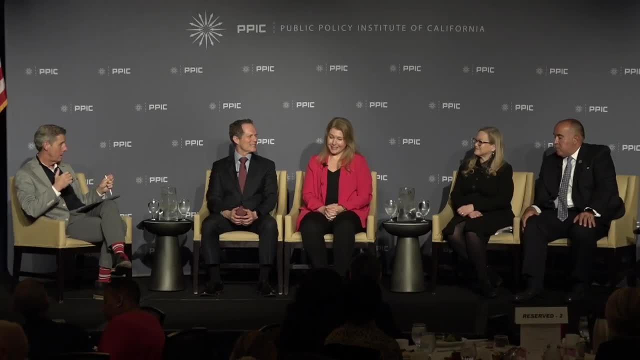 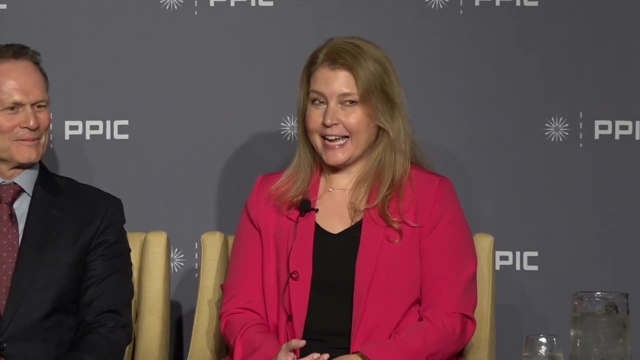 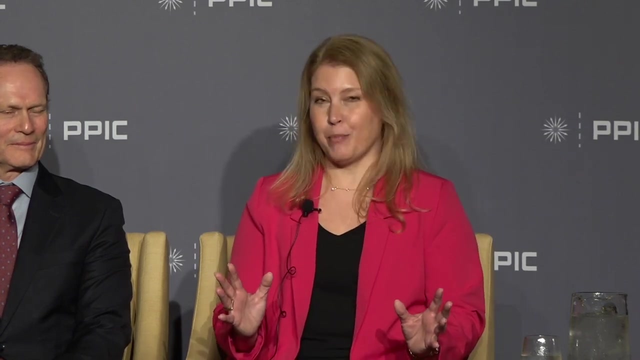 but you know what I mean, right? Well, I am an optimist, even though I'm an economist. so I do see a lot of strengths. We have had decades of of strong economic growth, innovation, wealth creation. you know, innovation that goes well beyond our borders. 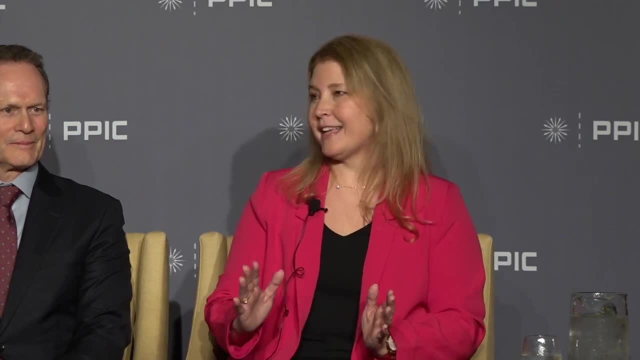 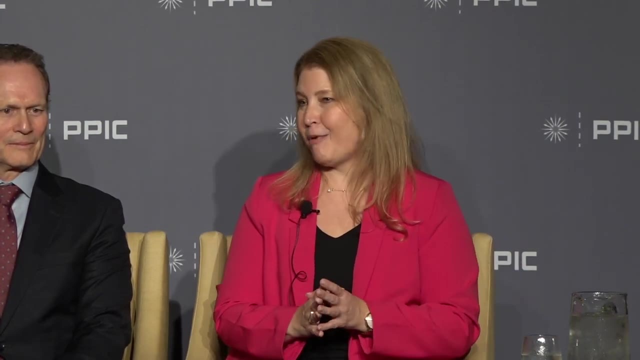 from California, coexisting with increasing inequality, where you know the structural, you know nature of opportunity in the labor market has bifurcated, as Paul described. Those things can coexist but they don't have to coexist. 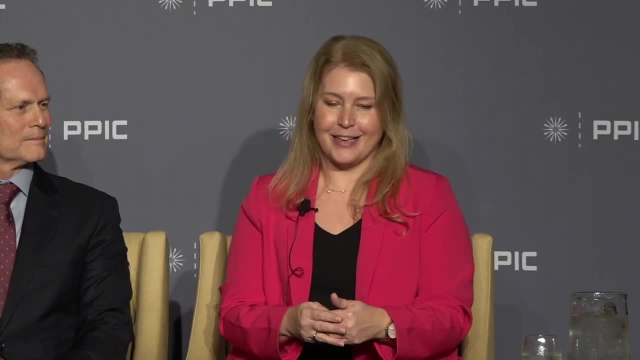 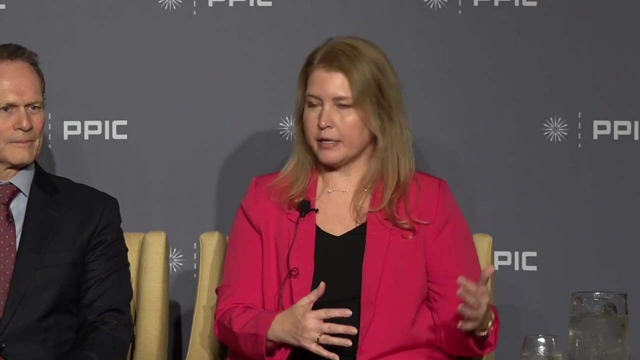 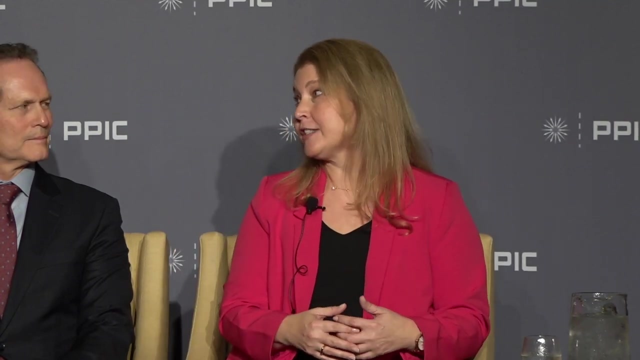 so I think we're on the cusp of, you know, those major transformations that the video talked about, On top of those long-term, persistent challenges that we have: cost of living, access to good work and upward mobility, along with those new challenges on the horizons. 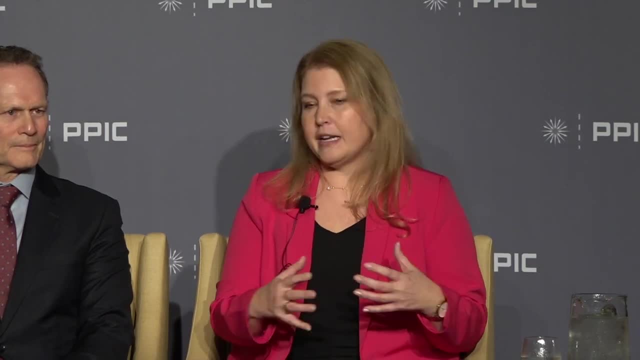 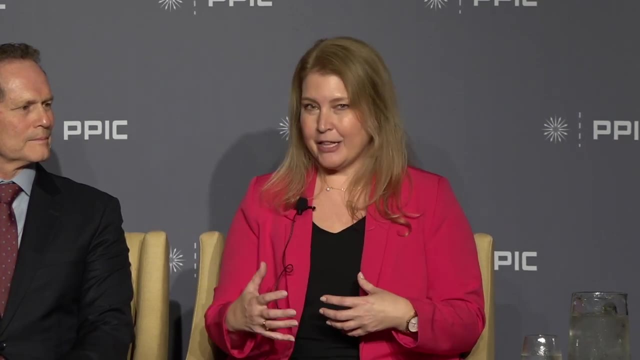 But I'm optimistic because the solutions, that kind of address both which get to the barriers that people face to building a business, to advancing through their work, to building their skills, are the same kind of things that we need for those future opportunities to be more kind of widely shared. 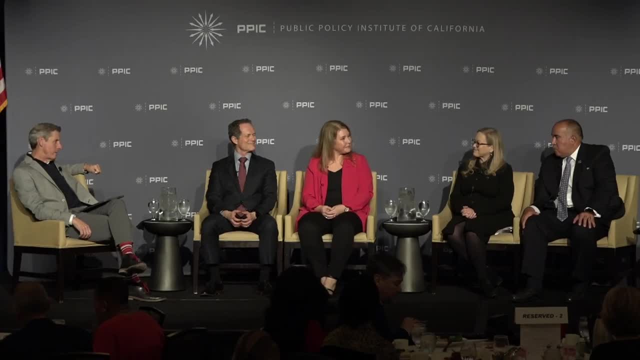 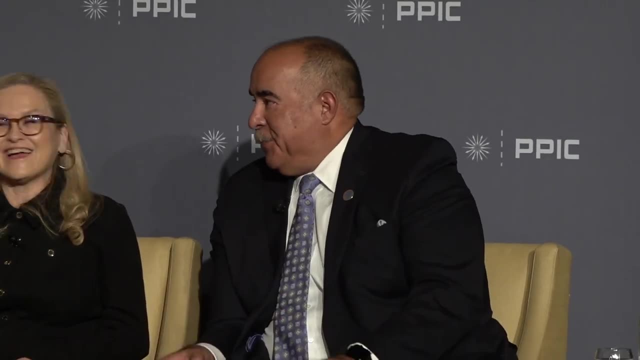 Paul, take me now to the Inland Empire. Take me now to Riverside and San Bernardino. You go out and you talk to people. What do they say? So, to use your line, let's do the numbers, All right. So most of you probably don't know. 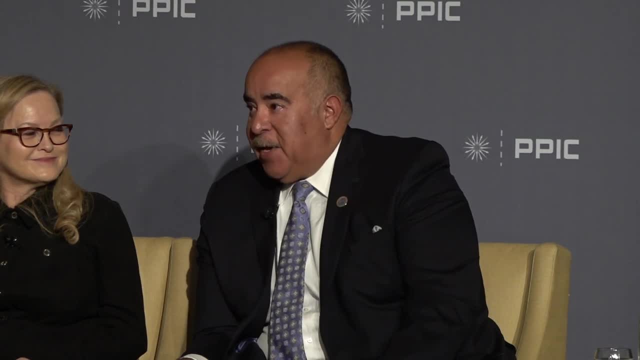 that the Inland Empire is the 12th largest MSA out of 390.. Metropolitan Statistical Area: Correct: We are larger than the Bay Area. and next on the list is Boston: 4.6 million people, Half of them are Latino. 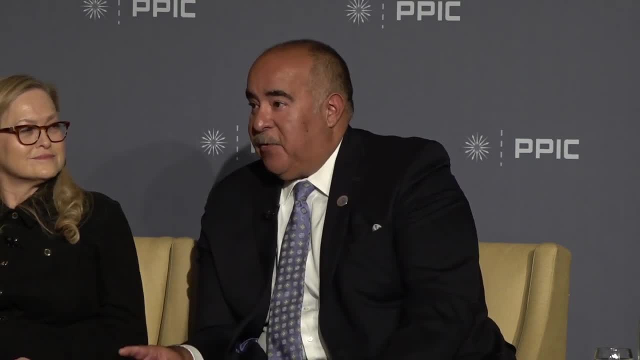 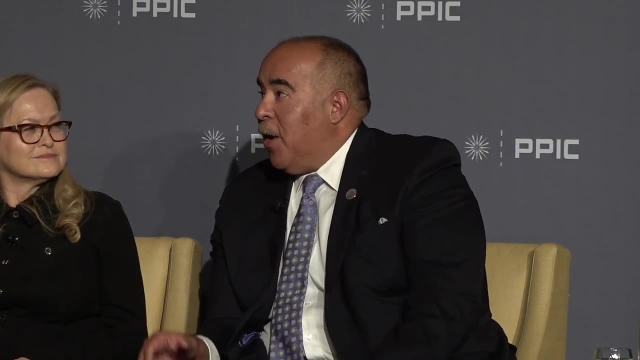 Okay, But of regions of over a million people, we have the lowest baccalaureate attainment in the nation. So when you talk to people, the question is: where is the future? So I talked about a very young population, the Latino population. 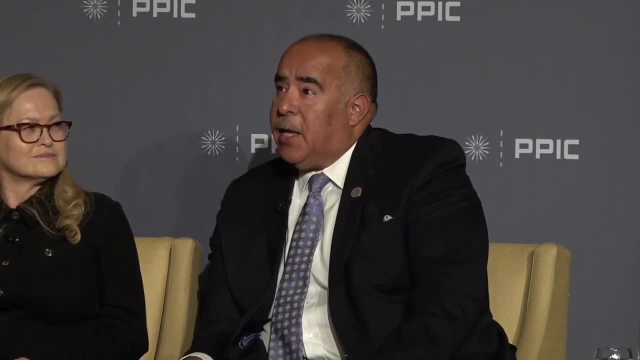 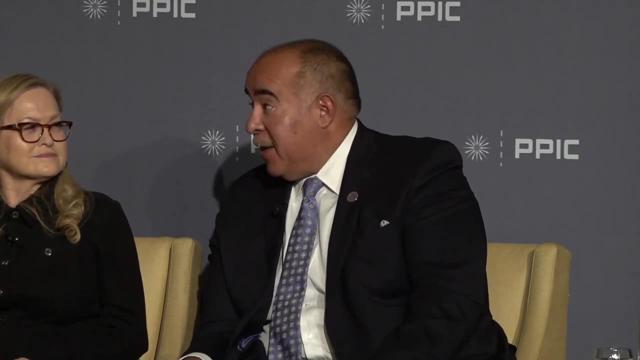 on average is about 17,. right, So the issue is: our best and brightest don't have opportunities when it comes to the tech sector, Many of the sectors that just are part of the equation in Los Angeles and San Francisco, Silicon Valley. So we lose our best. We lose our best. You know, my wife works at the UCR Medical School and that medical school was created for us to keep our own and have them be doctors and nurses in our area. yet we're competing against. 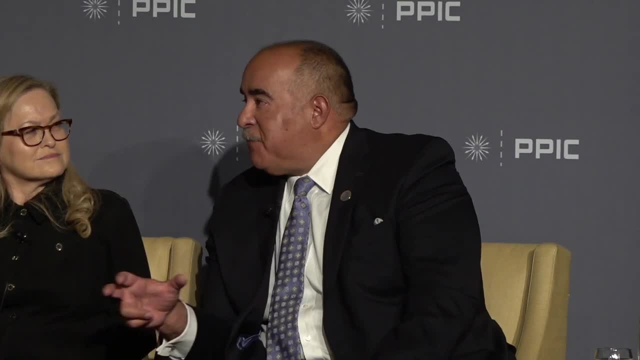 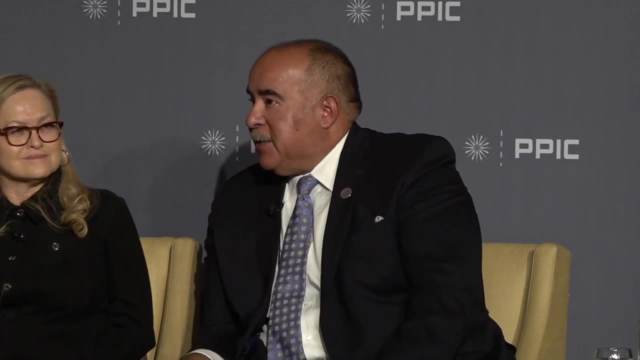 you know, hundreds of thousands of dollars of scholarship money that sucks out our best, And so what we're looking for is the opportunity to have some type of parity. That's what's important for us. So they leave in search of economic mobility. 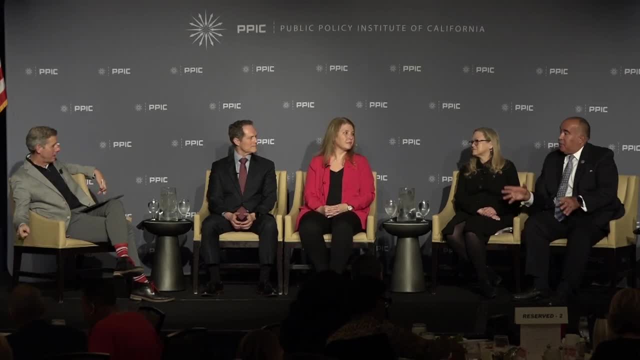 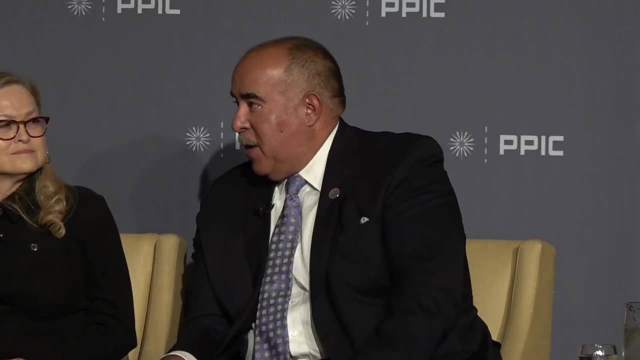 Do they come back Sometimes. but let's talk about doctors. Where you do, your residency is where you're going to stay, And that's one of the issues that we have Right right, Dr Isaac and I were speaking earlier about the Inland Empire. 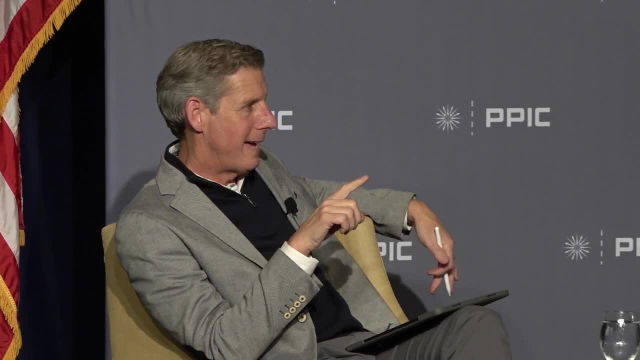 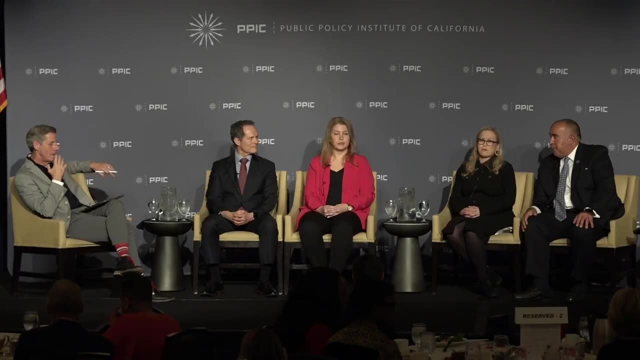 Basically as many people- more people than Alabama, basically, but as poor as Alabama, something like that. So it's tough down there. Yeah, in places, in places. Ruben, as you sit around, you know not the boardroom at Wells Fargo. 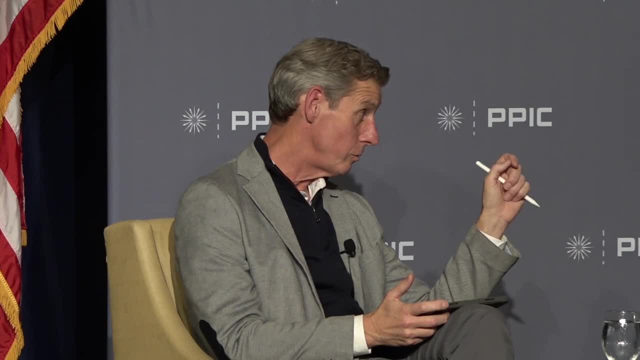 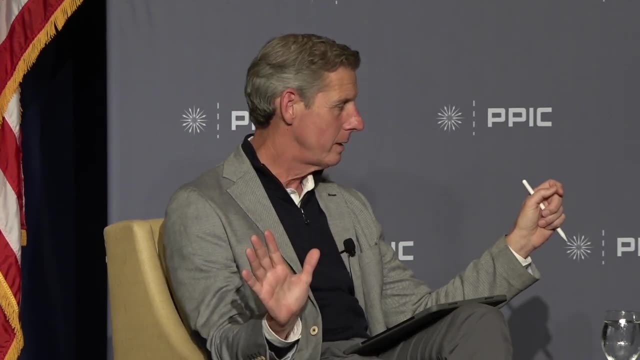 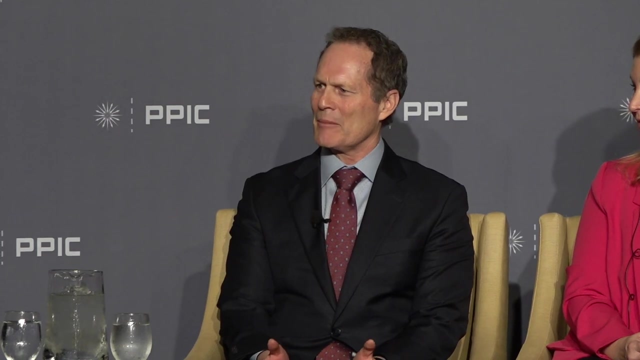 but as you're out talking to your clients and talking to the people that you do all that external affairs work with, what is their- I apologize, vibe. on this economy, Vibe, It really depends, Kind of like California is not really an economy. 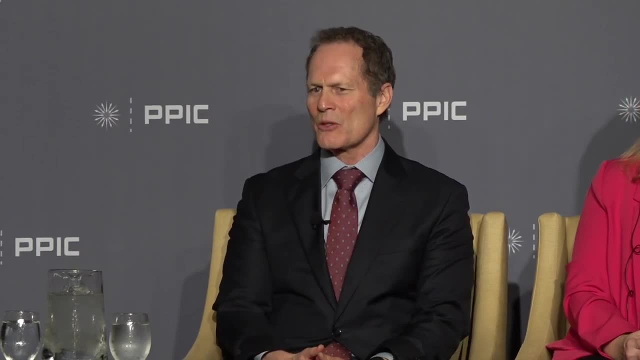 It's a conglomerate of regional economies. I think it really depends on who you ask. You know there's concern about, you know, tech sector layoffs, but the tech sector is still pretty strong in California- Biomedical as well. So I think for 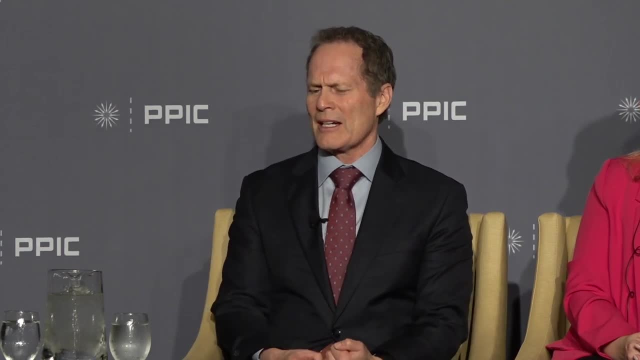 large corporations. you know we're seeing a little bit of uncertainty, so that creates some downward pressure on budgets and talent acquisition and all, And I think for small businesses. it's always been tough to be a small business anywhere but in California. 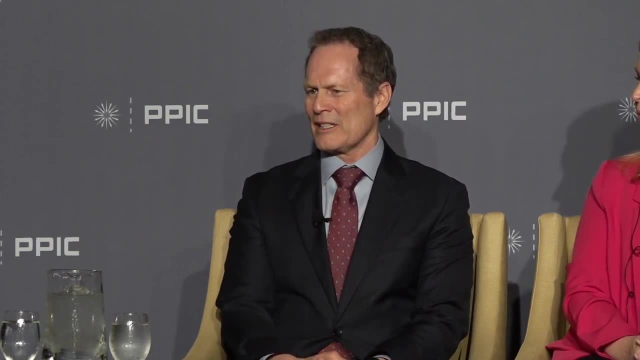 And I think that uncertainty is really making it hard for folks to be able to secure capital, interest rates and the like. So it's hard. I just want to say as a UCR alumni: the Inland Empire is a place where people are going. 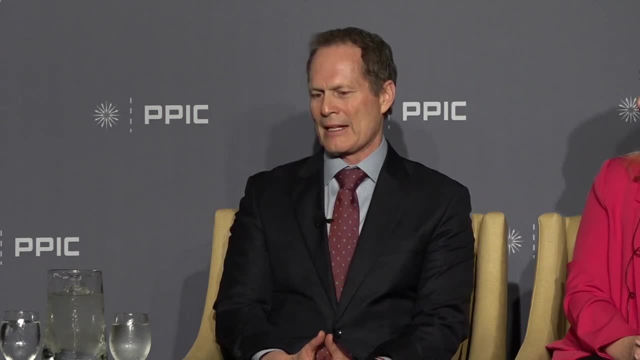 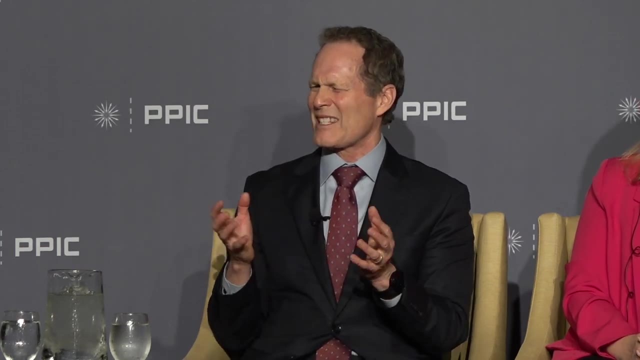 to you know, find affordable housing. And there are other sectors, regions, Central Valley, where people are going to find housing And the kind of working premise had been for decades. Well, if people go there, you get enough of a market there. 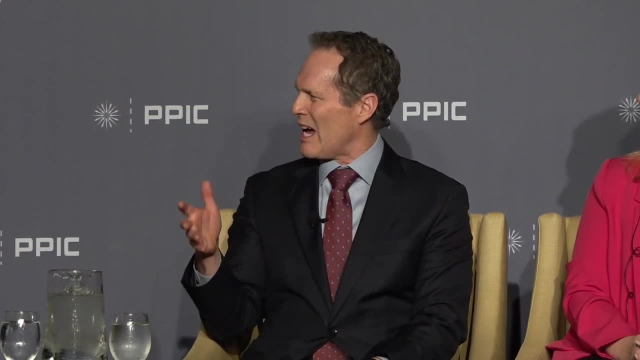 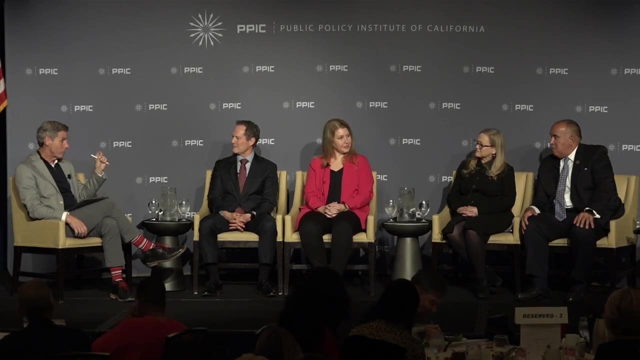 then jobs will be created there, And you're seeing some of that, but maybe not at the pace that we need. Sidney, let's talk about jobs and small businesses and economic development in Santa Clara County And, for those who aren't familiar, 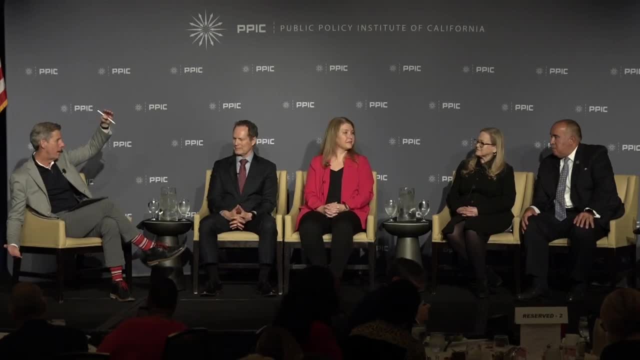 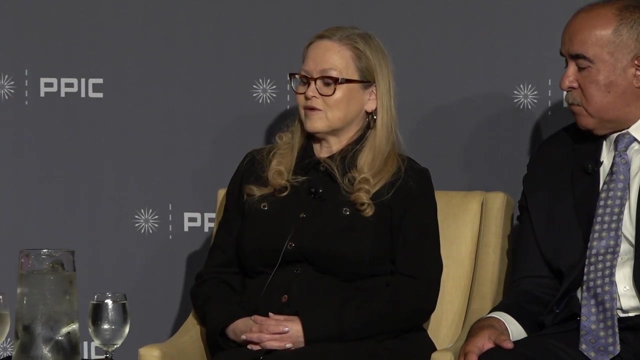 Gilroy, basically up to Stanford, Basically right A broad diversity of incomes, of education, of racial and ethnic makeup. How do you do economic development there? That's an excellent question. I think one thing to remember is that we're very blessed in our region. 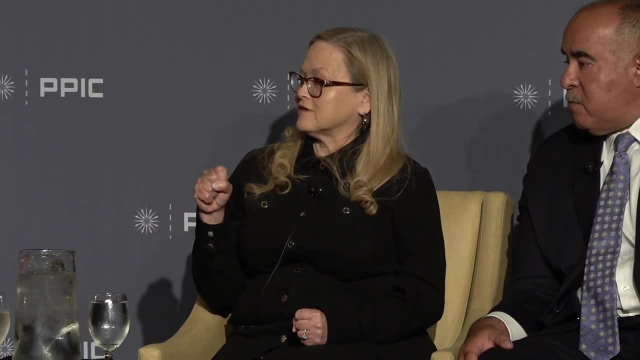 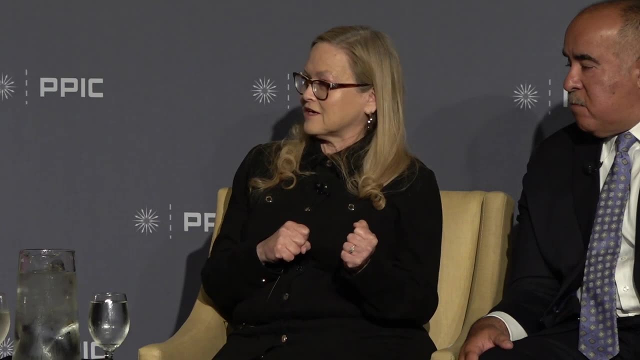 to have great community colleges: Stanford, Berkeley, San Jose State University. By the way, San Jose State University produces more engineers than any other school, And so when you look at Silicon Valley, what you're really seeing is Spartans everywhere, And I'm not 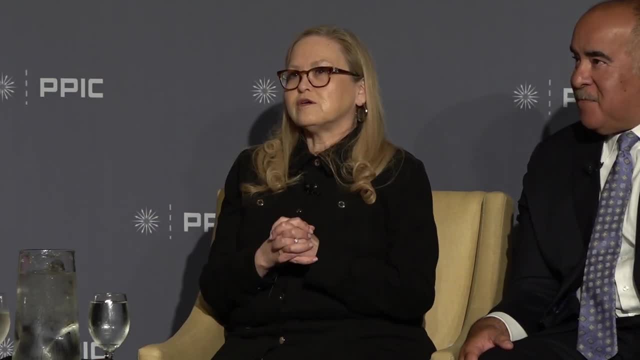 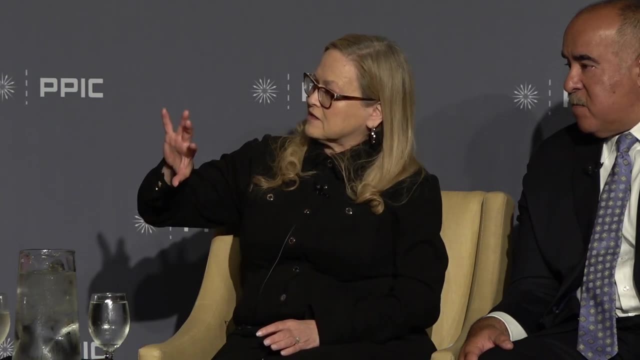 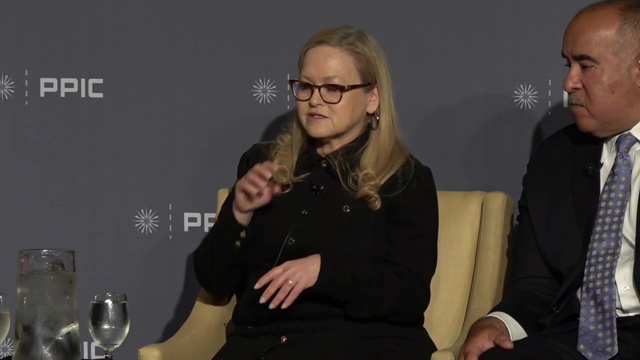 just saying that because I'm a Spartan. But what you see is this incredible, and I will use your term about the bifurcation between the tech jobs and the tech community, and then the lower income jobs, And I'll just give you one statistic that may be of interest. So, Santa Clara. 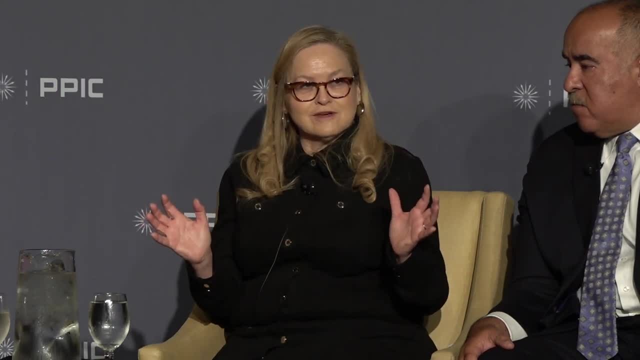 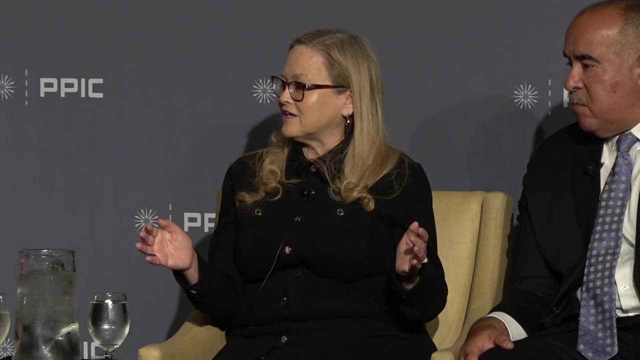 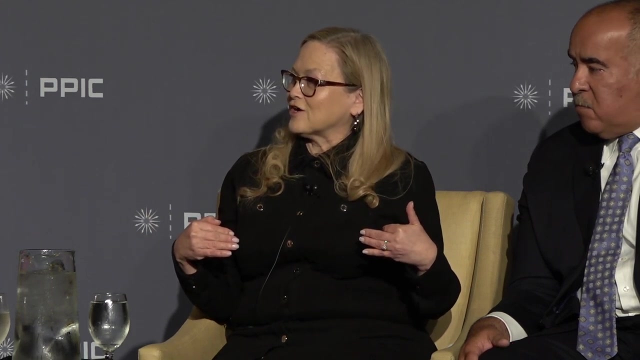 County is a really odd place in many respects in terms of its demographics, But one of the demographics is that 40% of all of the people who live in the county are foreign born. 67% of all of the folks that are in the tech industry are immigrants. 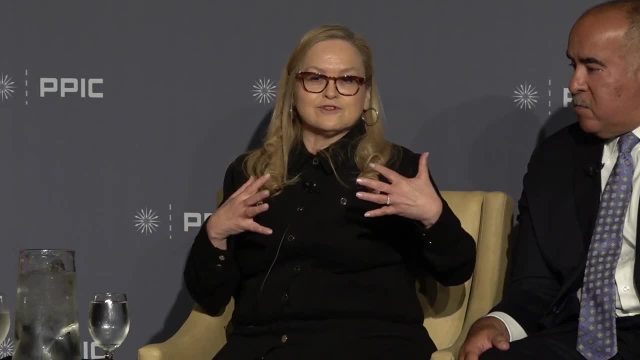 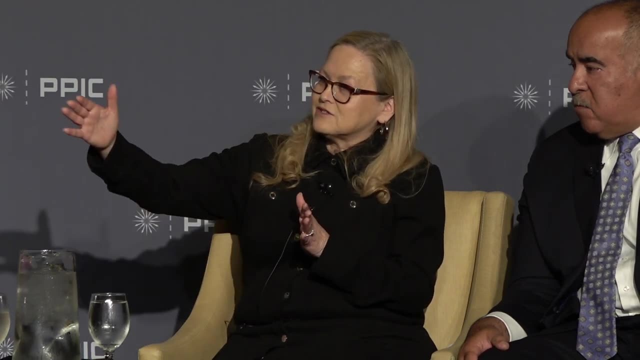 So what that means is that, to your point, we have children growing up in the east side of San Jose who don't have the social mobilization that will allow them to get into C-suites and into these other kinds of opportunities, And one of the things I 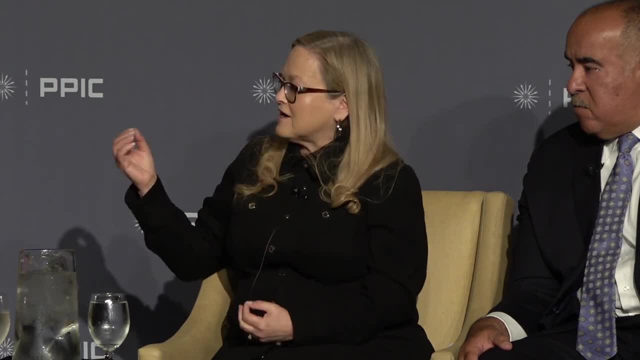 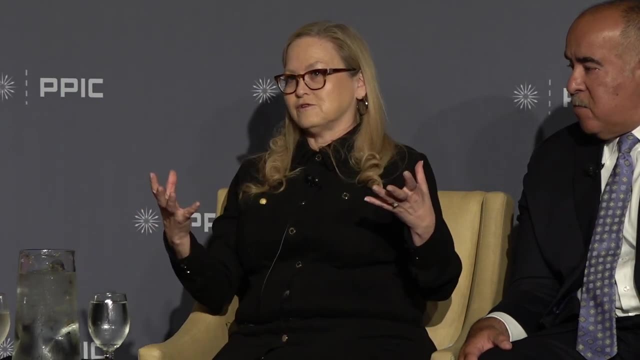 think about, as it relates to California, is that I, in general, am an optimist too, and so I think we don't have an option but to think about how do we make the future better. I will say that I think the state as a whole has. 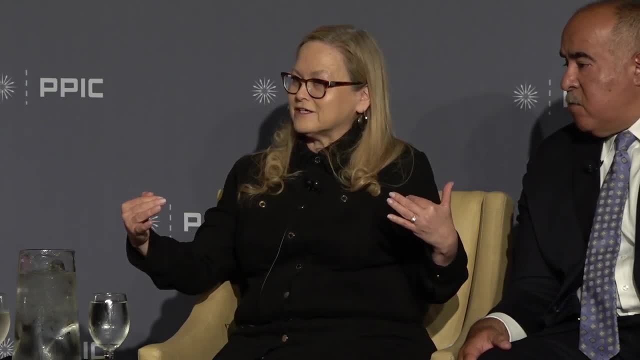 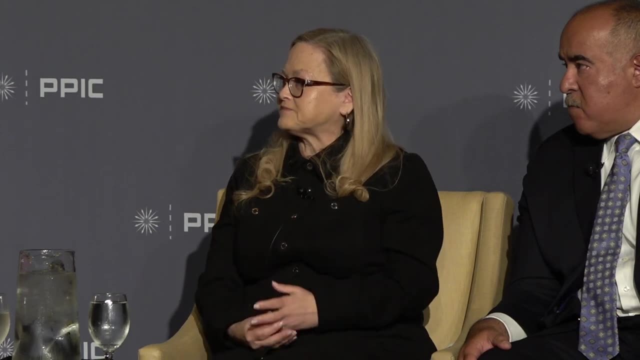 been so incremental in the way we are addressing really pressing issues that I worry that we're going to miss the window of opportunity for change. Hold that thought, oh, politician, on the panel, because we're going to get there. Sorry, I'm marking this in red. 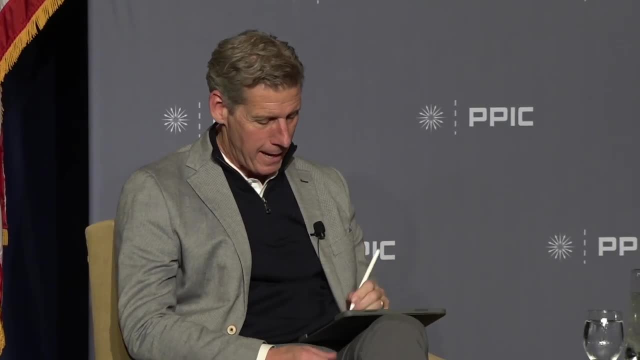 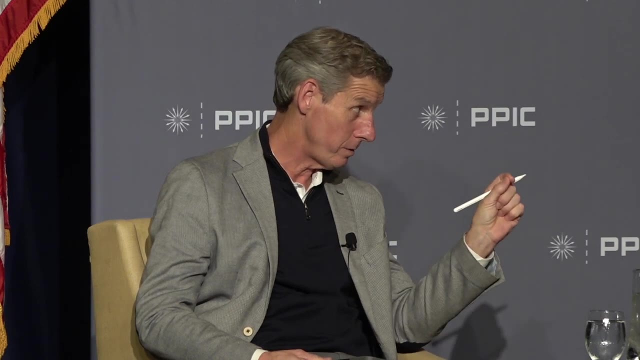 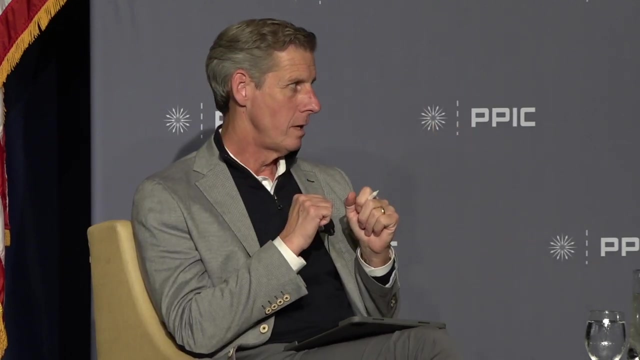 You bought yourself that question, Sarah. though let me take the workforce thing, the economic mobility thing. I will point out that you're a labor economist. right, Let's talk about the labor force in this state, in a time when immigration is being throttled. 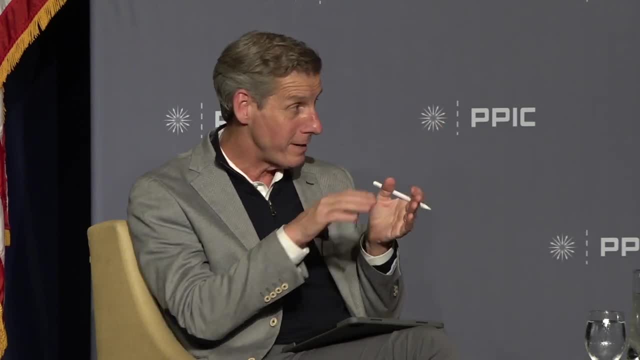 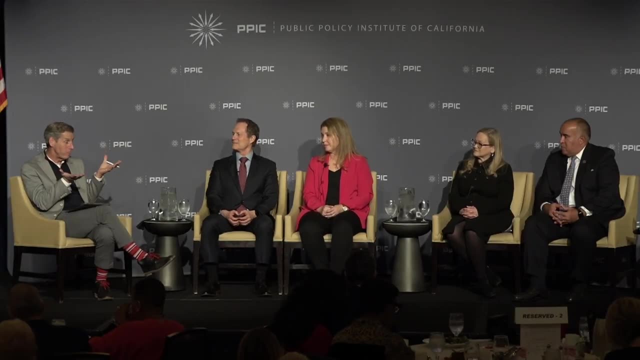 migration is changing. people are leaving the state of California. labor force participation rate in this state is down. What are we supposed to do about growing an economy and raising all boats if the people ain't there? The economy is people. It is the structure. 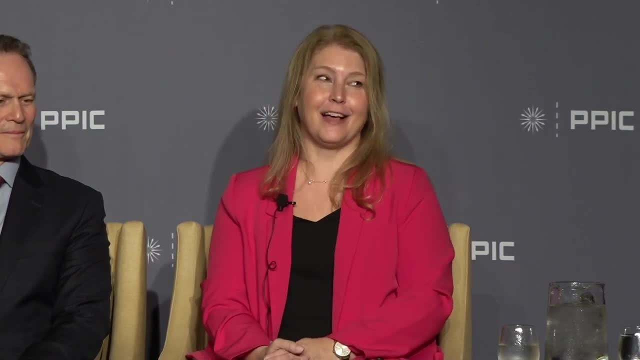 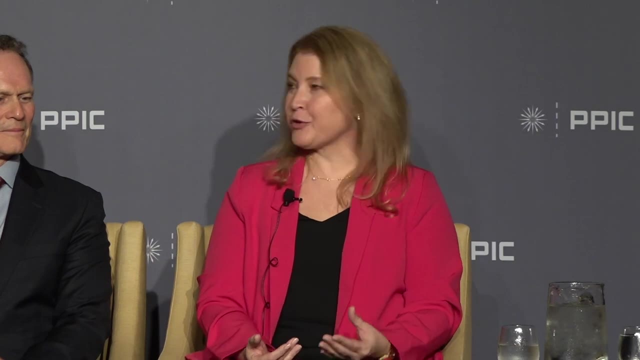 that we built, that organizes us, that coordinates us, that helps us all make our ends meet. If we don't have people, we don't really have an economy. It's not easy to have economic growth when you have shrinking population, Unless, maybe, robots. 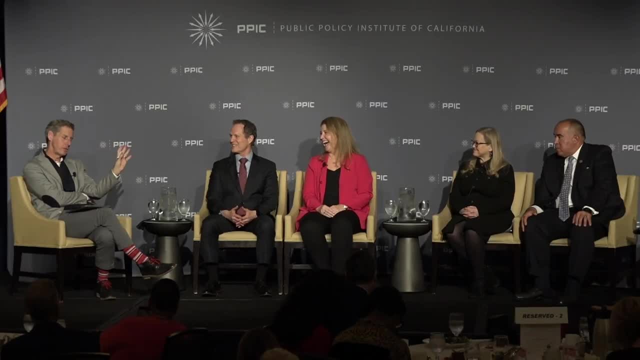 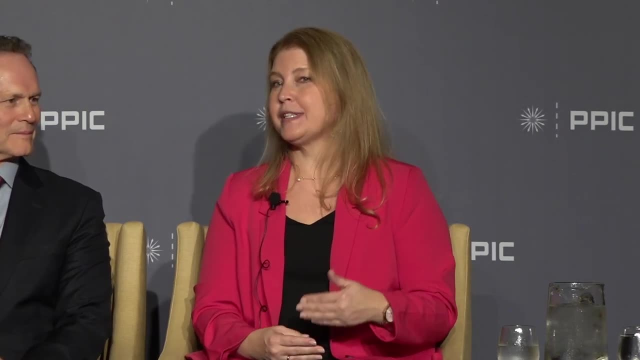 or technology can We can get there too. right, We're going to get to AI. Hold on. We have a big challenge ahead of us because we have an aging population, although California's workforce is younger than the rest of the US. 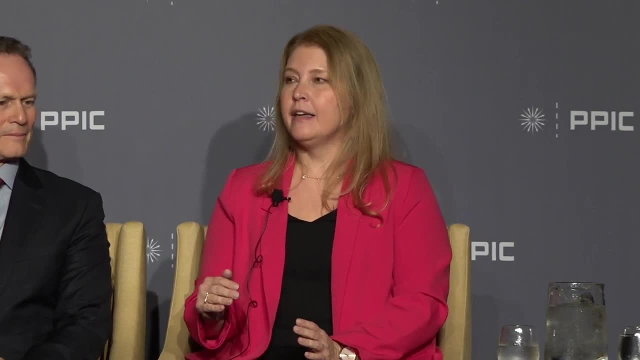 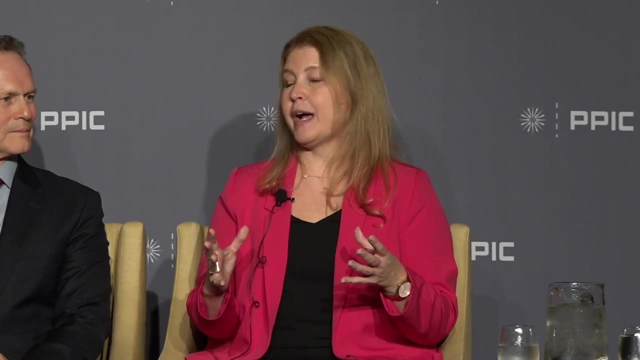 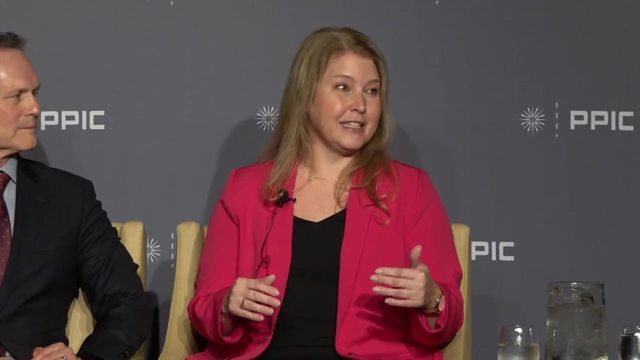 That's a plus. Nonetheless, it's still aging rapidly. We have a smaller and smaller workforce relative to the population. The pressure that we feel right now- that I would say businesses feel and that we see in the data- to the challenge of hiring is real and 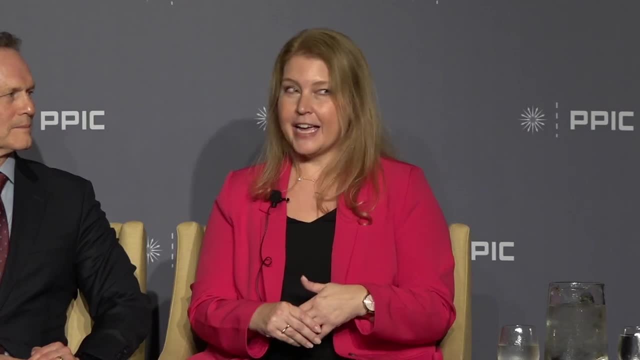 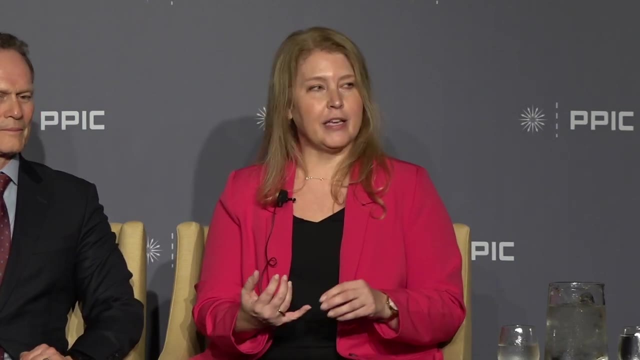 likely to be with us for a long time because of that. On the other hand, we have long-term challenges, barriers that individuals face to participating in the labor market, to having the skills that open up opportunities for them, to connecting with the right kind of jobs. 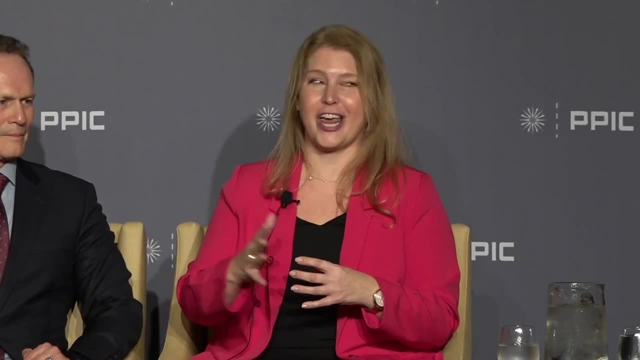 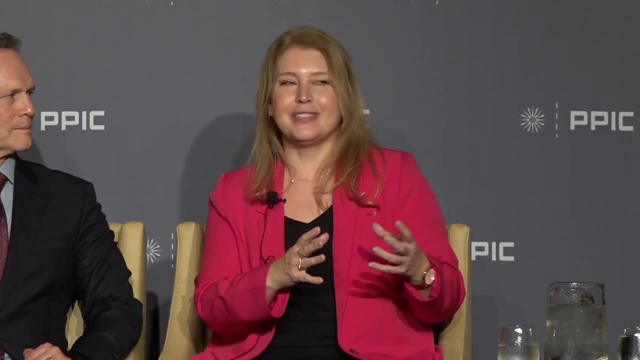 That's going to continue to be a pressure, I think, as things change needs change in our economy, going forward By addressing some of those barriers, whether it's on the skills side or say it's on the household side, the access to child care. 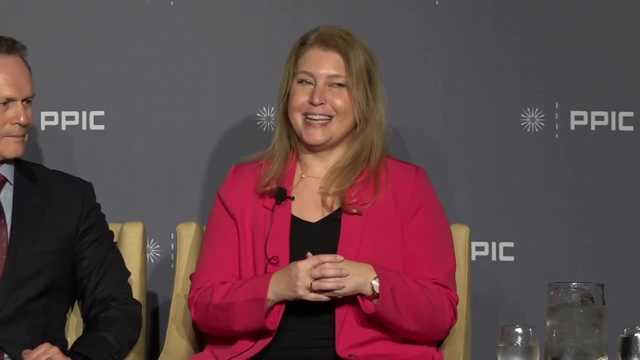 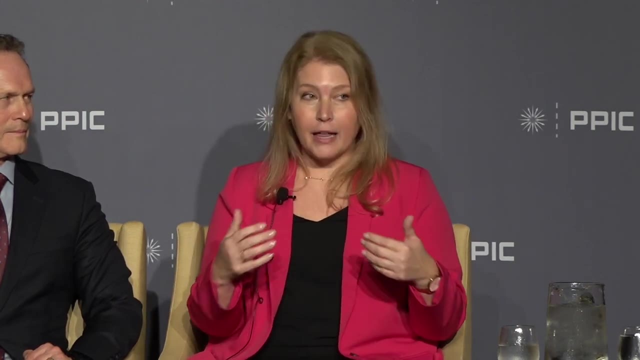 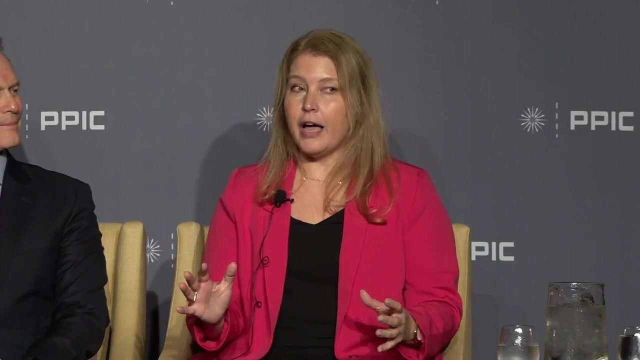 or elder care that allows you to meet your family needs while also maintaining a job. there are lots of levers there that can maximize the participation of all Californians. That's kind of about who in the state currently can meet those needs. I think there's a lot. 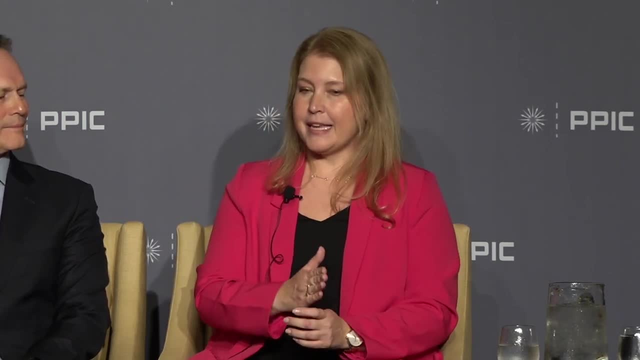 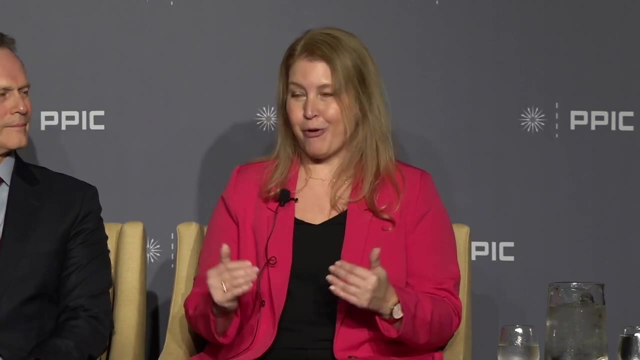 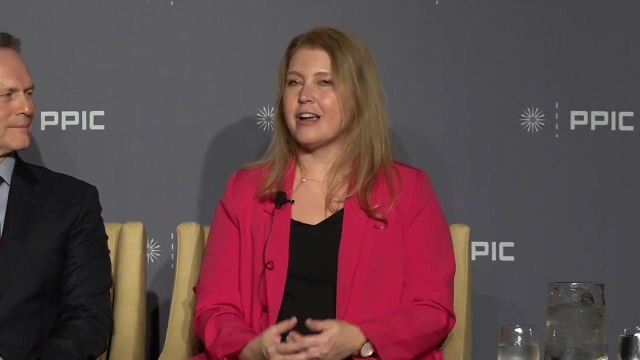 that we can and should be doing on those fronts, I would say over the long term. actually, California has lost people to other states for decades. It's immigration that has grown our population. That external force factor is going to be really important to see how it plays out. 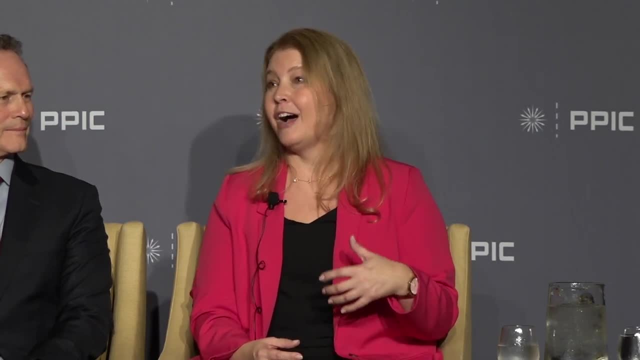 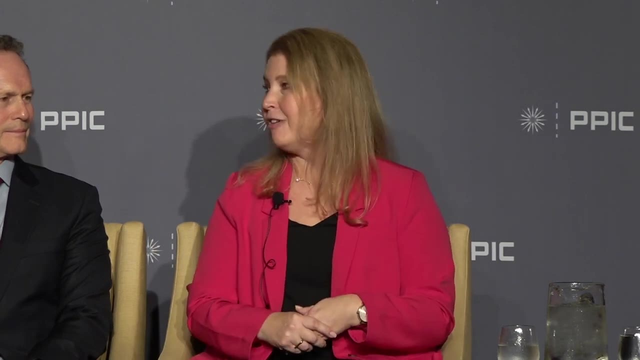 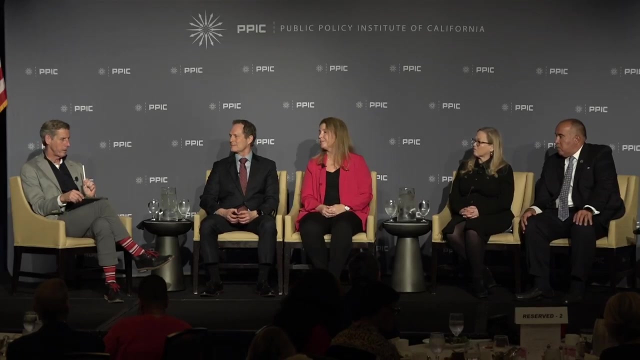 What are the kind of things that will continue to make the state a draw for people that have the mix of jobs, living options, housing costs being more reasonable to draw people, especially from abroad, but potentially from other states as well? Just keep going on that for two seconds. 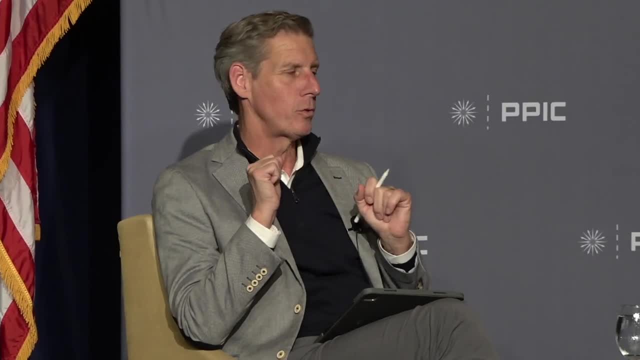 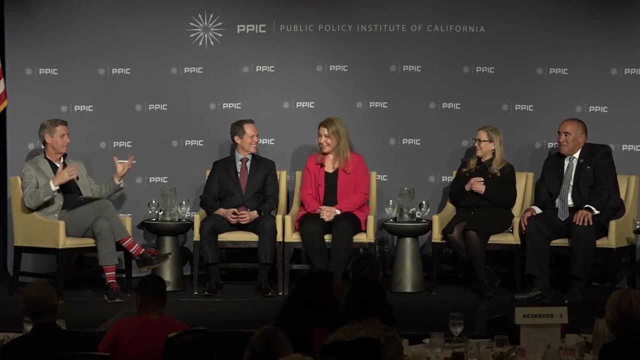 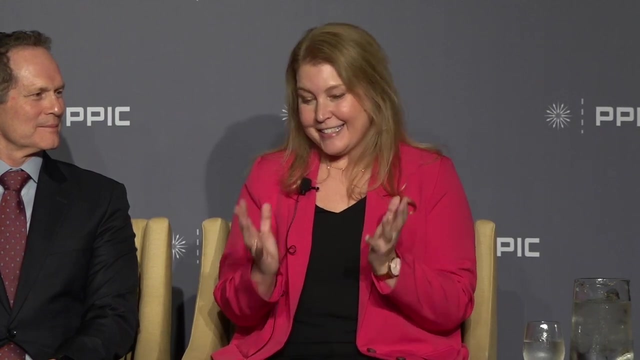 I don't want to get all political about this, but immigration is a labor market story. Discuss. You're the labor economist on the panel. My dissertation was on immigrants in the workforce. I mean it's essential. As I said, people are. 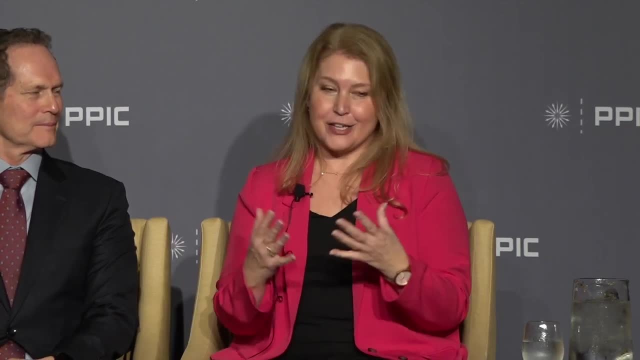 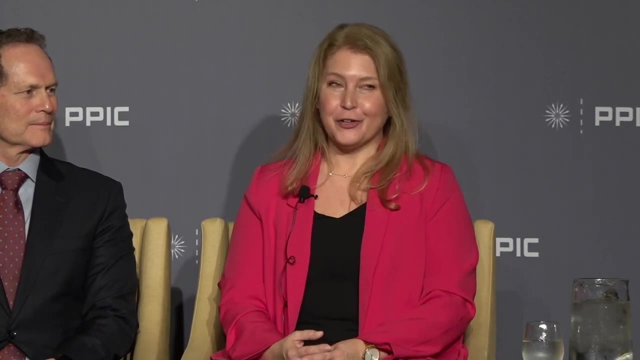 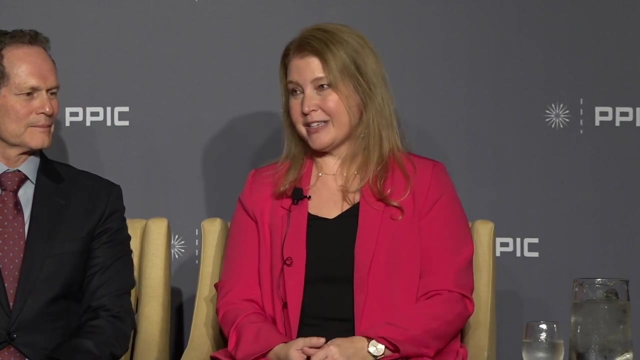 the economy. But there are existential choices that go well beyond California, which we can't control and we wouldn't pretend to. But we can address the things that make the state that kind of golden place to be for immigrants, for people from other states. 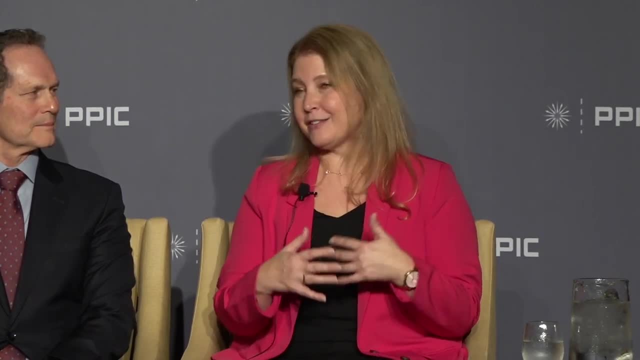 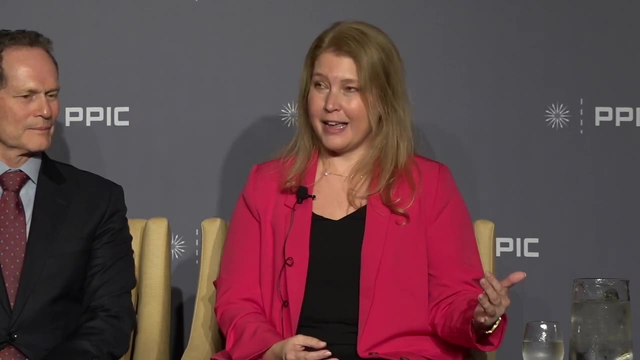 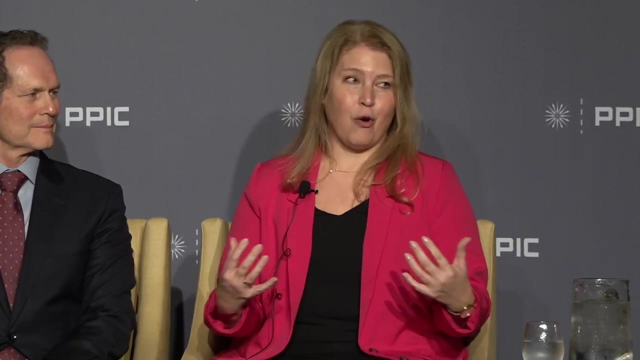 to drive our economy and help us meet our needs. If you look at the care workforce, it is largely women of color and immigrant women of color, And that need there is only going to grow. So we all know how critical that is to quality of life. 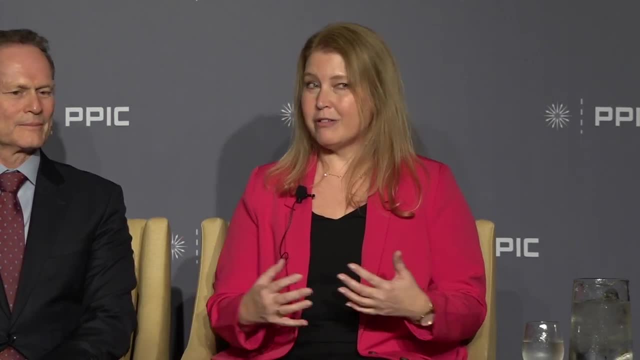 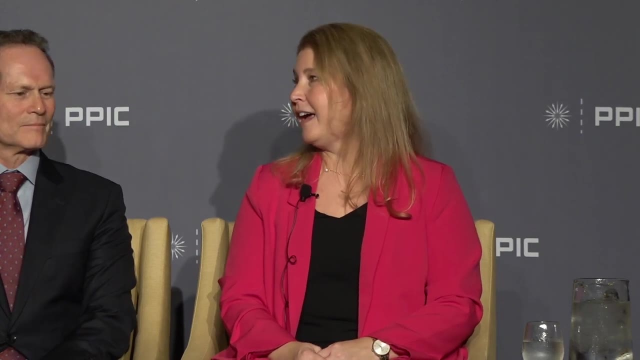 for our families and those we care about to have access to affordable, really high quality care. So that's just one example of where we really can't progress without diversity of workforce. I said I wasn't going to go down the row and ask you all the same question. 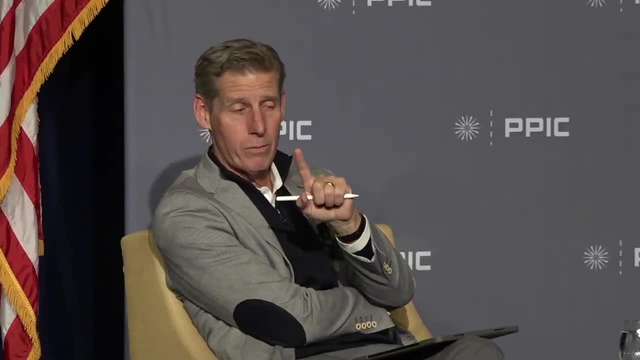 but I am in this one And, just as a reminder, get your questions ready. We're going to go another 15-ish 20 minutes And then the mic runners will come around You. just raise your hands and they'll come to you. 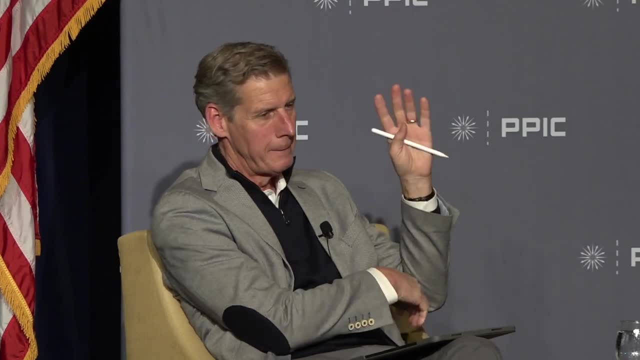 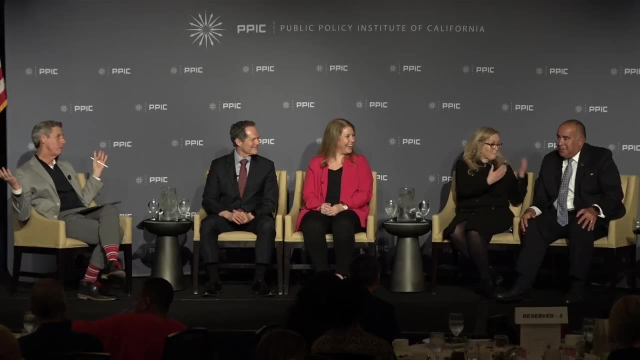 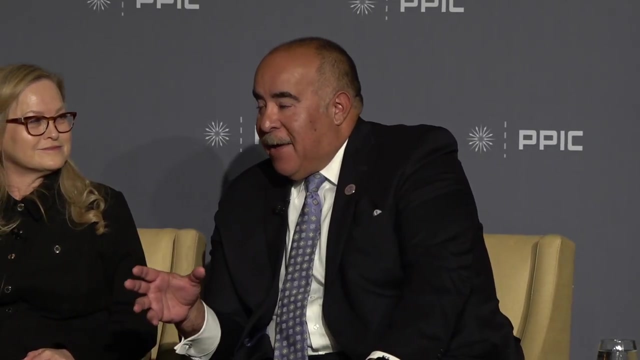 And I spent some time trying to craft the question about cost of living and this and that And finally I just wrote: it's too damn expensive, Paul. What do we do about that? It's too damn expensive. So, three bedroom, two bath house. in Riverside is about $600,000.. You pick it up, you move it across the county line to Claremont and it just gained $400,000.. You pick it up and you move it to Irvine and it gained a million dollars. It's the same. 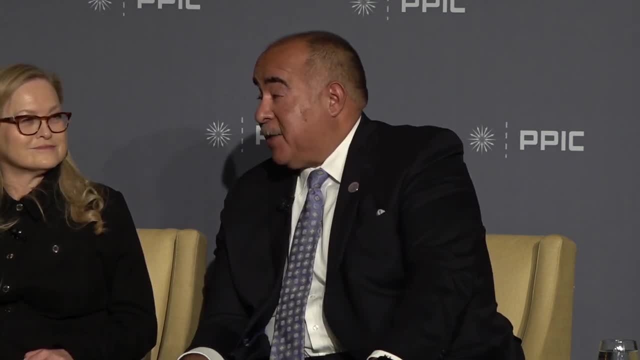 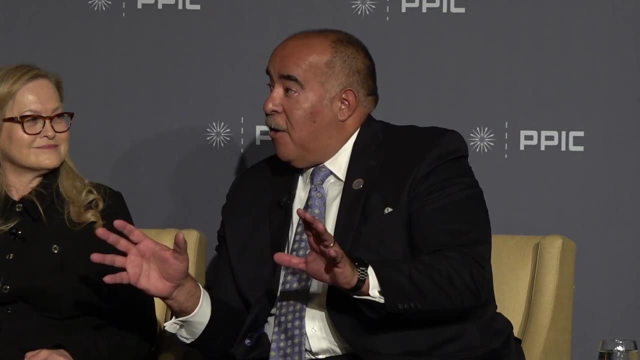 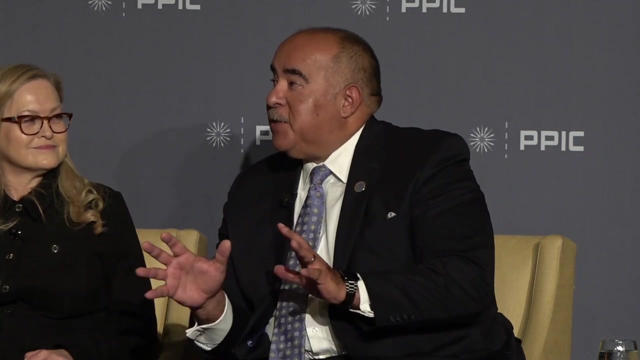 damn house. That has got to change. And California, if we're going to be successful, we've got to align our regulatory with the needs of the employer community, Because what's happening now is a mismatch that is not allowing business to grow in the way. 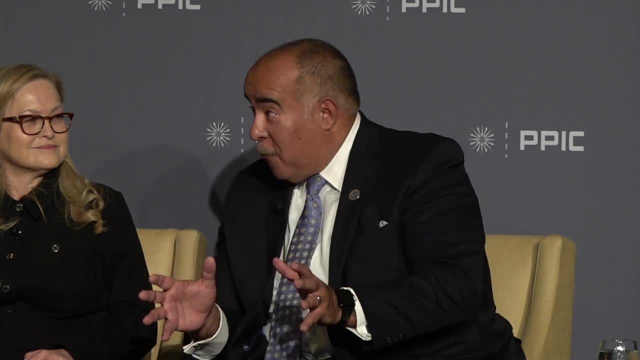 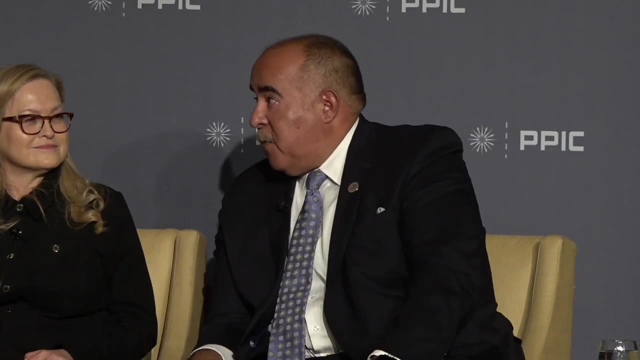 that it needs to grow, Not allowing it to bring in the workforce that it needs in order to be successful, And that, to me, is one of the biggest things that we have to focus on. Cindy, same question. It's not really a question, it's a statement. 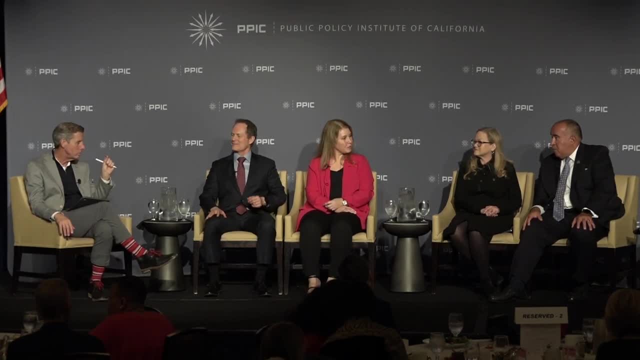 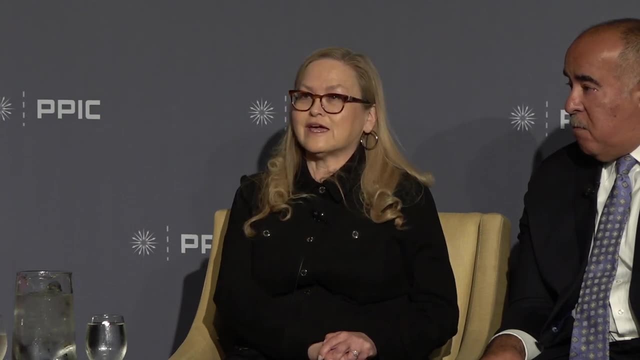 Too damn expensive, But build on his answer and tell me what we do about that. You know I don't actually have an answer to that question, I really don't. And I will say that we- just to go back to the point I raised about 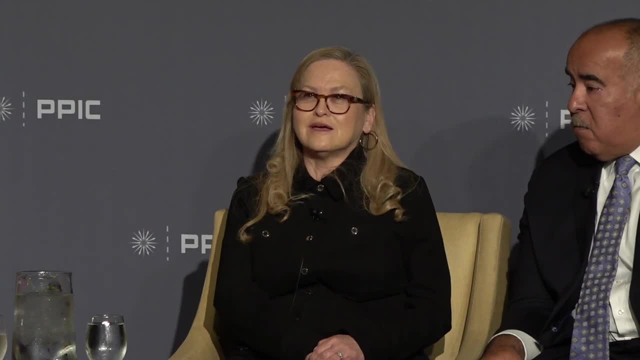 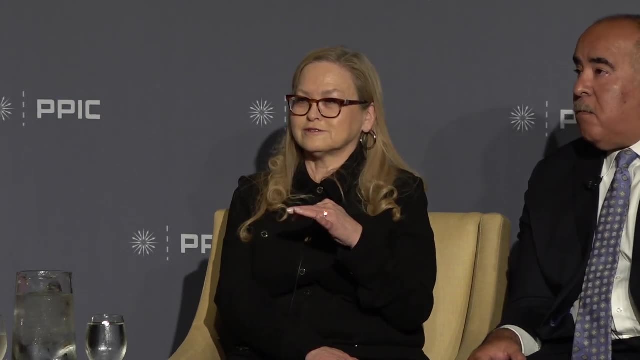 the cost of housing in our community, too, is that over 60% of all the people who live in our community are rent burdened or mortgage burdened- 60%- And what that means is you're spending more than one-third of your income. 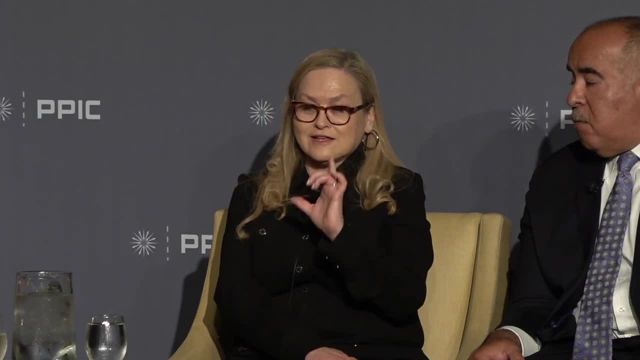 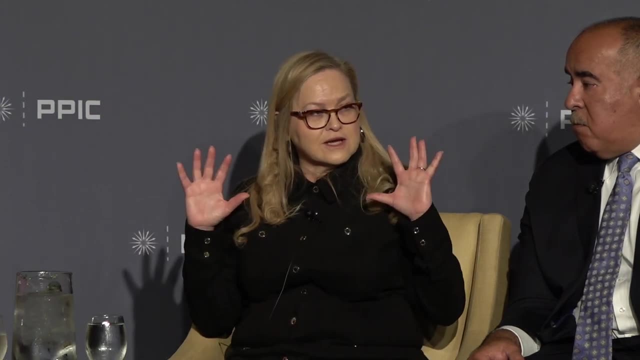 on where you live And that's a problem. And we still have people and I'm going to go to the childcare workers that we're talking about. So in COVID, the state of California lost childcare slots like crazy In Silicon Valley. 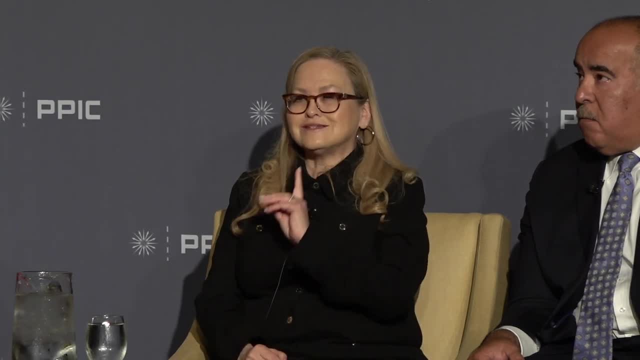 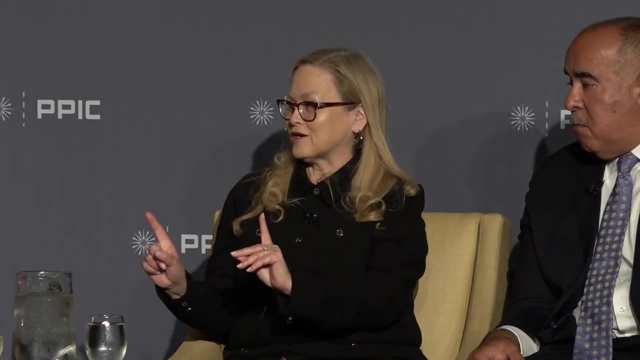 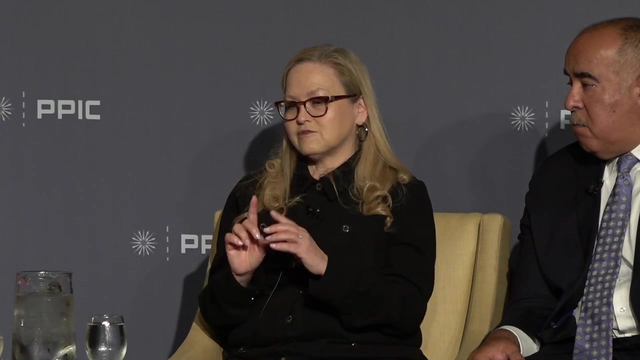 we lost 500 centers And today we only have enough childcare available for one-third of all the parents who need the childcare in order to go back to work. So the reason I was focusing a little bit on not being incremental is that one of the challenges we have is that we want. 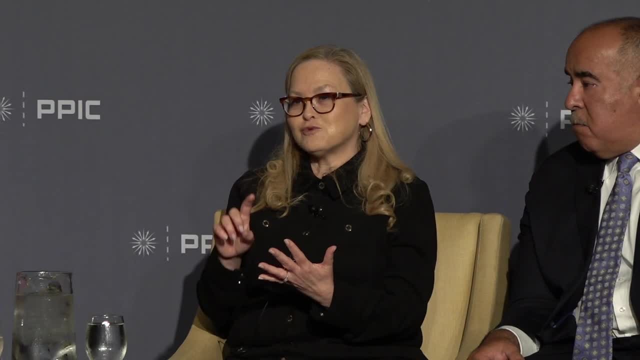 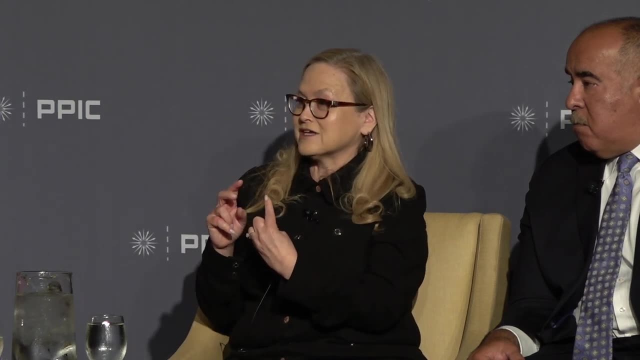 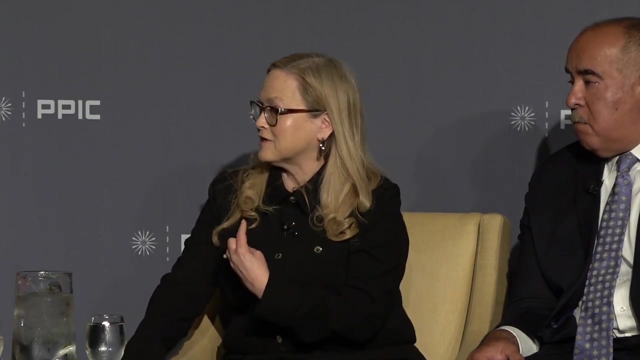 quality childcare that's affordable. It costs $20,000 for childcare for one year for one child In our community. it doubled in 10 years And the childcare worker is still at the lowest level that she- primarily she- can possibly make. And so the real 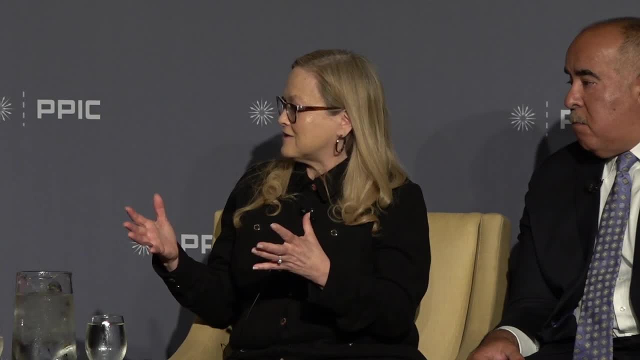 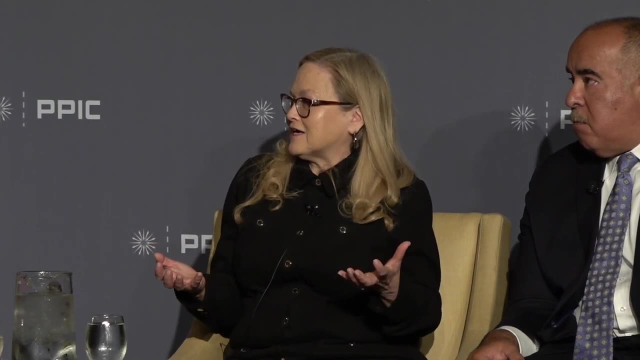 question is in my mind and I think your point, and I love that you say that the economy's about people, because the real question is, as a community, as a society, what do we want our society to look like And what are we willing to do? 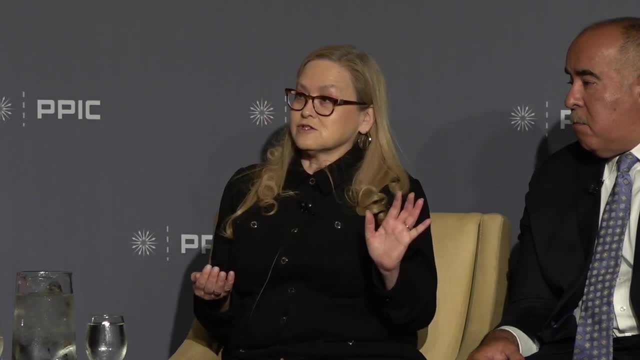 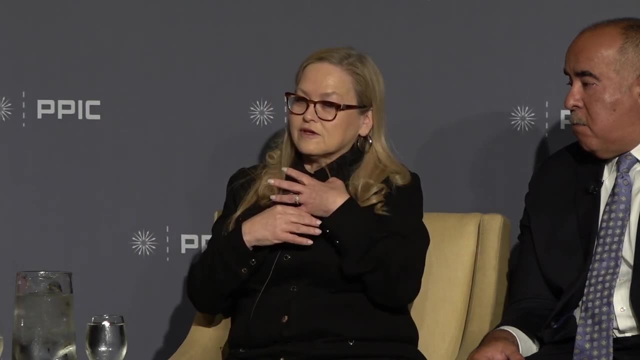 to get there And you talk about removing regulations, which I think is a fair point, And I think in some areas we need to add them, Because what's happening in our community is we have investors coming and buying hordes of homes. 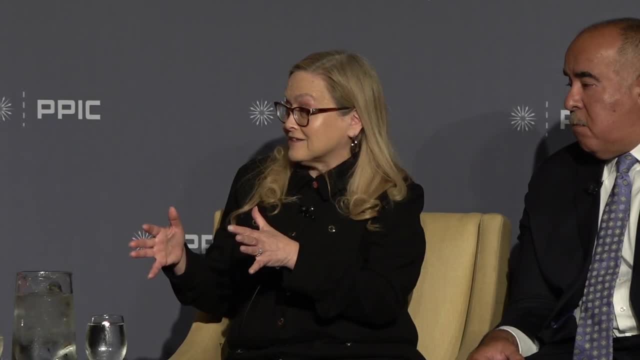 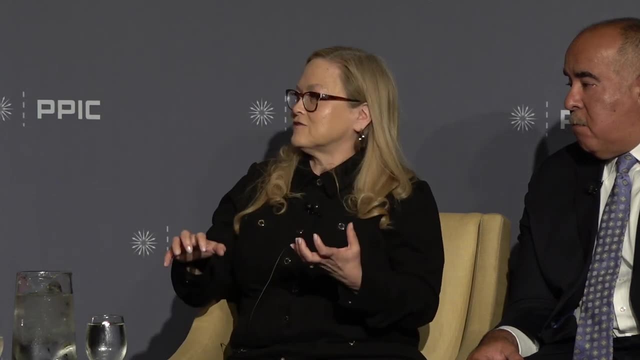 hordes, literally keeping them vacant while they wait to get somebody in them. That is an economic pressure that's adding already to the pressure that these families are feeling. So that's why I'm like I'm done with incrementalism, maybe too, because I'm going to be. 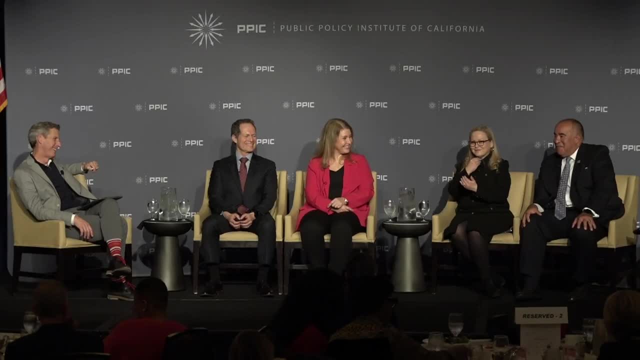 60 soon and I'm sort of like done. No more of that We need, we don't? we don't have a lot of time left on the planet. I want to make things happen. Amen. I'm going to skip you, Sarah, on this. 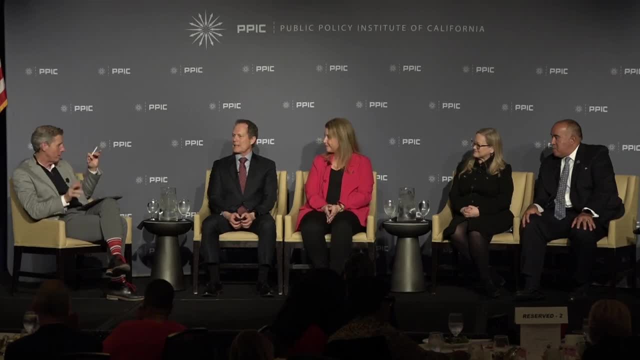 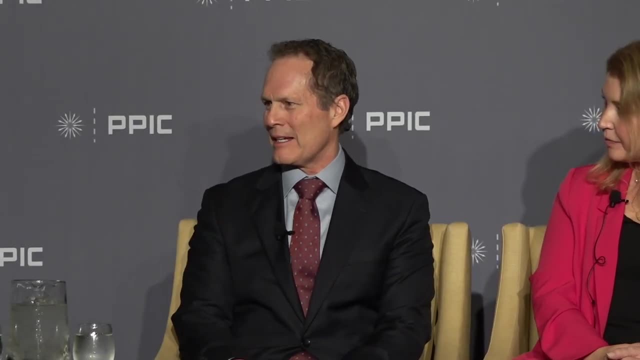 too damn expensive. question, Reuben, over to you, Put your business hat on here. It's interesting because you say that it's too expensive and everyone goes to housing Because it is right And again, that is a driving force. The. 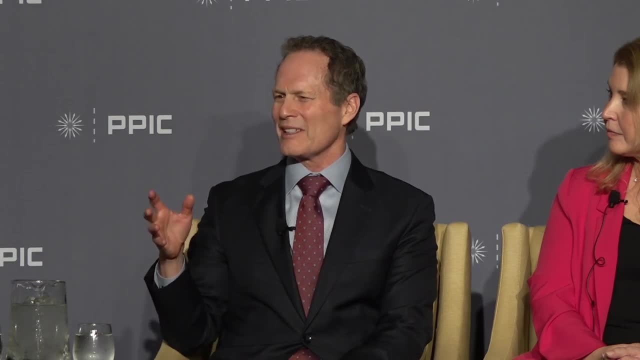 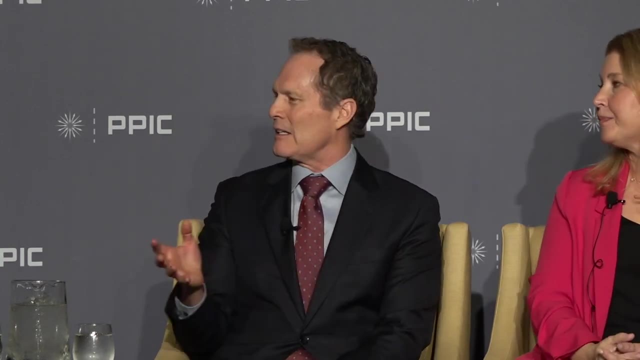 hundreds of thousands of people that are leaving California, which is really almost a rounding error in terms of a 38 million population. but a lot of them are leaving. I know this because I read the PPIC blogs. Are leaving because of housing. 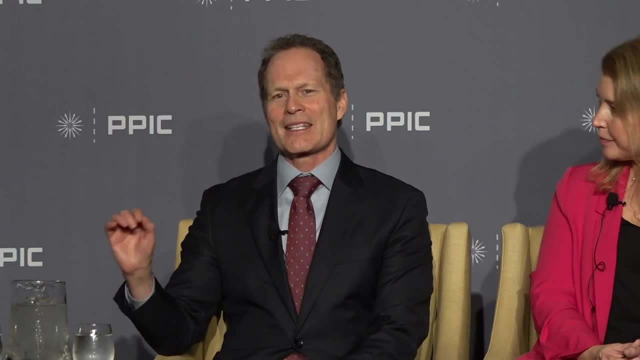 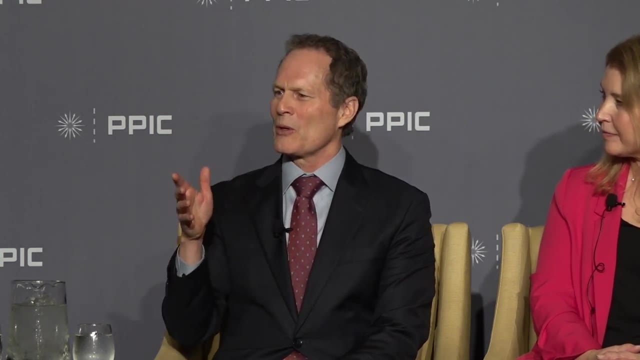 right Jobs and housing. So not to answer your question directly, I guess maybe I did. it's housing. For me, the beauty of California from about 1849 to almost 2000 was, you know that whole manifest destiny in terms. of like. you can go, you can build a life, you can own a home and create generational wealth. People are looking for that outside of California now, So that to me does not bode well, except again, I think California is so big and 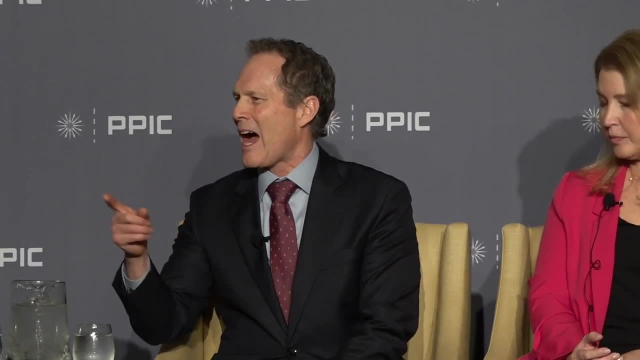 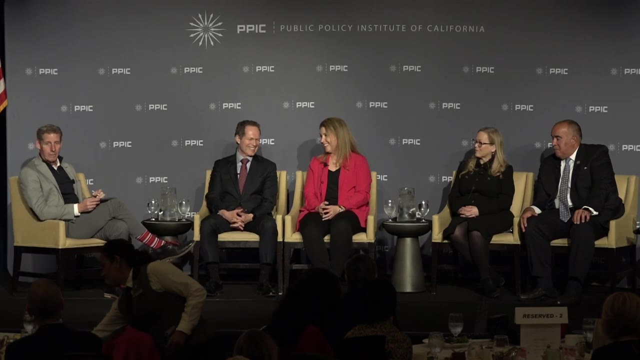 there's so much to it that we can't overcome that, And so housing supply for me would be kind of where to focus Man. we're going to need more than NMR on this conversation, So look not to put you on the hook, Sarah, for something that. 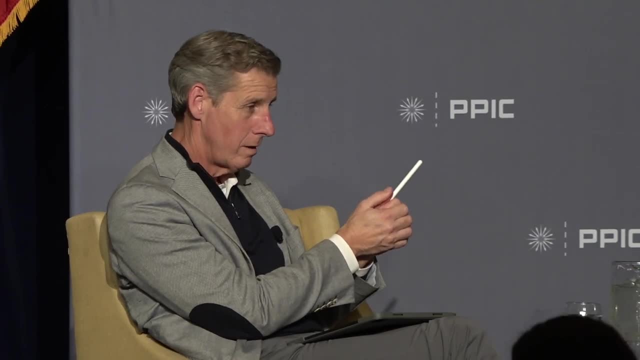 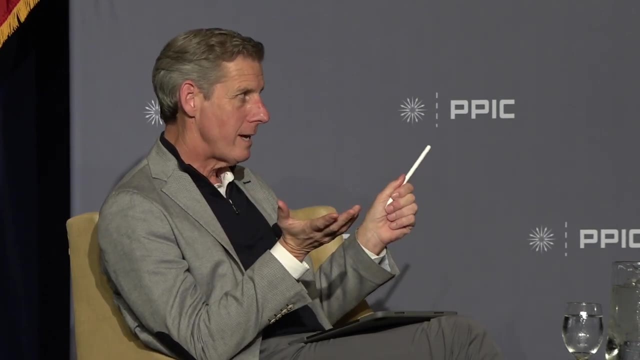 somebody else at PPIC wrote, maybe on your staff, I don't know. Dean Bonner wrote a thing about: is the American Dream in California dead? Just building on what Ruben was just saying, A lot of people in this state say yeah, maybe it is. 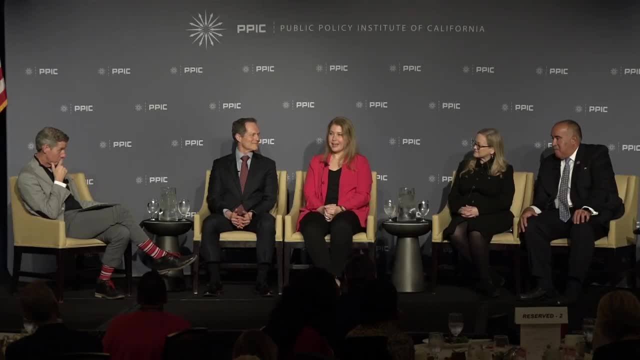 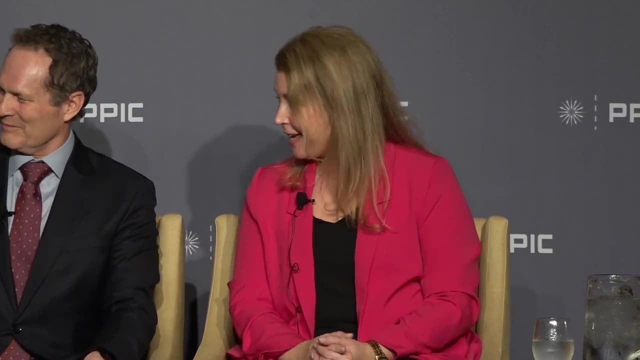 What do you think? That is what our survey shows Californians are very pessimistic about right now. They're predicting recession. Hang on, I'm sorry to interrupt. If we're pessimistic, how do we do these really aspirational things? 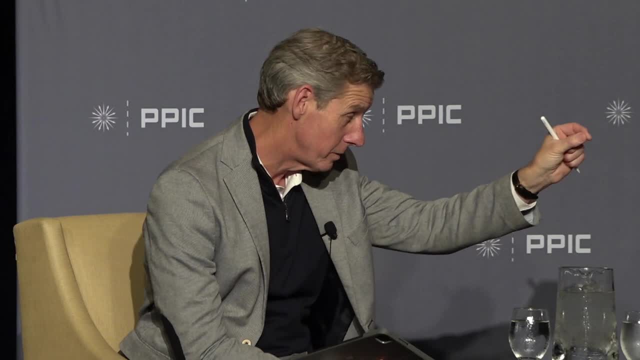 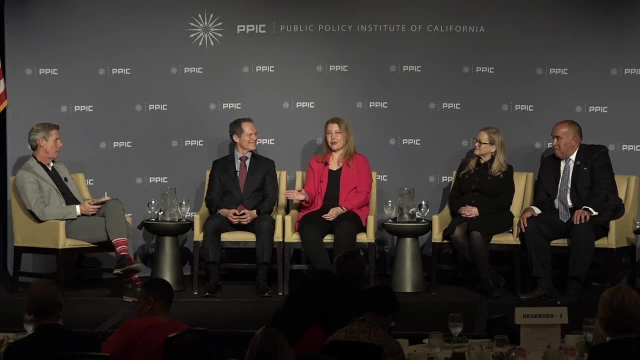 Which I know. you're an economist and it's not your job to figure that out, but it's Cindy's job. But how do we do it Right? Let's do a little solutions journalism here, Okay. so one more dismal point, though Stop. 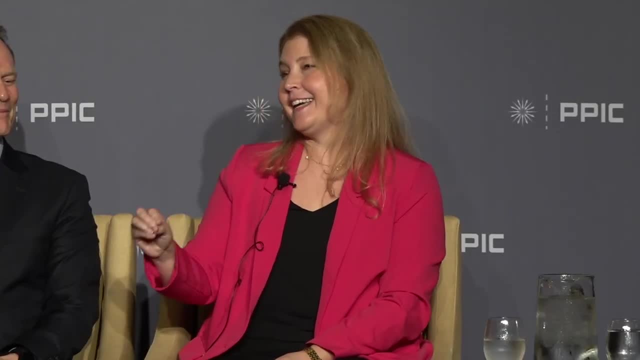 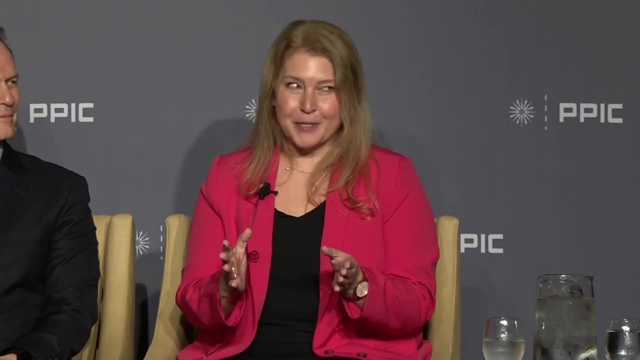 I'm going to get there, I promise. I think it's about mobility and it's about the future for our children. The dismal point is that Californians- are 70%- think that the state's children will be worse off financially than their parents. 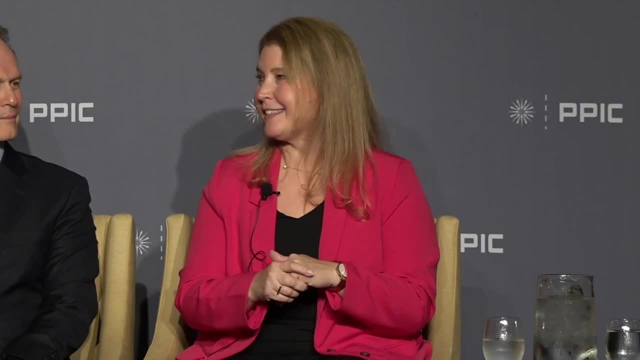 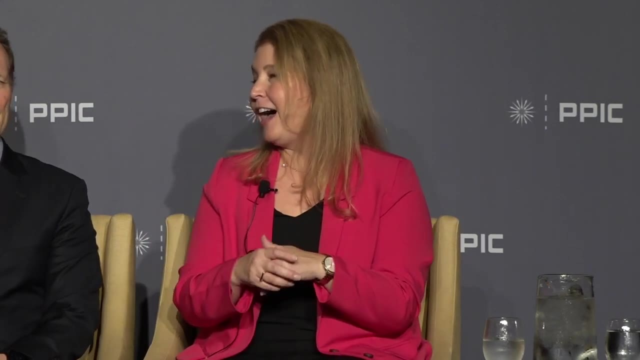 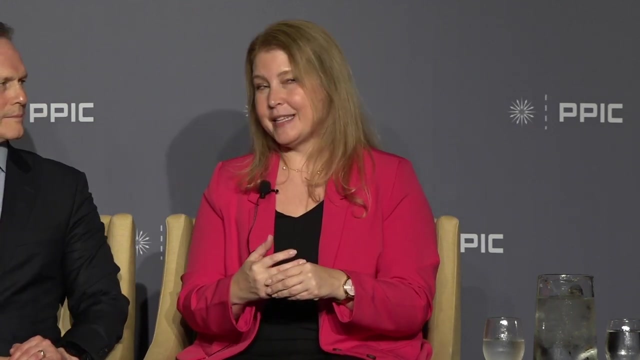 when they reach adulthood. That's been a persistent finding. That's not just like a recent pandemic thing, But I think we all want solutions for our children to thrive. Maybe some will thrive outside of California, but I think that the chances for upward mobility and 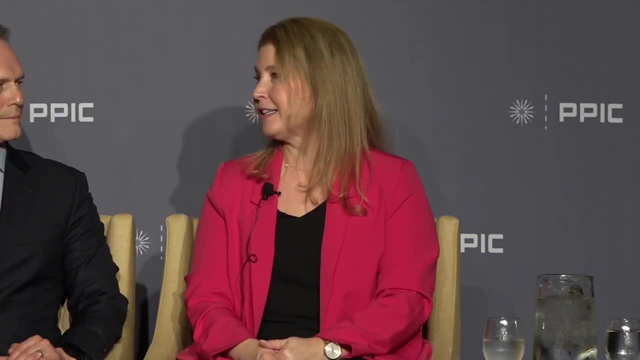 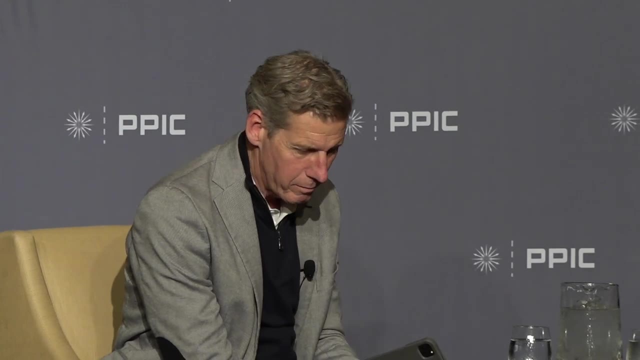 building more of that into what's possible in our economy, is there? So, Cindy, maybe you could get the governor on the phone. I don't know, But as you, I'm sure you have conversations with people in Sacramento in the state legislature, right? 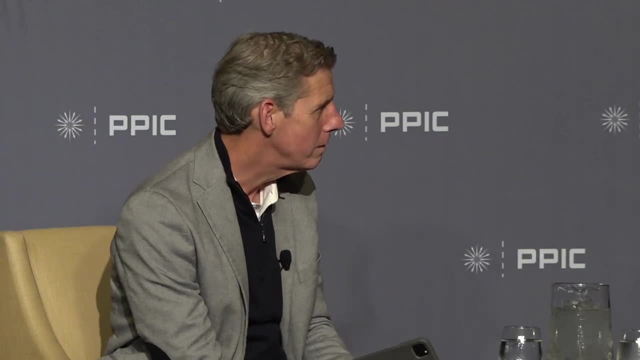 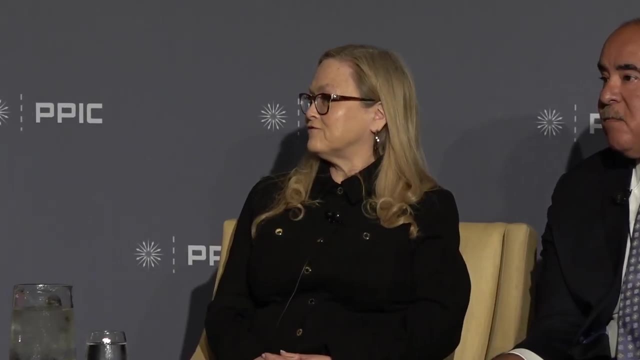 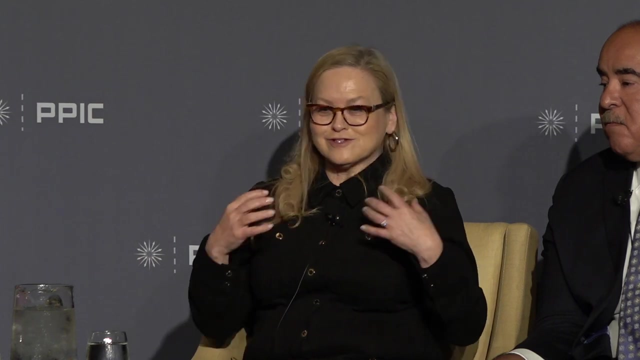 Do they appreciate any sense of economic urgency? I would say yes, and I would say that just based on the flurry of bills that are focused on housing and trying to remove local control, because I think at the state level they're saying: oh my god, you cities, you're a hot mess. 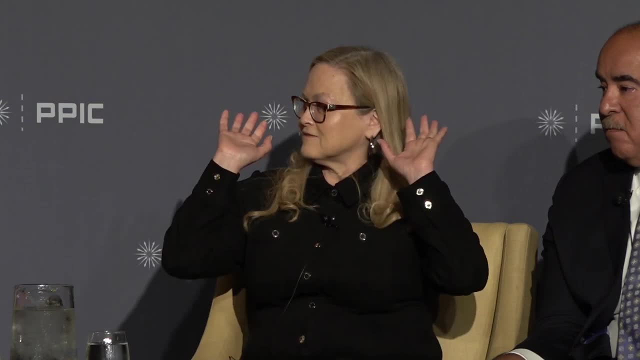 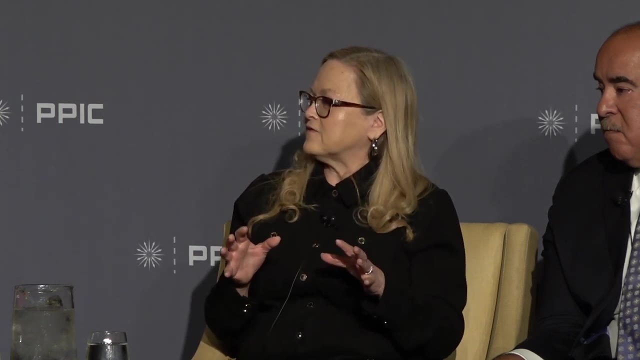 And so we're going to get in and fix you, And part of that is removing what they perceive as barriers. So, yes, I think that's true. I think the challenge is that we, as Californians, haven't said: here are the. 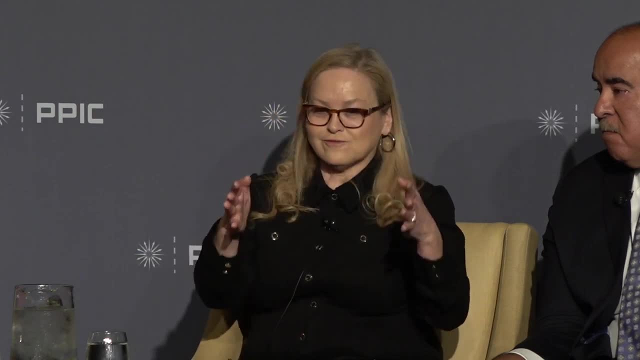 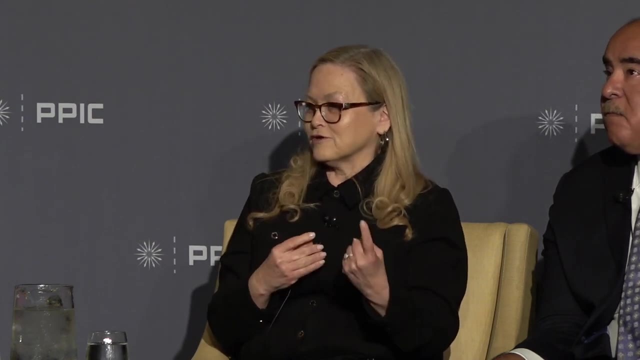 four things that we need to do to get us on the right path and focus on those four things. I'm old enough to remember Jerry Brown, the first, and when I think about him, I think about this idea that we're going to have the best. 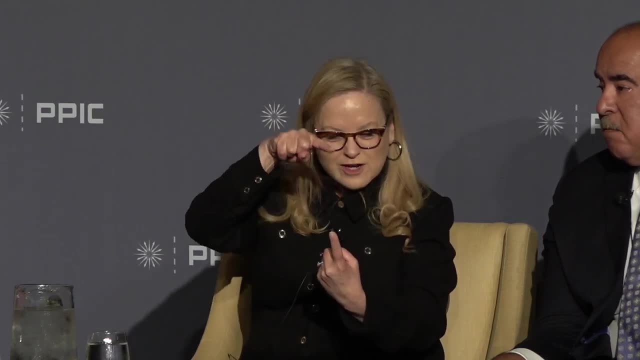 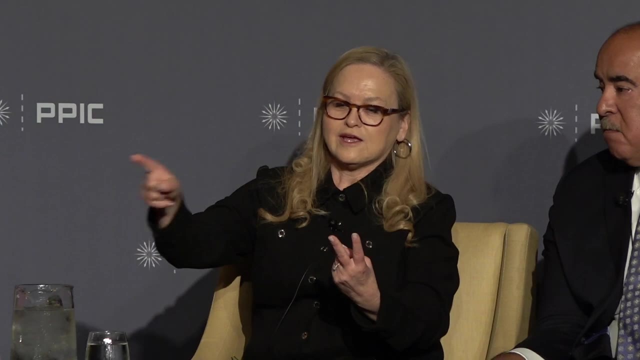 university system in the world, Not just in the country in the world. We're going to connect California with freeways and we're going to make sure that people and goods can get from point A to point B. And when I think about and we're 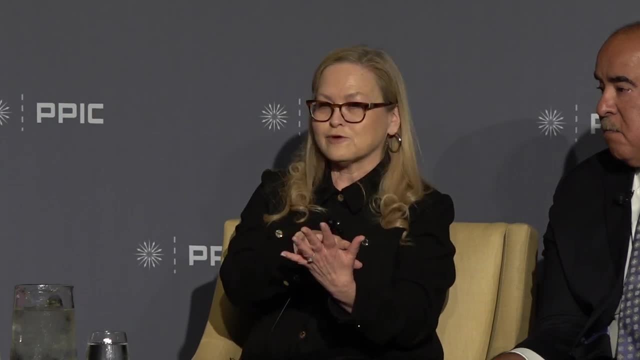 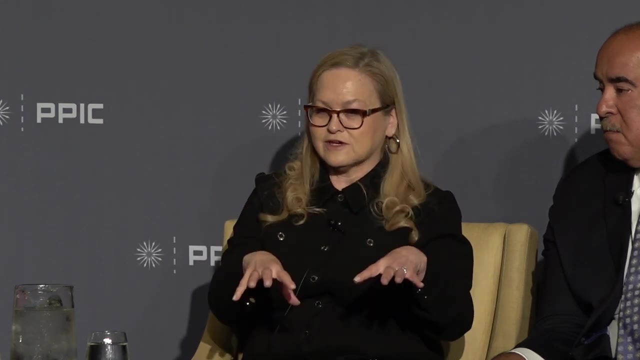 going to invest in schools, and that's at that time- this is pre-Prop 13,- you could go to almost any school in California and your social mobility opportunities were higher because the investments, irrespective of the neighborhood you were in, were closer than. 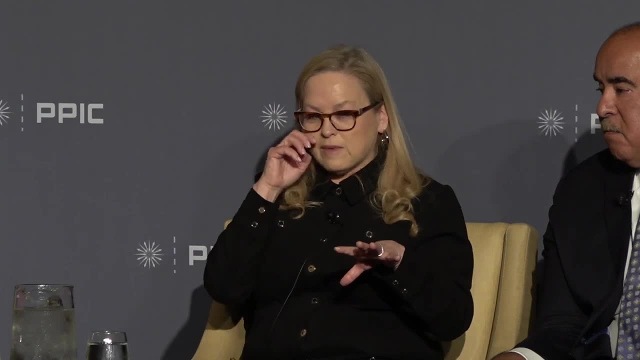 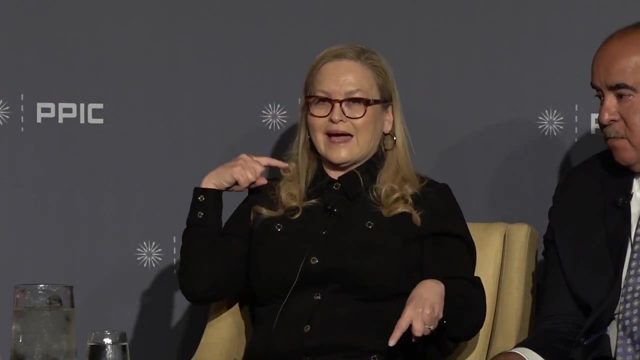 they are today. When I say that I'm kind of done with incrementalism, what I'm wanting to say is: what is the big plan and then how are we actualizing that plan at a local level that really allows us to shift this dramatically? 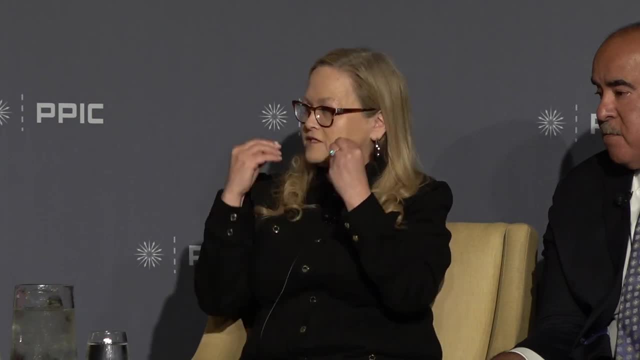 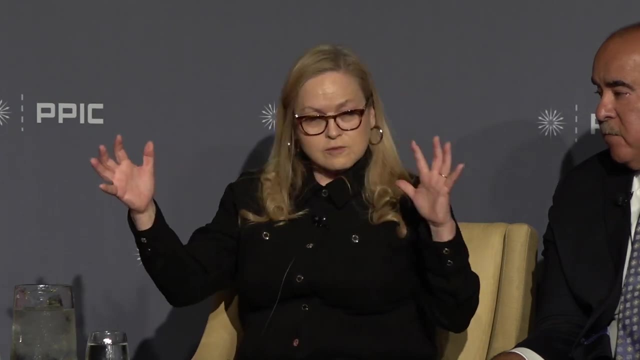 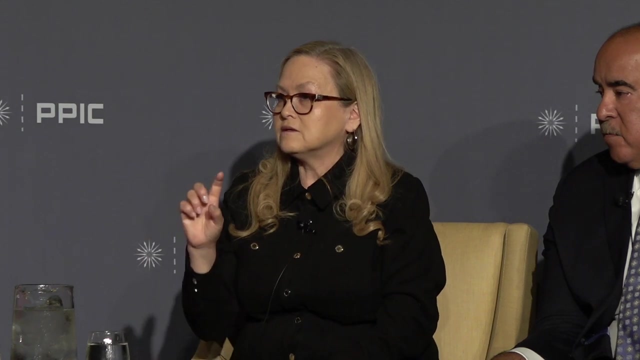 I just want to give you one more pain point, but then tell you why I feel excited about this And we in the community that I live in, if you go to school at a Palo Alto elementary school, we spend. that school district will spend about 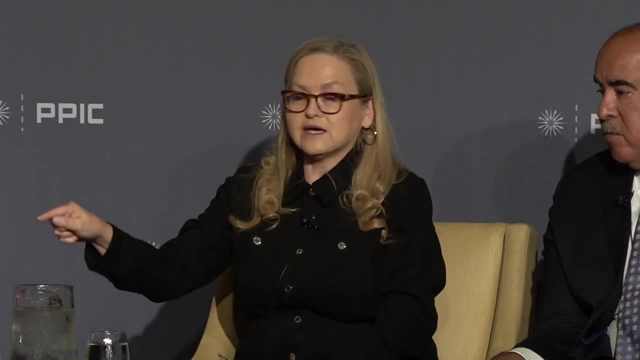 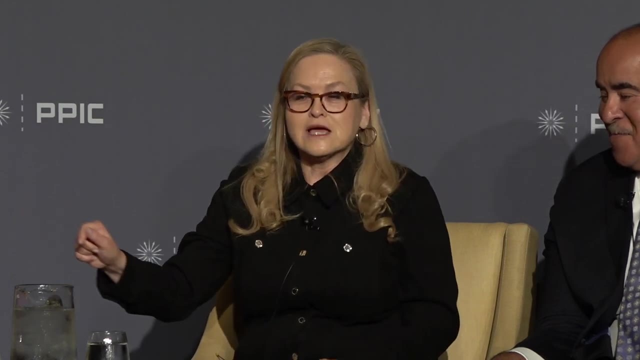 $22,000 per child to get an education where the homes are in the jillion. I'm going to go above the millions, The high jillion, The high jillions. If you go to the district I represent and you go to, 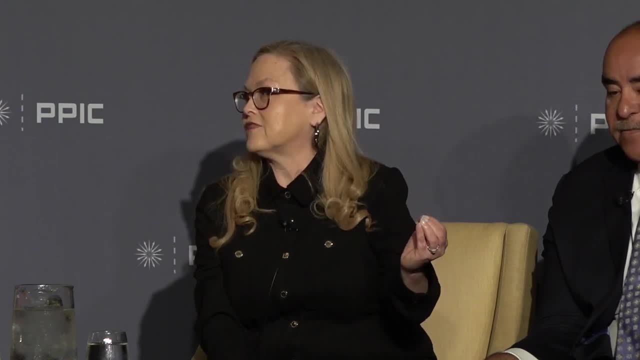 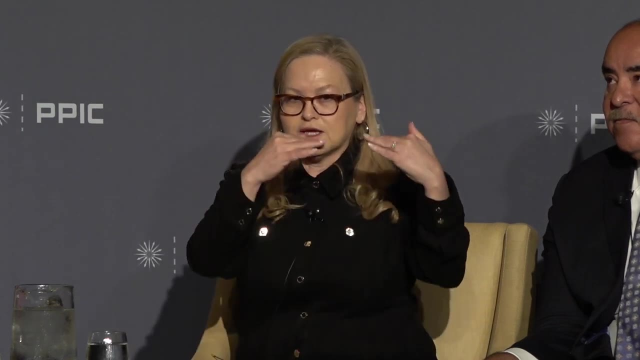 an average school district. in my community elementary school we're at $11,000. And so if, in fact, what we're saying is that we want young people who can get into these jobs, we actually need to have a fundamental shift in the way we fund. 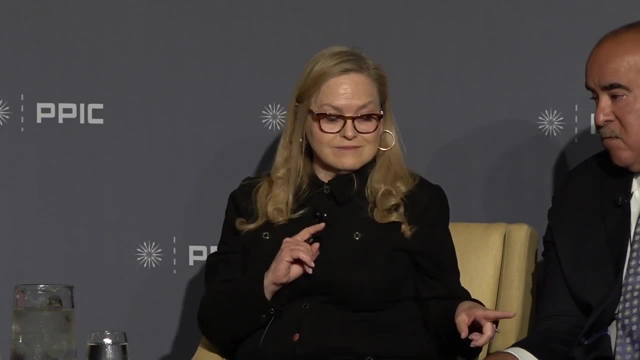 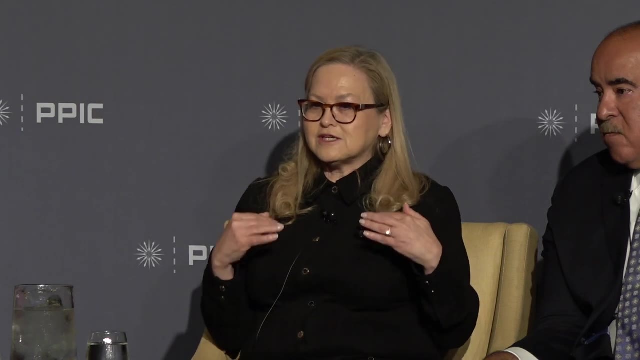 institutions and the tradeoffs- And there are a lot of tradeoffs that we have to think about- but being able to do that again with some urgency and direction, with the idea that the fourth largest economy in the world, the way I think about it is like: 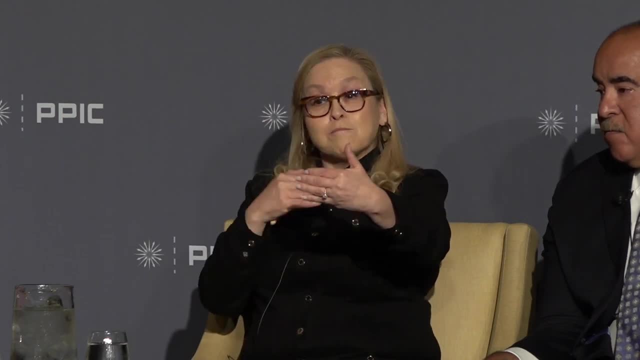 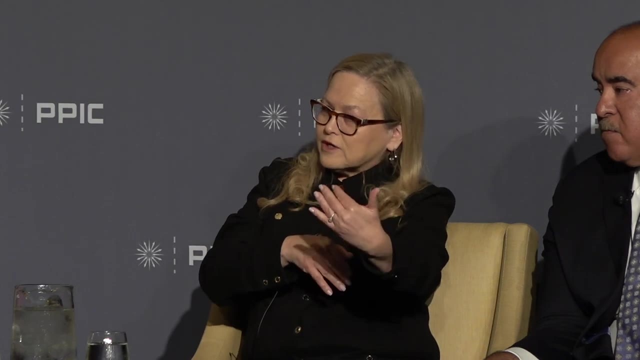 a ship that's imbalanced And it's a big ship. it's an important ship to the United States, but if it tilts, if we lose the direction, if we don't have the assets and resources where we need them, we are going to be in. 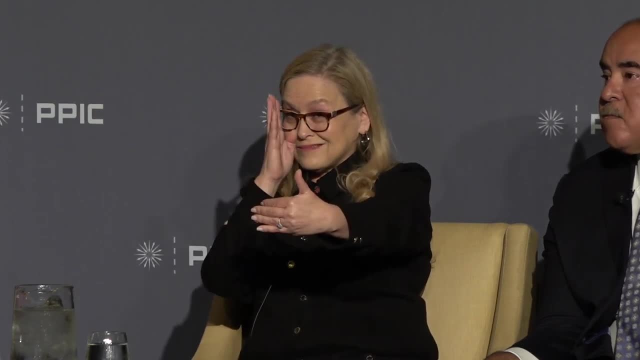 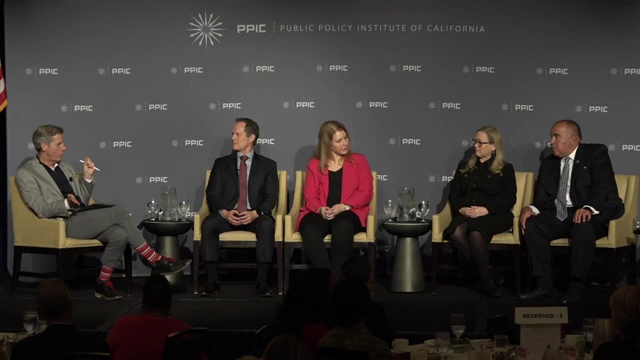 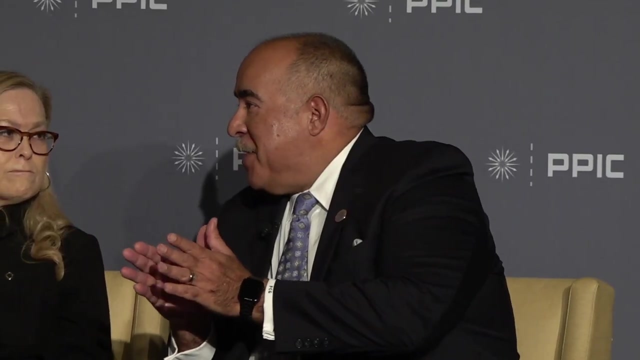 big trouble. So now I say, how do we right the ship? and you know, get moving Right. So, Paul, do you think the risks are that the ship tips more or do we right it? So clarification, I said align. 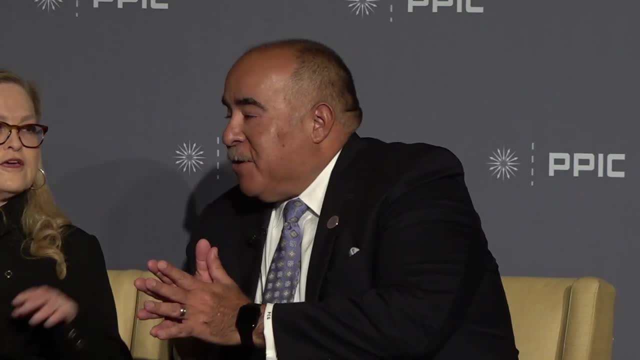 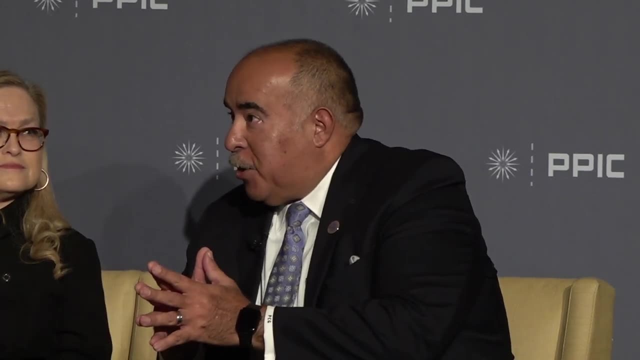 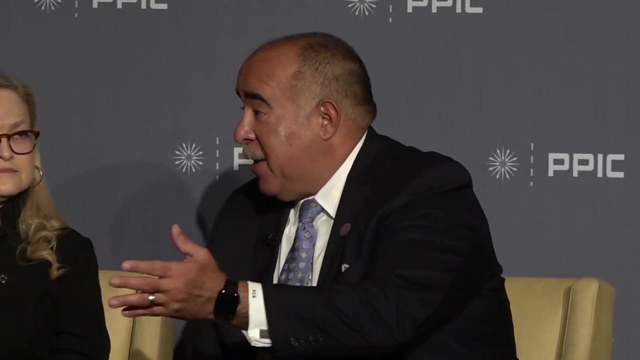 regulation, not remove regulation Fair. Yeah, thank you. I think that that's the question. So in Southern California, we're a goods movement hub for the world. Thank you all of you who are ordering from Amazon as you're sitting out there. But we are the cause of the growth of warehouses and trucks. We are the cause because we are choosing to purchase goods in a different way. Yet in order to meet our regulatory goals in Southern California, the EPA is threatening to take away all of our money. 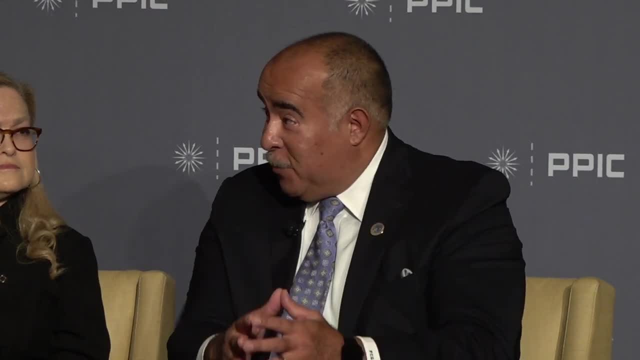 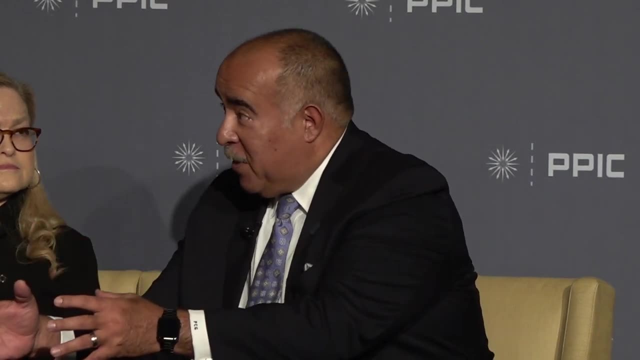 But the fact of the matter is is that the Air Resources Board has a piece of this, The South Coast Air Quality Management has a piece of this, The Federal Government has a piece of this, And you can't just say well, in order to hit that goal. 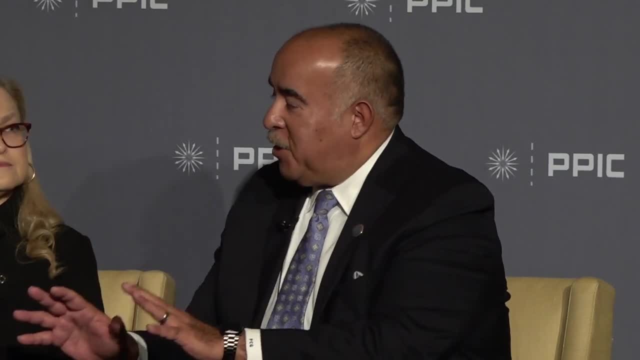 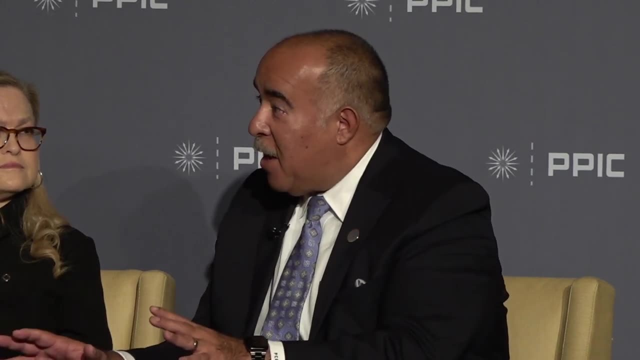 we're going to throttle the ports, We're going to stop ships coming into the ports, because then you're going to do a huge damage to a major driver of the Southern California economy, the economy of California and the nation. So which is it? 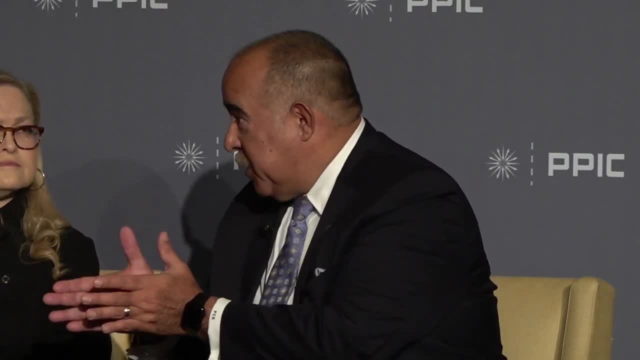 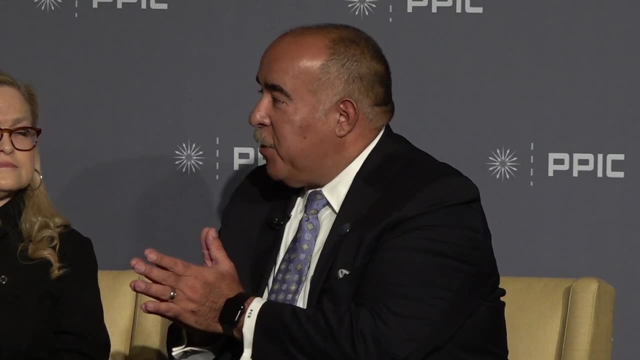 And it can't be one or the other. It has to be the alignment. And what I don't see, to your point, the plan. Where is the plan? California is, as Ruben says, an economy of decisions, And so we have to. 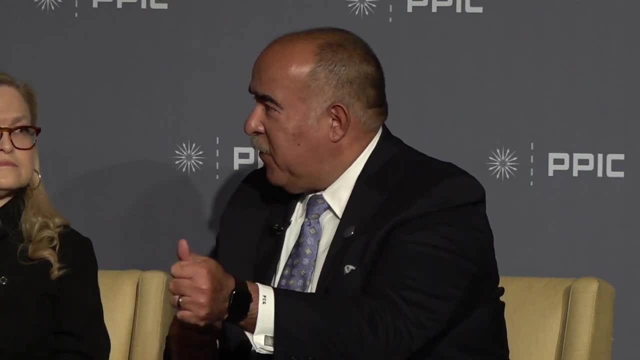 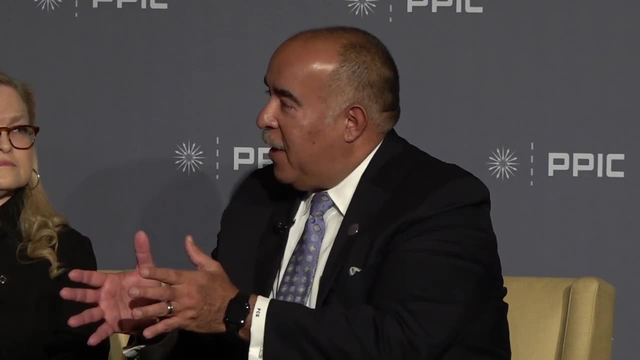 look at the Silicon Valley and say what's good, what's working and what needs to be fixed, And do the same in the Inland Empire and in the Central Valley. But that's going to need someone's going to need to sit down and create a plan. 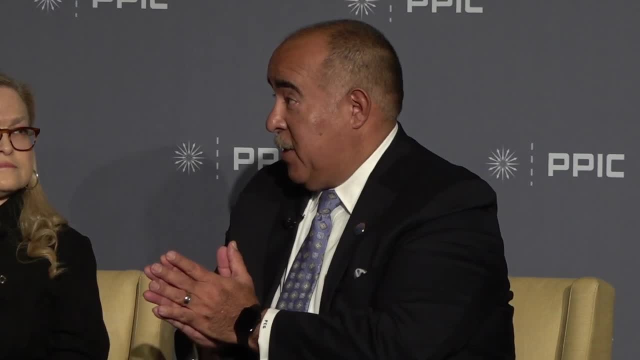 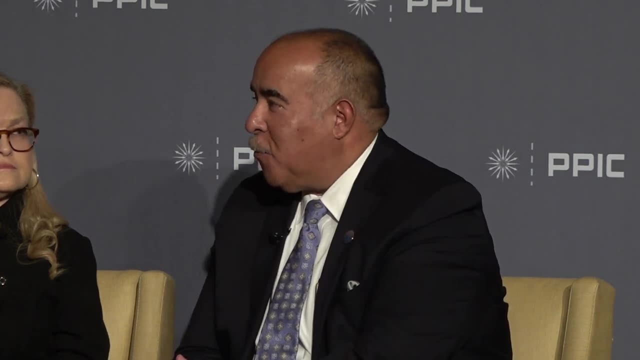 The Lieutenant Governor Newsom. he advocated for a plan, But we don't see that out of the current administration And I just think that we have to go back there. We're all smart people, We're Californians And we can fix our problems. 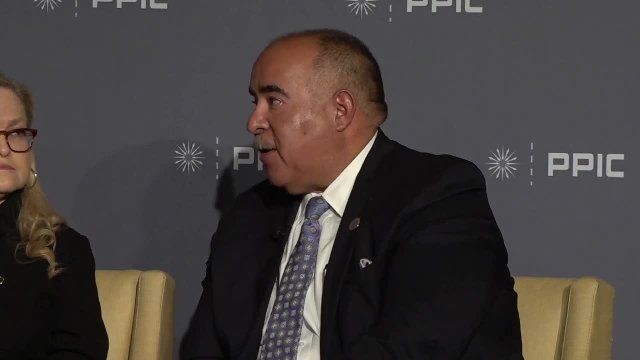 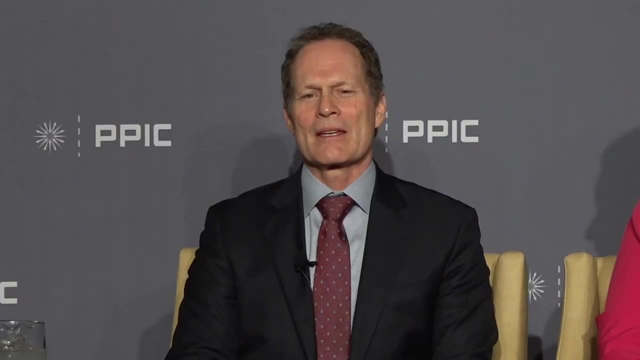 But we have to have a place to come together and work on doing that hard lift. Ruben, is the risk to the upside or the downside for the great state of California. Well, I don't know, I'm in the camp, kind of like. 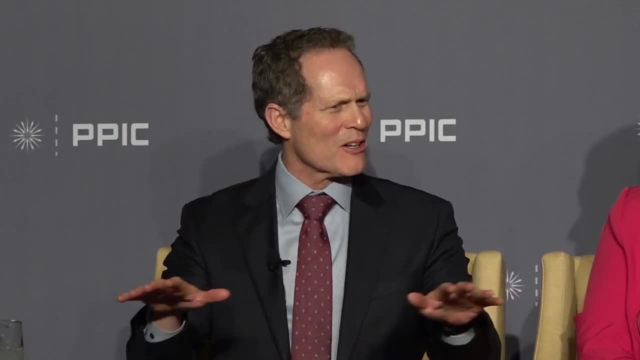 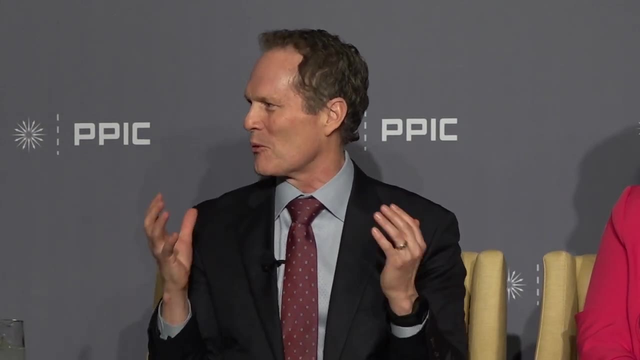 more GDP, the better. And then the policy makers, you all here in Sacramento, kind of figure out how we deal with that and make it more equitable. But like: grow the frickin' economy, Grow the economy, Create more. you know, I don't know. 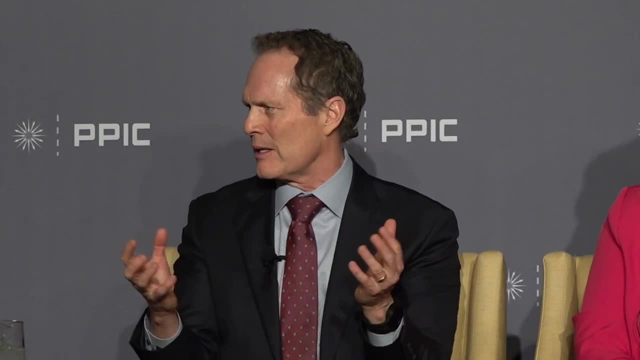 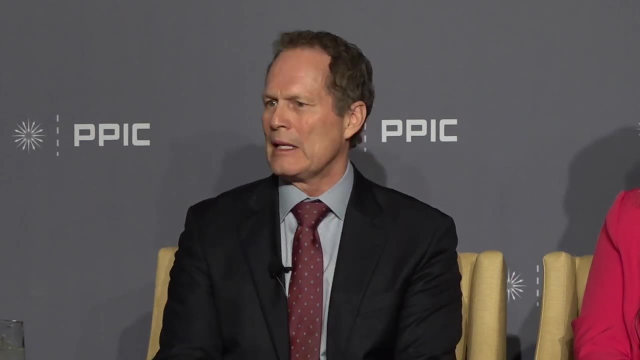 anywhere in the world where you go, where there's not some inequity, imbalance. I mean, we definitely have it in California. We've got more people under the poverty line, I think, than any other state for sure. So that's why Sacramento, you know. 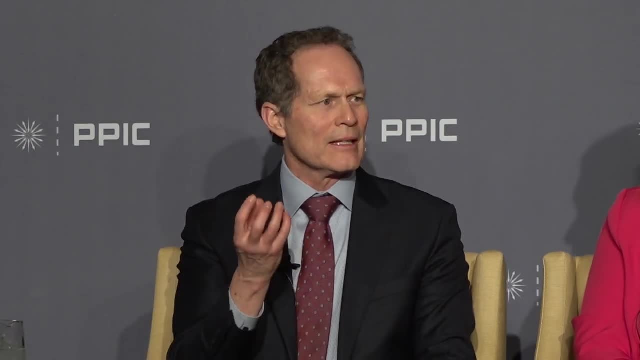 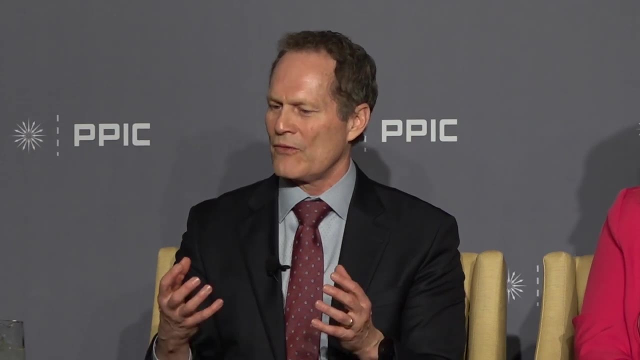 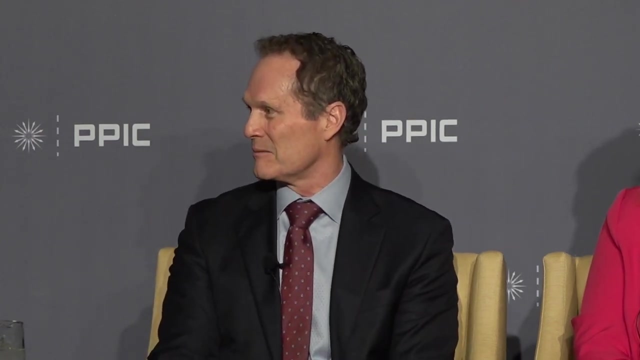 policy is so important in terms of, you know it's having labor and business, the public sector, private sector- labor together trying to figure out how do we grow a more equitable economy, But grow the economy Okay. How do we grow a more equitable economy? 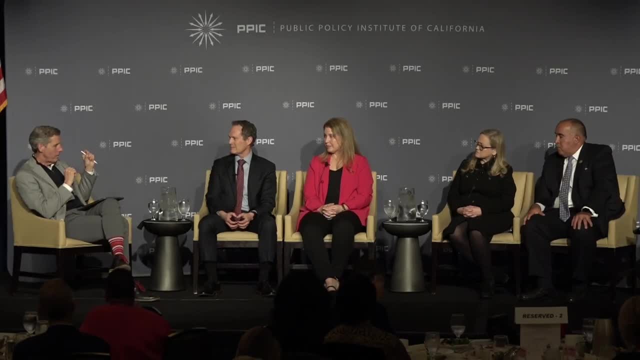 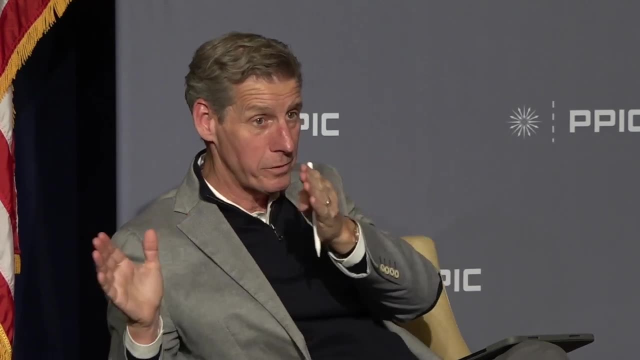 Here's the last question for me. then we're going to open it up. You all get one magic bullet, You get a wave of your magic wand and, in keeping with you, want practical policy solutions, which is what this place is all about. Sarah, you get to go first. 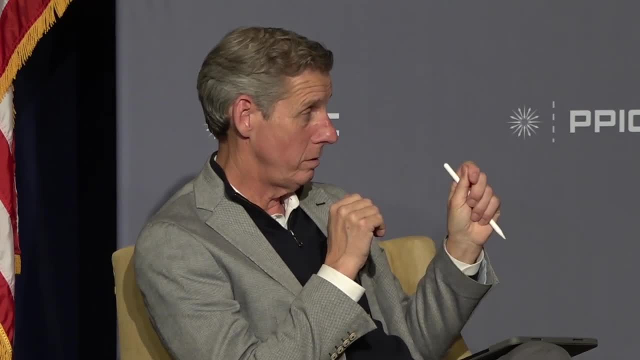 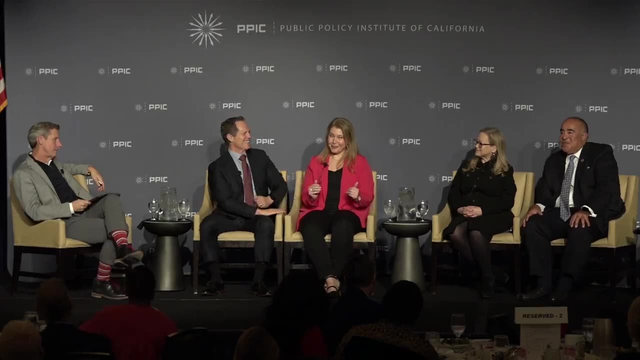 on this one. What is the policy solution you believe contributes most? The smart kid gets the answer first. I don't know about that. I'm learning a lot from all of you. I think it's if I had to pick one word. 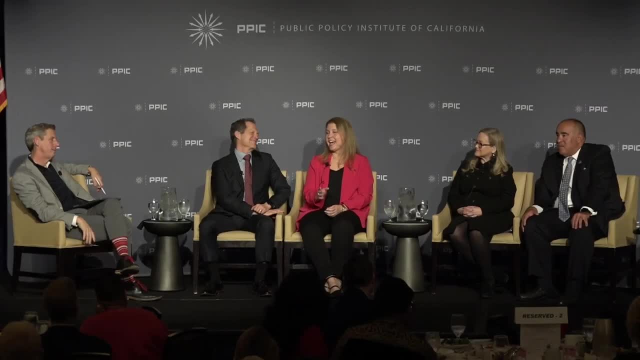 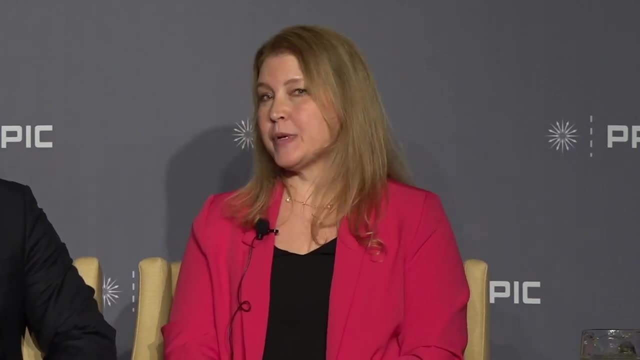 Sorry, it's got to be specific. You can't give me this wiffle, waffle or whatever. It's skills, So education, It's education, it's training, it's retraining, it's access to what makes an entrepreneur. 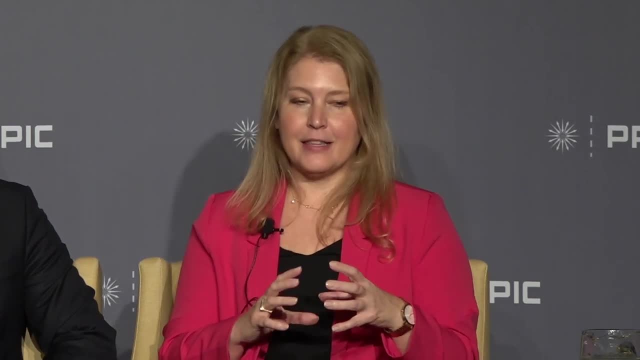 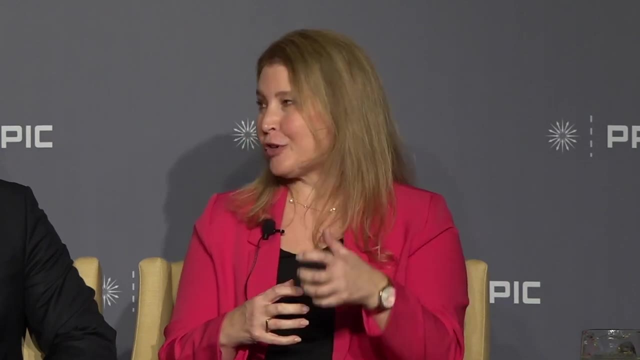 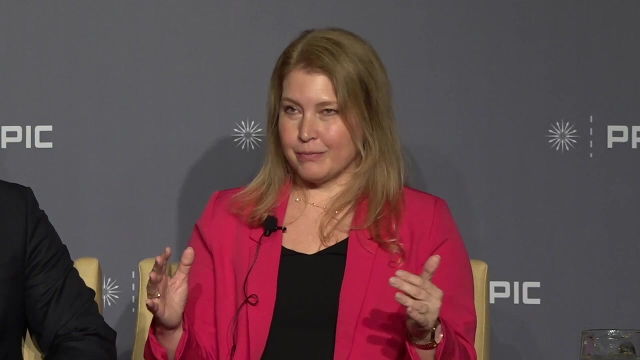 successful. It's all of the kind of building on the diversity, the skill, the potential of Californians and connecting that to future opportunity. There's a lot of systems that we've created for those purposes. I'm not. There's a lot that works within that. 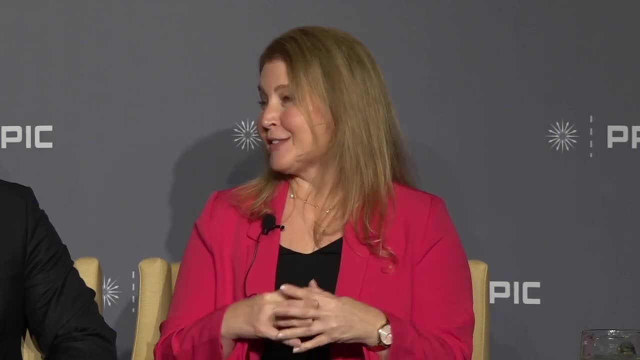 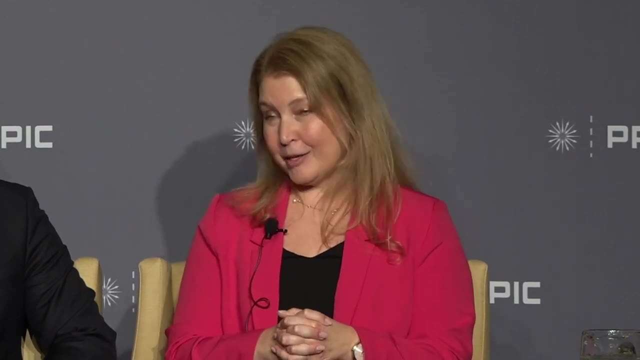 There's also a lot of lack of access. There's the costliness of education. Even investing in retraining when you're working in a low-wage job isn't really very viable for most people. We have a lot of those people and those jobs. 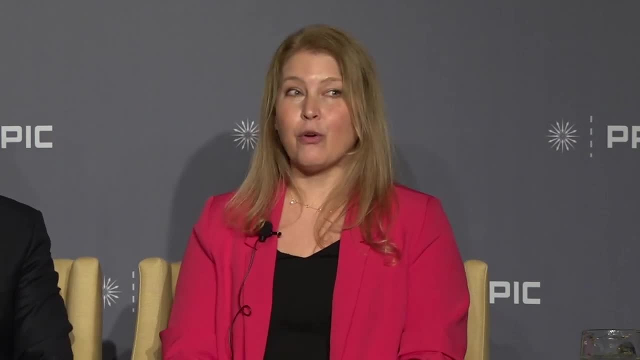 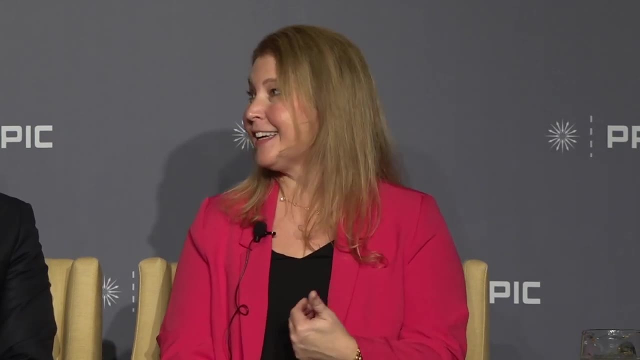 There's a lot of systems that we can work with or we can rethink them for the future, because I think we all need to know, as individuals, what those future skills are going to help us either maintain our jobs, going forward, if AI is going to take it over. 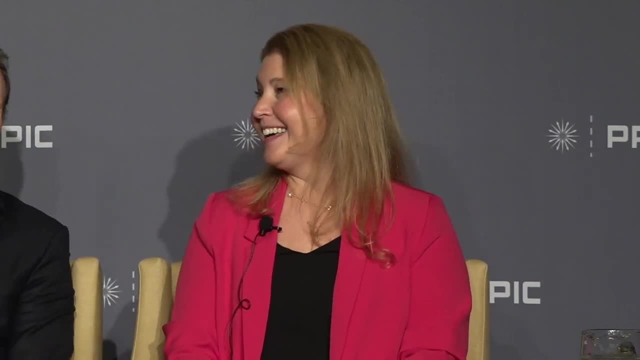 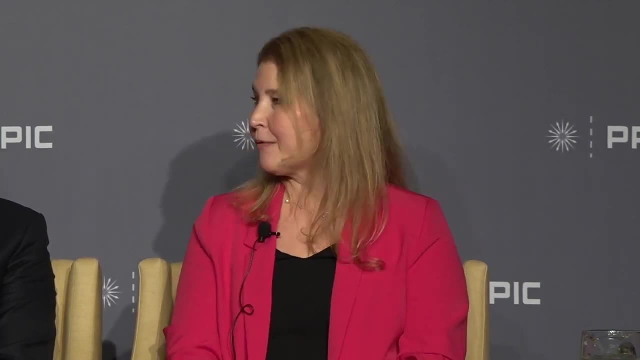 the role of the economist maybe, and beyond that, how climate change is going to affect the world of work. I think that is the baseline, the number one thing I would pick Cindy. Number one thing: Education. Okay, Ruben. 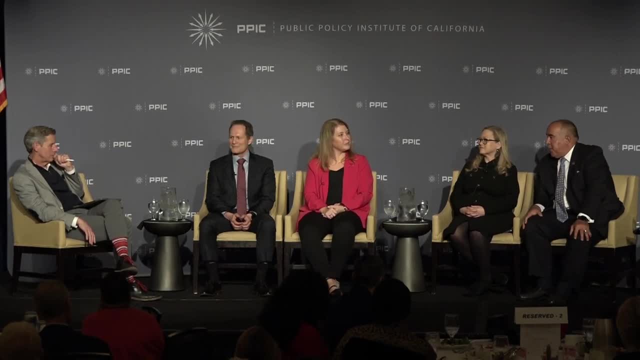 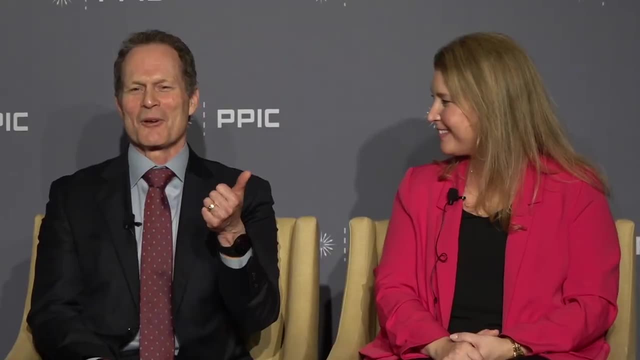 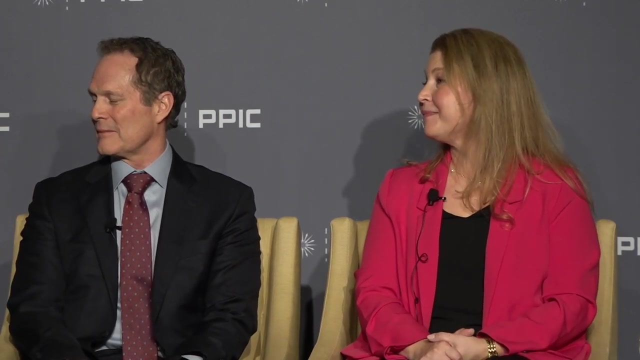 Paul, Sorry. Education and workforce- One word. So interesting, Cheater, I've got a compound One word too. Well, a number of words: Housing supply, increased housing supply and increased immigration. Yeah, Labor force. 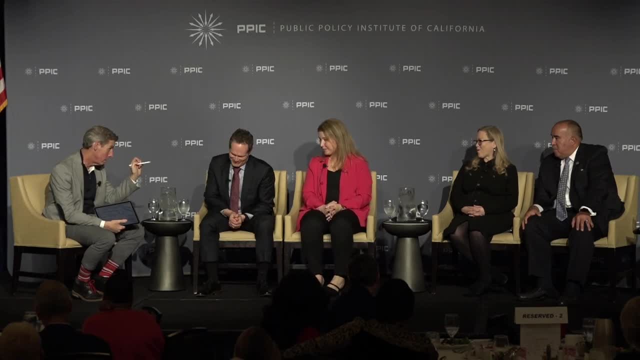 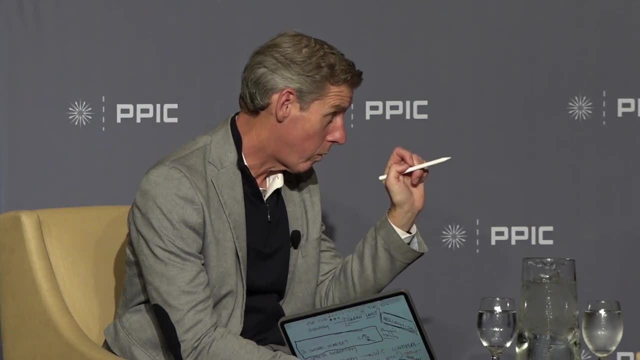 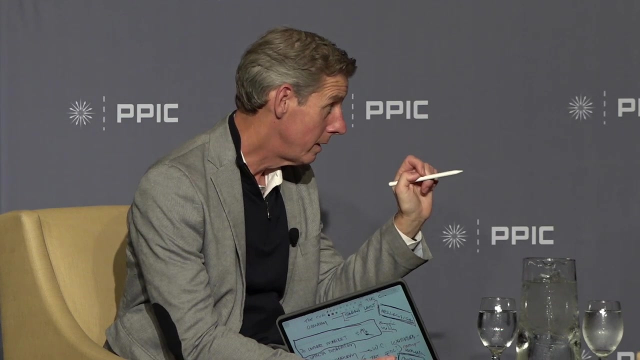 Sorry, I said that was the last one, but it's actually not. Let me squeeze you here, Supervisor Chavez. Leadership, which is required here, requires acts of sacrifice, political sacrifice. It requires acts of great wisdom and it requires an ability. 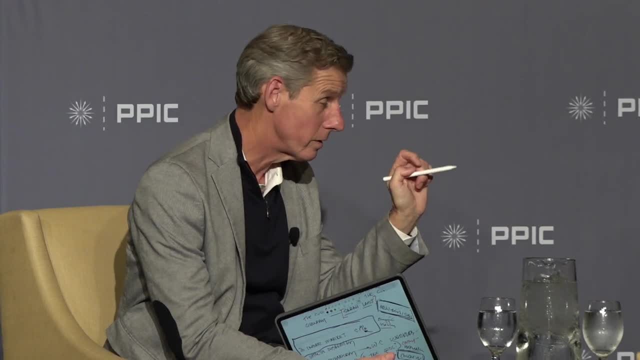 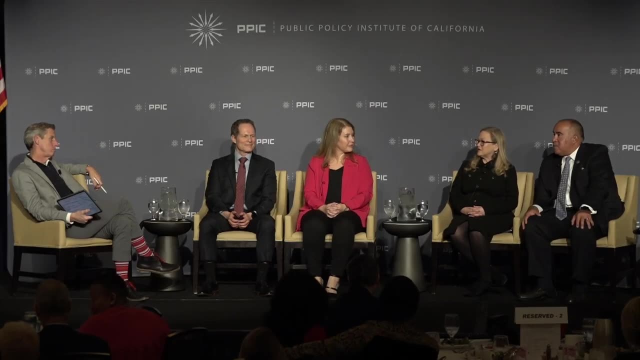 to see the future. My question is: do you think the politicians in the state of California- and this is really the one political question- have the guts to do what it takes to fix the state of California? I think many, many do. 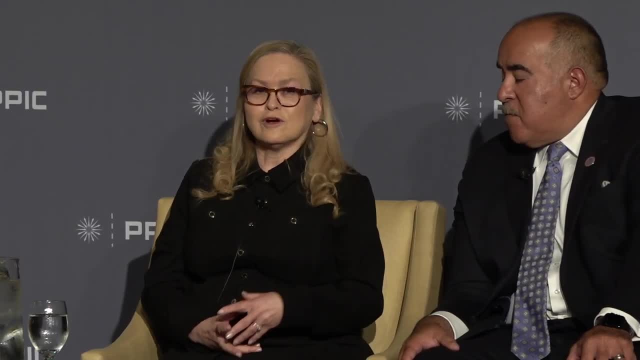 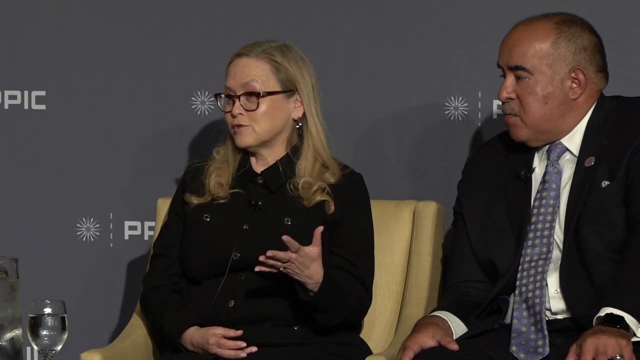 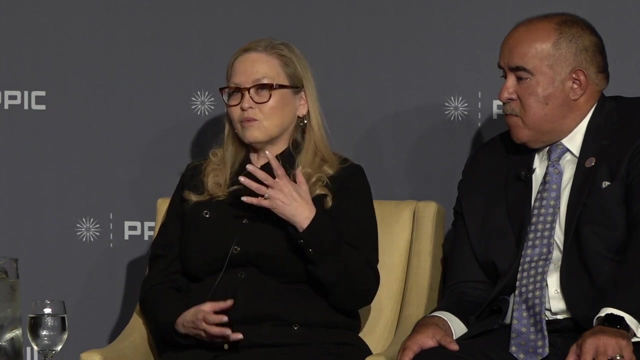 I really do And I would just say for all of you in this room: you know public servants and you know that so many are willing to die on more than one hill. I think really the challenge for us is that at a statewide level, 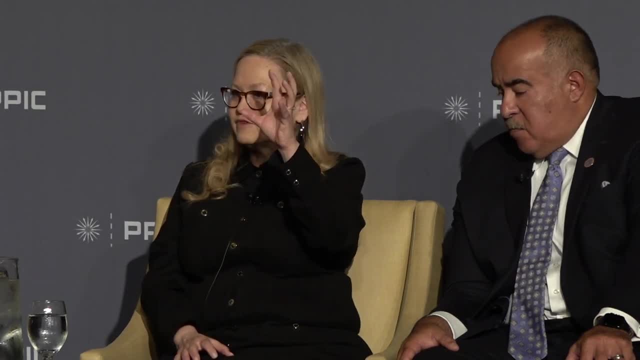 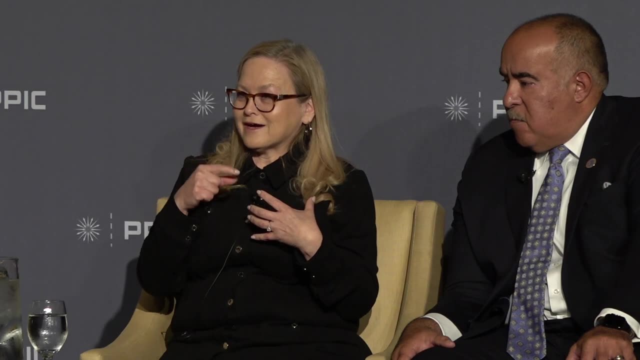 we not only need a governor with vision, we actually need- and this is something I felt with Jerry Brown when he came back the second time, which was he was a total grown up Now- I didn't agree with, I mean, I was mad at him a lot. 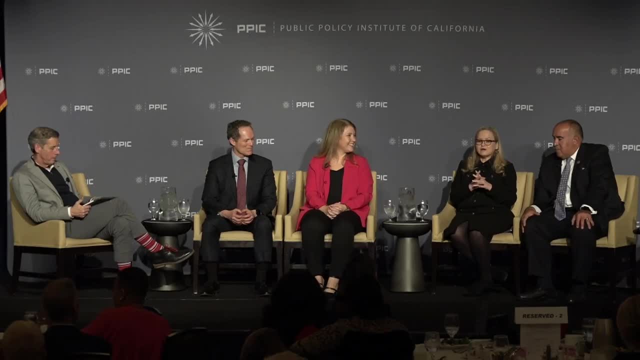 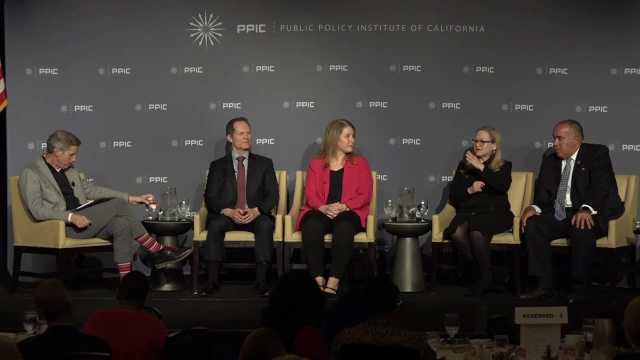 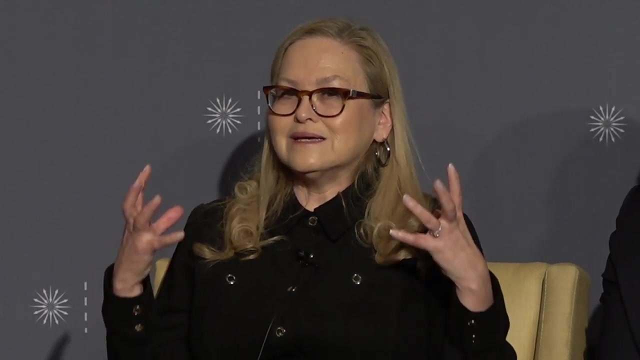 I think a lot of people probably- But I felt like he was willing to say no to allies. He was willing to say yes to his enemies, And so what I'm really looking for in the next crop of statewide elected officials is their ability to get. 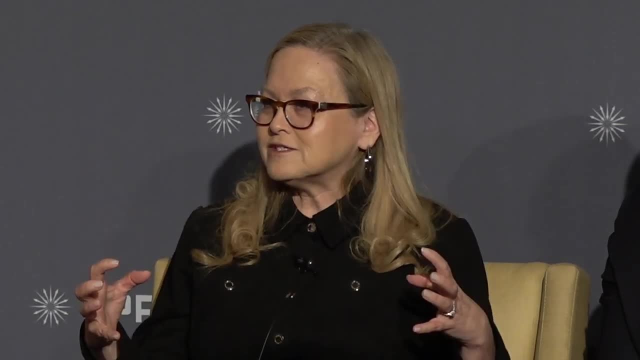 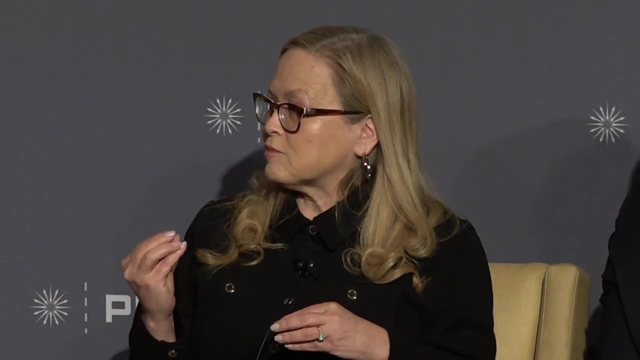 in a room and box it out and make people listen to each other in a way that people don't do anymore. And Ruben, you hit on this that when you're trying to solve a problem at a local level, you know, and especially 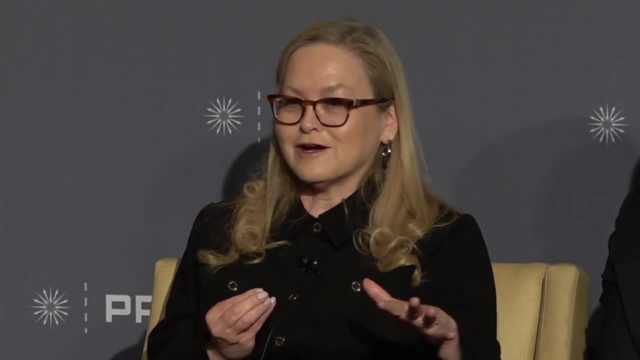 if you're a city council member, I feel so bad for you because everybody thinks you've done everything wrong. You're the mayor, like you're in charge of the world, But the truth of the matter is at a local level you can do this. 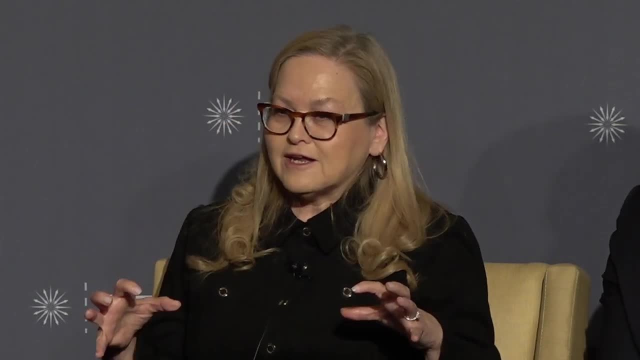 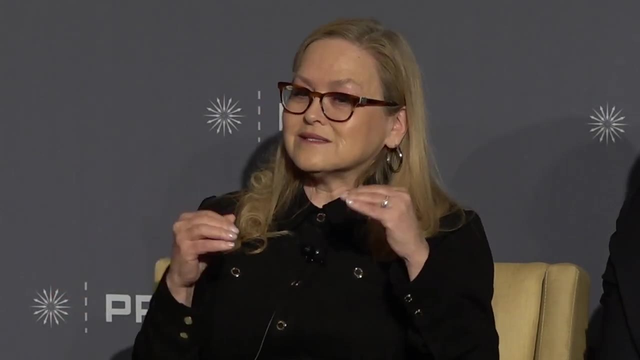 You can do that. You can get people in a room and you can fight out the details and you can make the kind of change that you want to make. We need that exported up, because what we're seeing instead is this top down control like okay, cities. 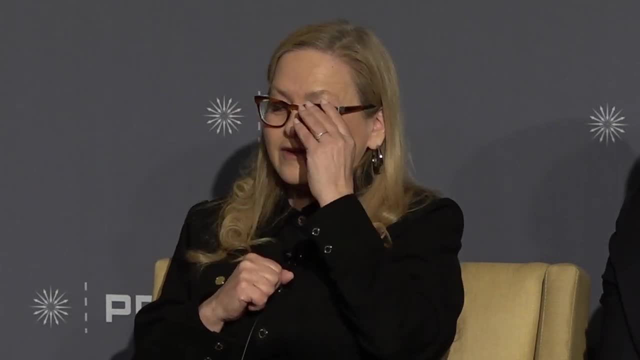 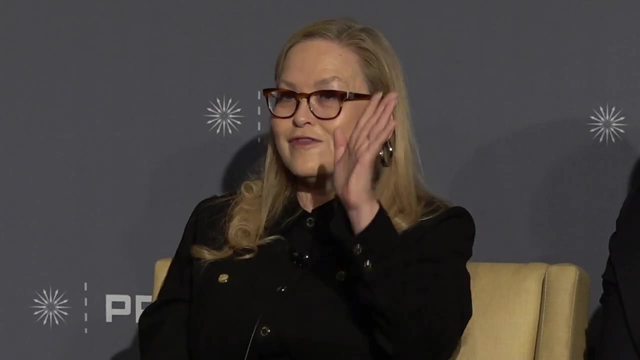 you will do this for housing or you will do that for the environment. I understand why they're doing it, but it's only meaningful if the actions they're taking at a statewide level are therefore not incremental and have the five, ten year, fifteen year vision. 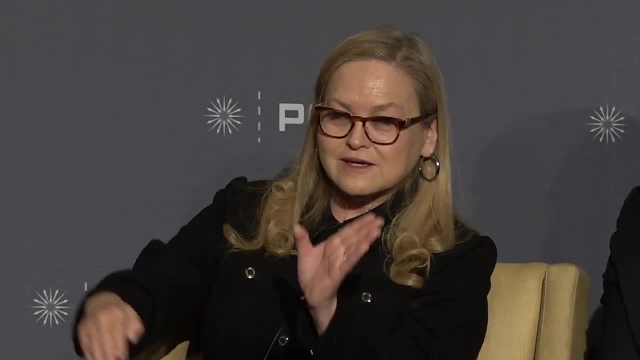 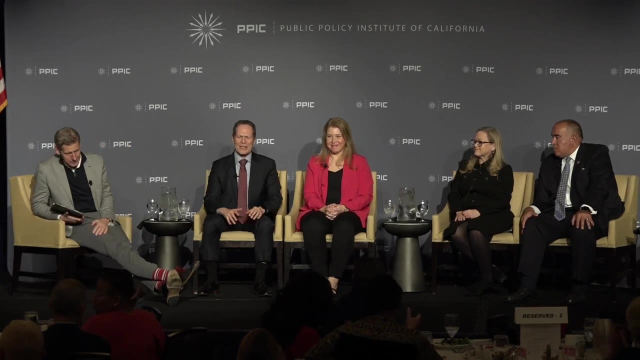 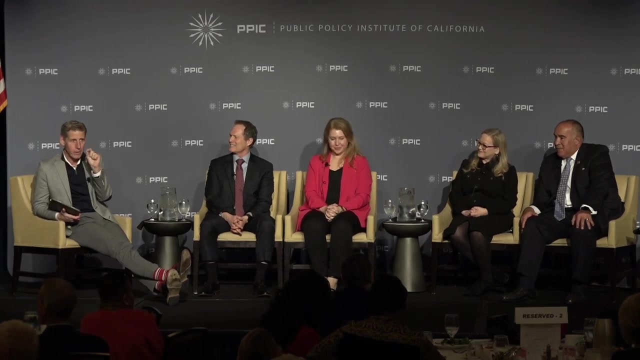 that says, by passing this and making all of you mad at me, here's why California is going to be awesome for your kids and your grandkids. That's why you need something like a PPIC economic center. Okay, so raise your hand, The mic runners will come. 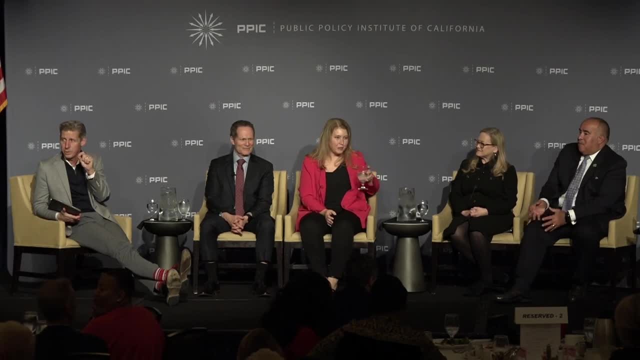 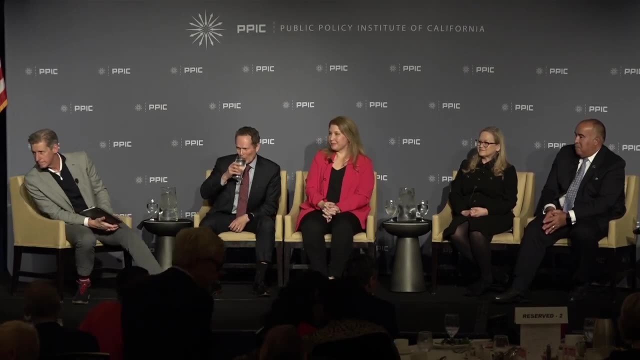 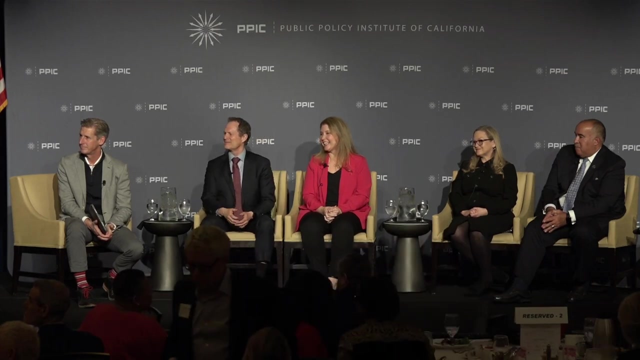 to you. Again. they will hold the mics, and questions should be in the form of a question. There's one over there. There we go, Let's go over there. They're going to hold the mics, Hold on So. 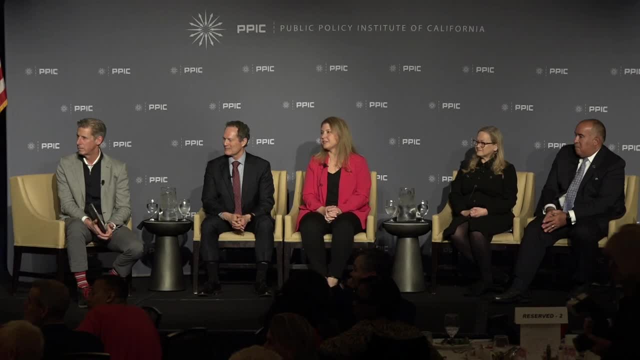 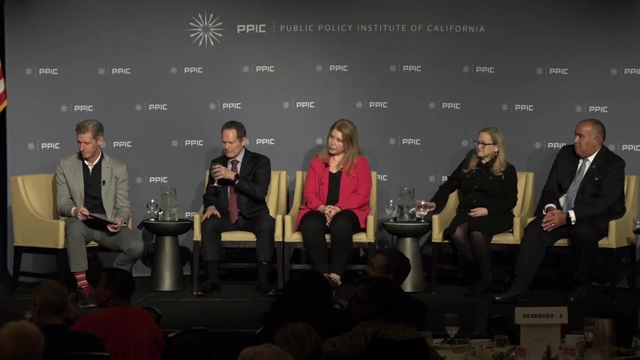 this past few years, after the with the pandemic, there's been a lot of economic pressure, and inflation has really been hitting people close to home and close to their wallets. Corporate greed has been a huge factor in this, and so how can California sort of hold these? 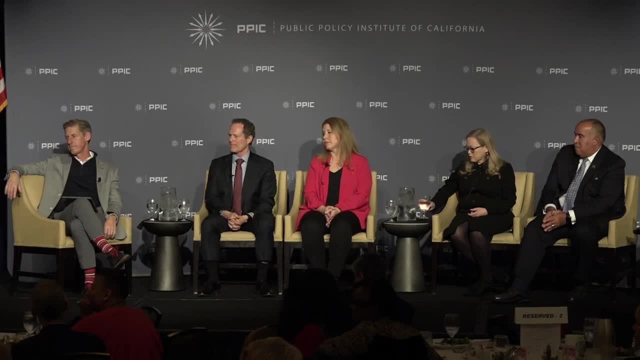 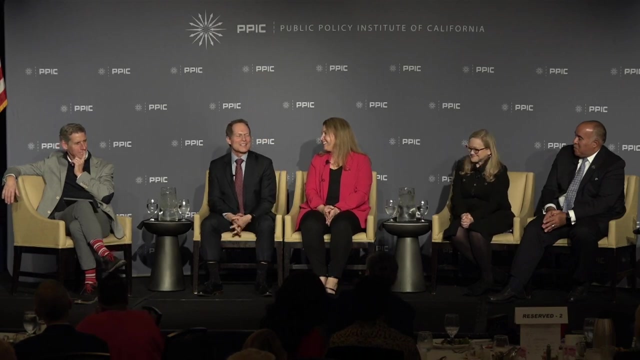 companies accountable for their role in this market manipulation that's been happening. Is there anyone on the panel who works for a big company? You get the first one. Well, you know, corporate greed, human greed, you know, I think it's. 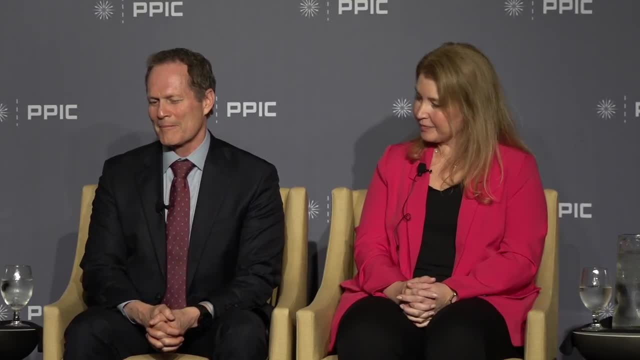 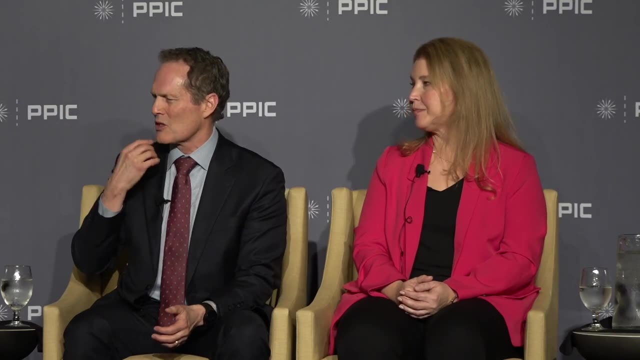 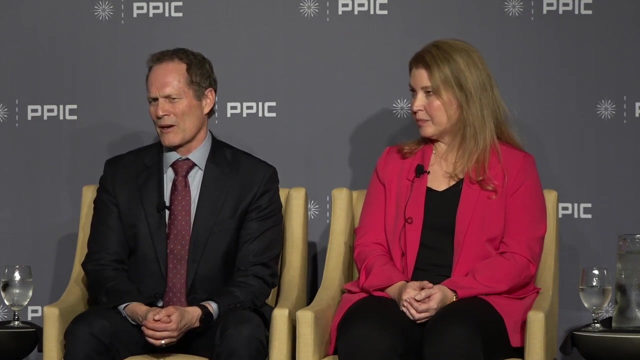 all related? I'm not sure, but I do know that inflation is going down, Which statistically is good for the economy, good for consumers, but consumers don't necessarily feel it. So, in terms of people's perceptions of you know where, 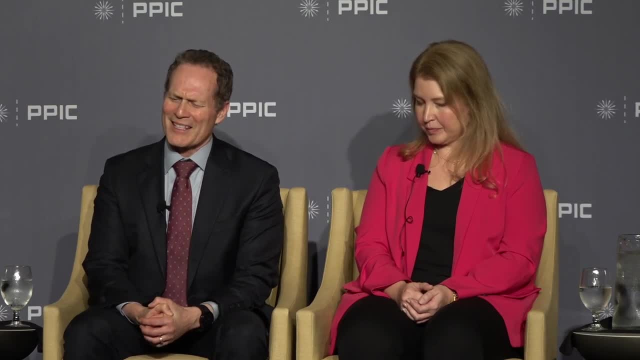 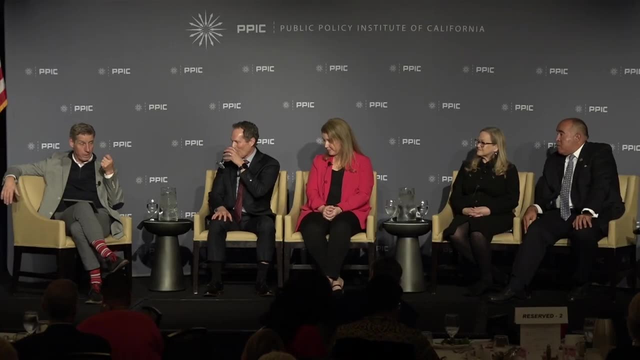 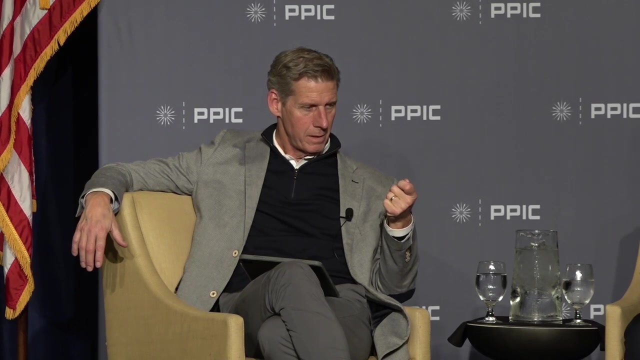 the economy is and where it's headed. it's a. we don't have enough time to go into the actual question, So let me put a slightly sharper point on that question, And it goes like this: Do you believe businesses are responsible for where California? 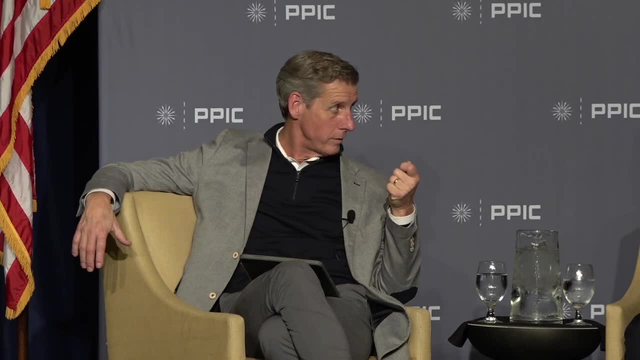 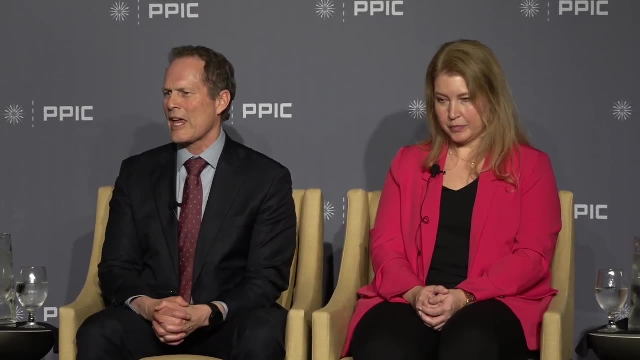 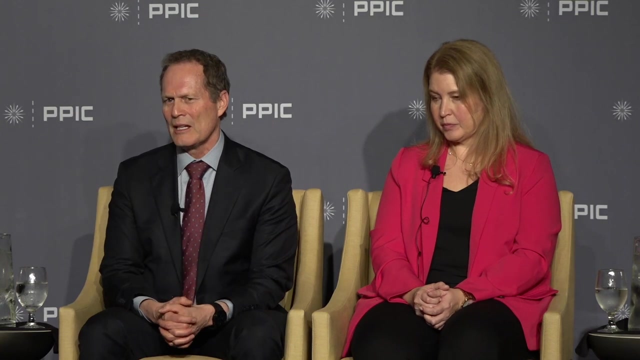 finds itself today and what is their role in the solution? Yeah, businesses are part of the problem, part of the solution. I mean you can't grow an economy without a vibrant public private sector. I mean you need a vibrant private sector. 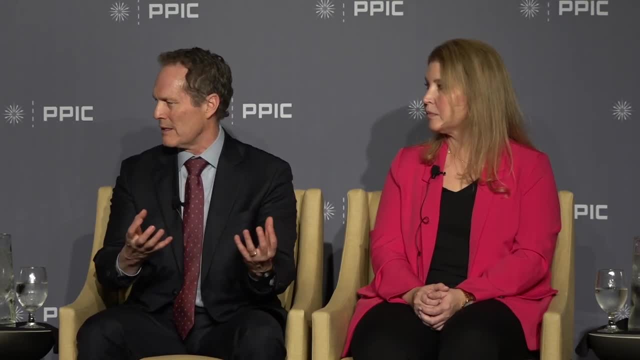 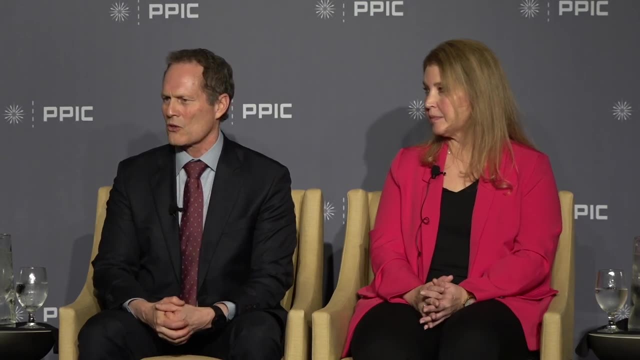 which, as I think we all know, is mainly small businesses. and then you have Overwhelmingly- not mainly overwhelmingly- small businesses, Overwhelmingly small businesses, and then you have large corporations that are going to do what large corporations do, which 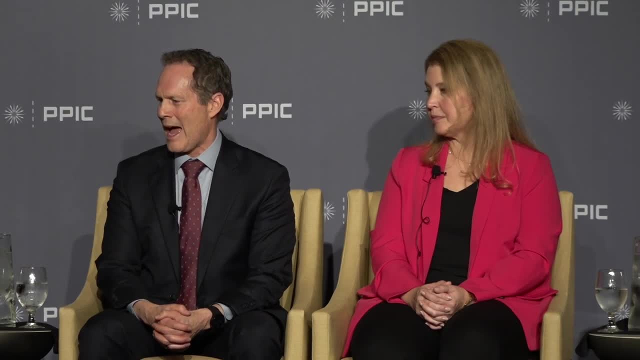 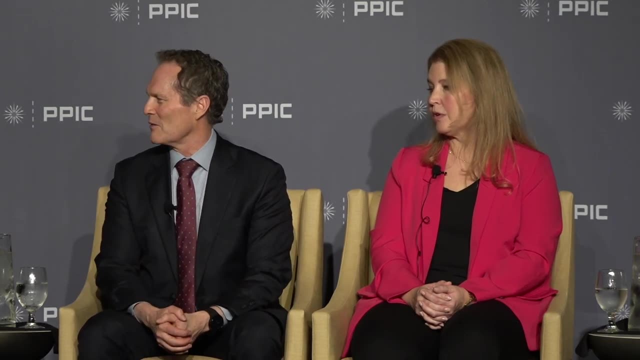 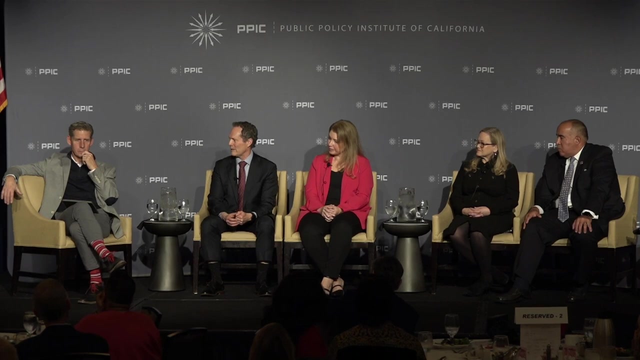 is, you know, consolidate aggregate and, yeah, in many cases create a large profit. But you know, I'll leave it to the regulators. They're pretty good at their job in terms of the laws and regulations governing kind of how regulated industries. 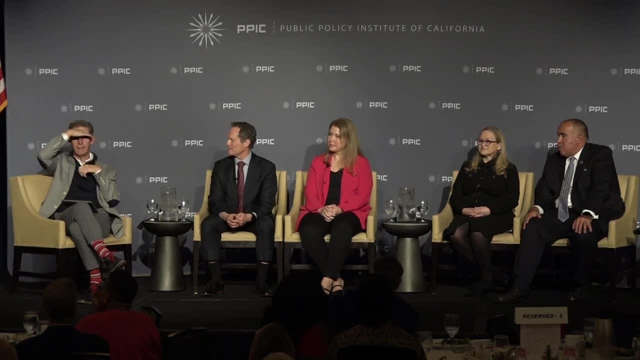 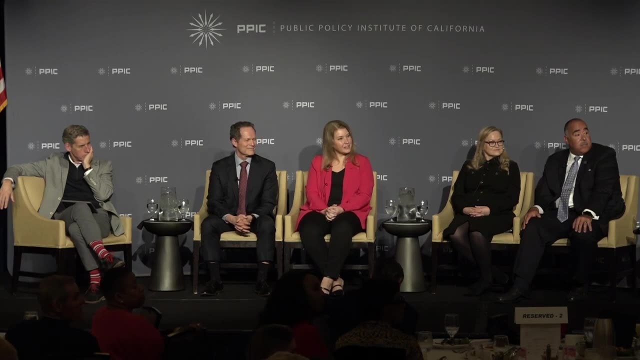 are supposed to behave. Alright, we'll go out again. There we go all the way in the corner. Thank you, Hi. I'm John Downs, I'm a member of the California Association of Professional Scientists and I'm hoping you can. 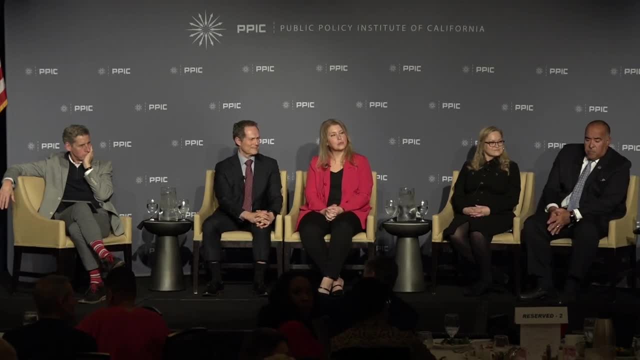 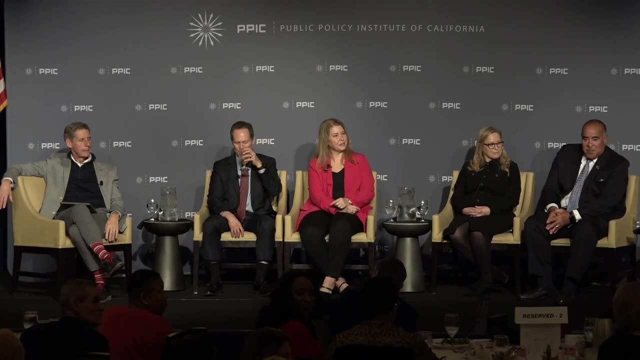 help me understand this multivariable question that I've gotten. Oh man, Scientists and multivariable questions. So we have this Politico article recently that was talked about making downtown great again, getting workers back into their offices. We have this DGS dashboard. 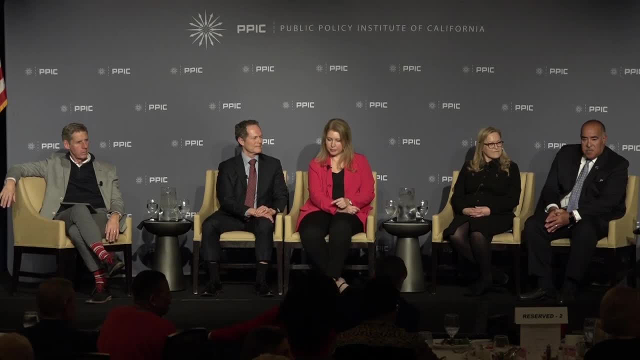 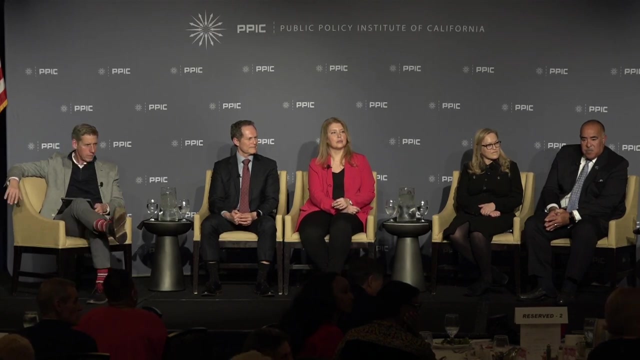 that kind of touts how remote work has. you know, with remote work productivity is up, pollution, traffic congestion is down. We've got kind of this equitable access to jobs now that people can do it from their homes, They don't have to drive. 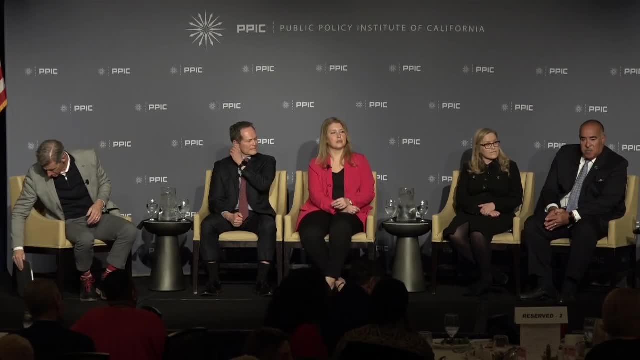 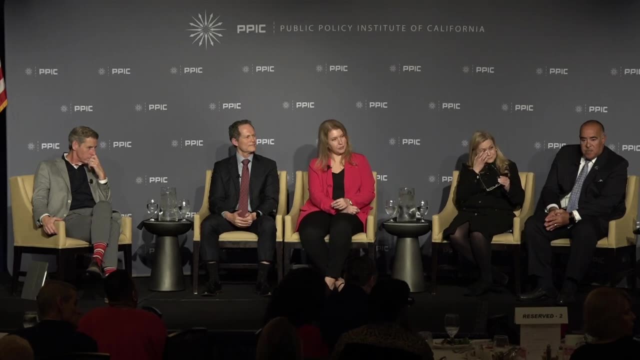 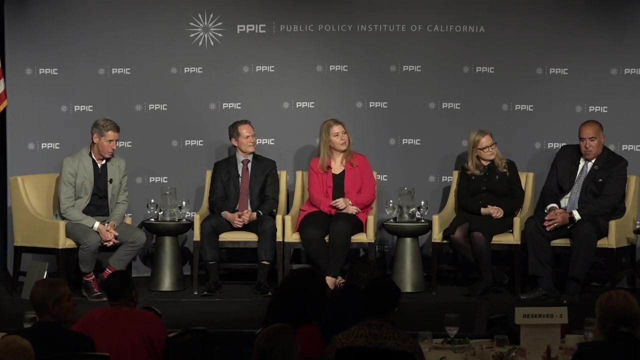 in. They don't have to pay for childcare. The cost of housing near where they work is now not part of that factor. Reduction in commute times and kind of that burden of commuting Help me understand this landscape of pushing people back to work and pushing the cost. 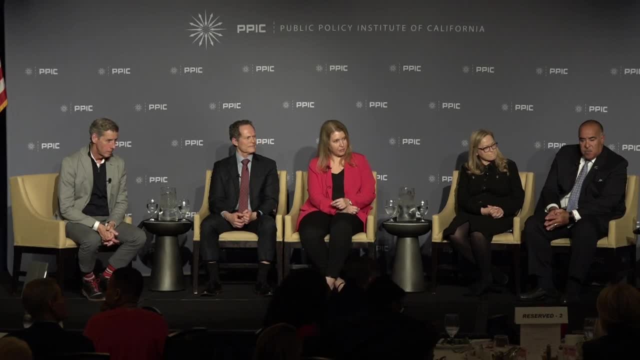 of returning to work on the employers- sorry on the employees- and not at their expense. you know, kind of using them as the stimulus package for local downtown businesses. Sarah, Well, that's a very interesting question. Look, it's a super complicated question. 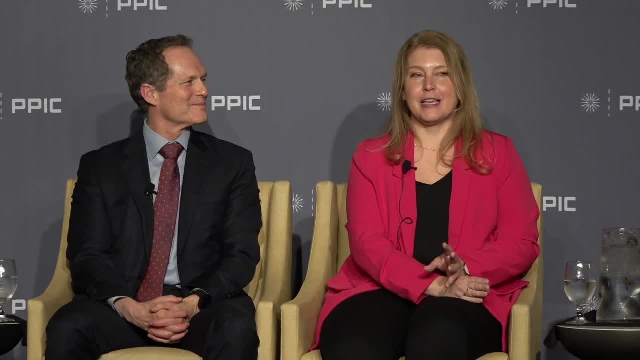 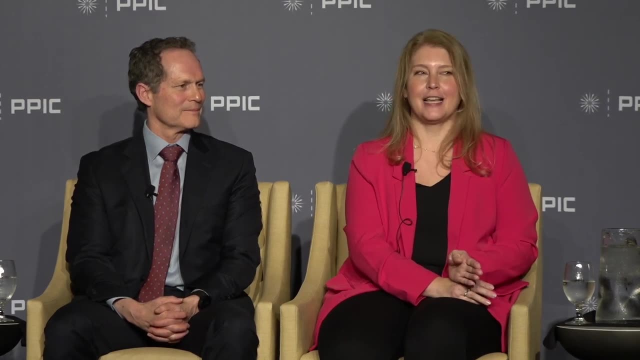 and you've got a minute to answer. Go. So. remote work was the biggest, fastest transformation in the labor market we've seen, probably will ever see, in our lifetimes. We went from 5% of working hours at home to 60%. 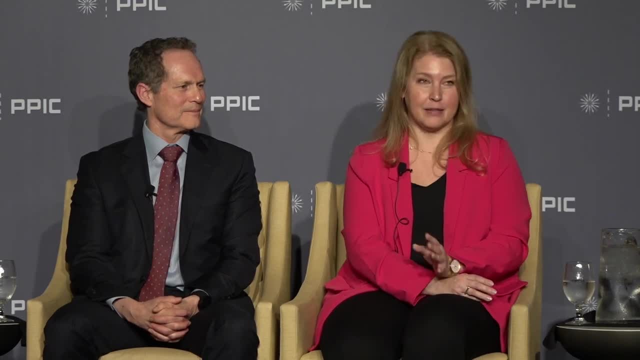 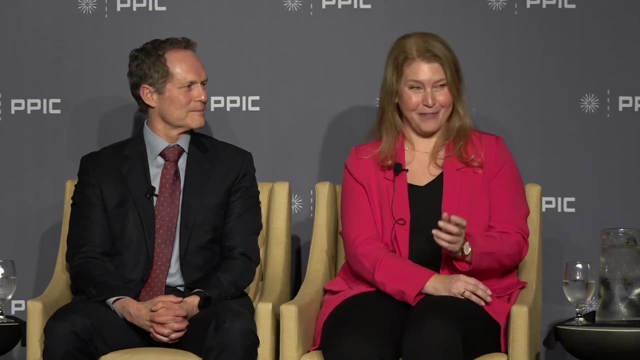 during the pandemic to 30% now and that's pretty stable right for about the past year. That's one to two days working remotely and workers say they want even more of that. But I think we're still in the midst of that transformation. 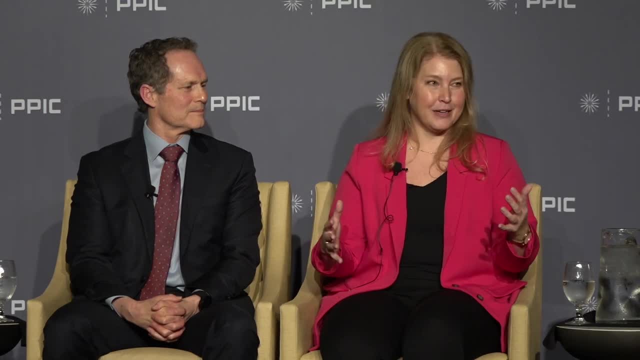 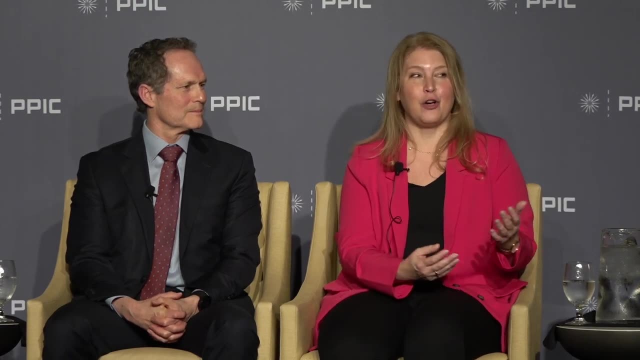 I think we're still kind of negotiating between workers, businesses, where we need to be, how we can be most productive. So I'm still watching it. I don't know the answer to that question. I know that it creates some opportunities for some. 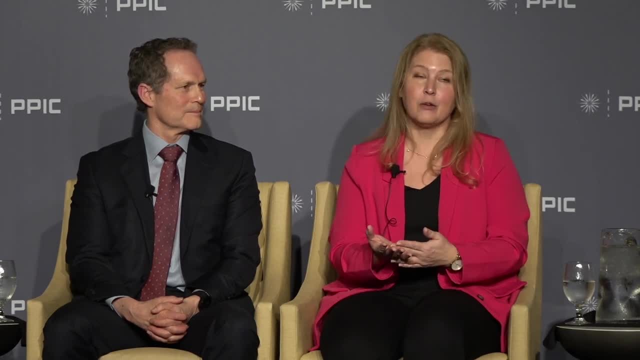 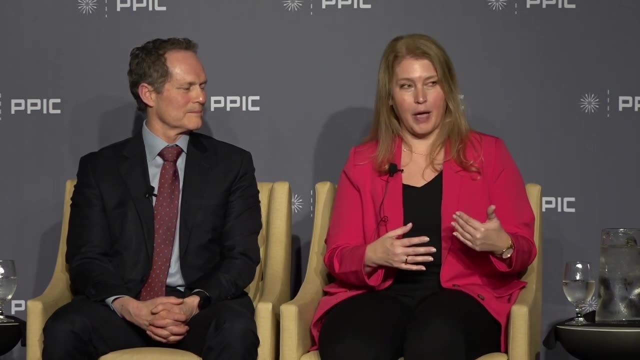 We see an increase in people with disabilities participating in work. There's some anecdotal evidence that could be because of the ability to work remotely, And same for women, whose employment has picked up more than for men, maybe because of the flexibility to care for children. 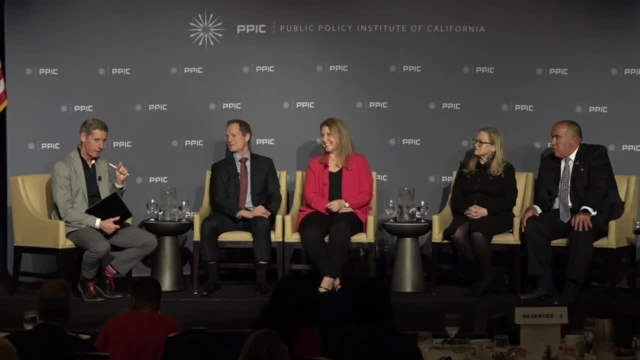 So lots that we're still sorting out in that space. Super quick anecdote and then a follow-up. My 25-year-old son said to me a couple of months ago: Dad, I am never going to work for a company that makes me go to the office. 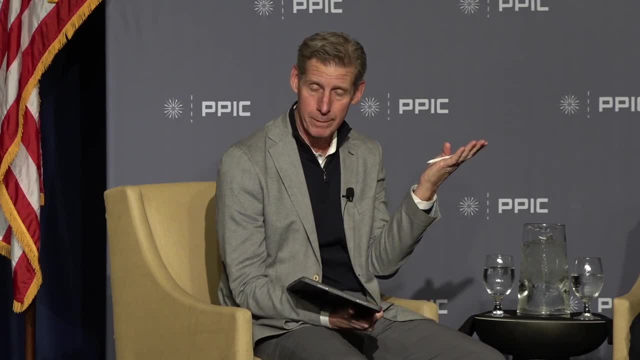 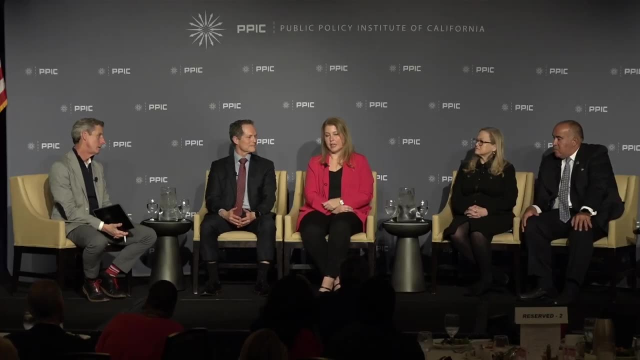 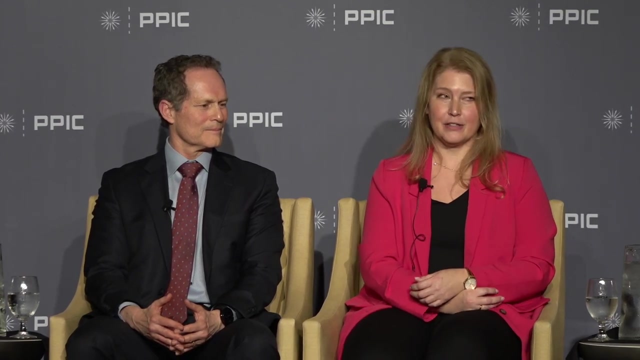 five days a week Can't blame him right? What does this mean for the future of California's economy, which is the subject at hand? It could mean improvements for workers who have access to that kind of work, But not everybody does. There's a lot of jobs. 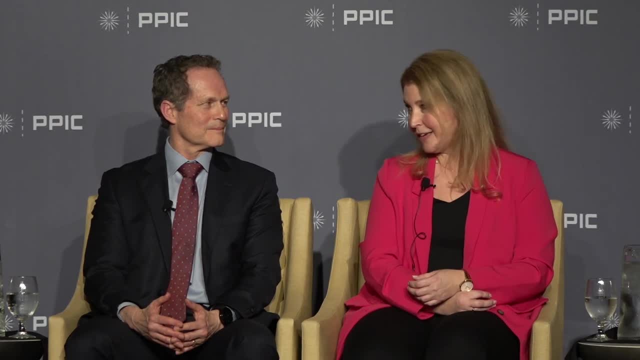 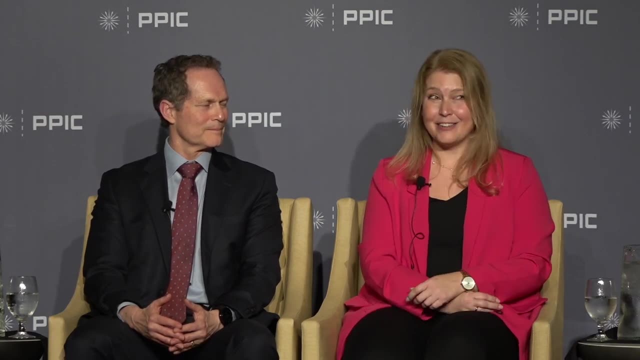 in sectors and businesses that are still face-to-face and will still be face-to-face. So I guess it's kind of a weak answer, but we're still sorting it out also regionally, Like you go to any downtown here in Sacramento. 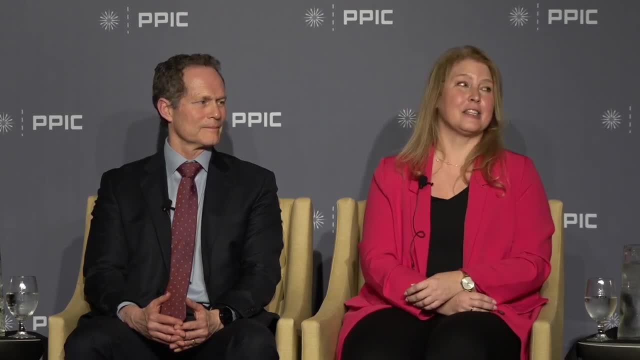 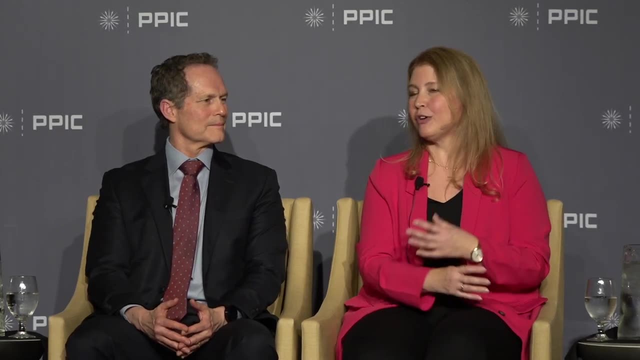 you see that we're still figuring out what that business district is going to look like, how the businesses that supported office work are doing. Are they moving to suburbs, where people are during the day, Or exurbs? That's still a process that's unfolding. It's a really important point. 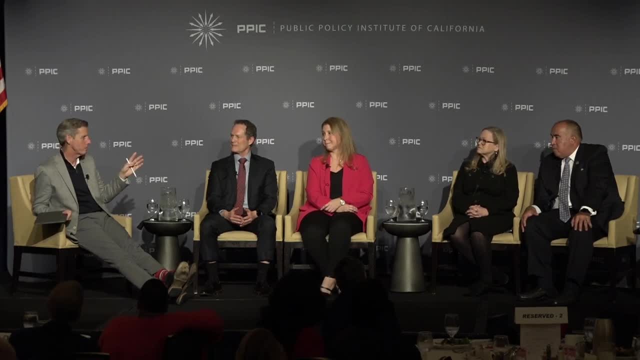 For as long ago as March of 2020- feels it was really only four years ago- which you know blink of an eye. We've got an online question, Steve, Thanks. This comes from our online audience and this has to do with attracting. 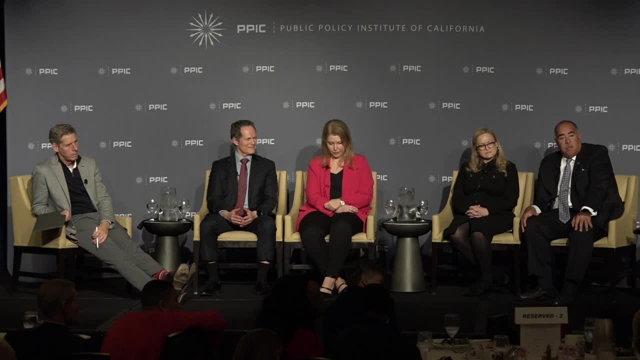 talent and capital to California. So this is Ashish from Idea. who's the President and CEO of Growing Inland Achievement? And the question is, in a recent survey published in the LA Times, California's national reputation as a place of dreams and prosperity. 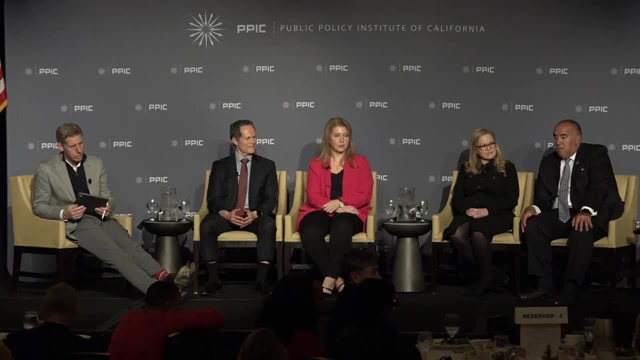 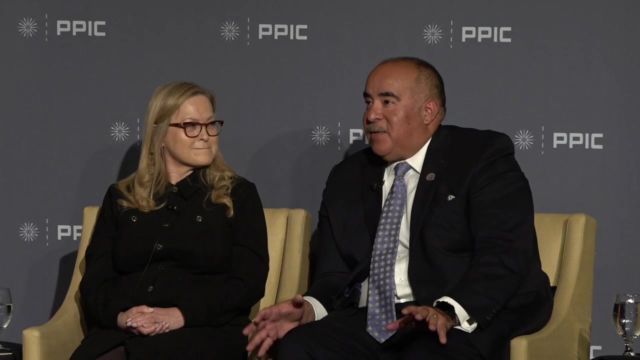 has been significantly tarnished. What specific economic and social policy should be introduced so the state can continue to attract talent and capital into the future? Paul, if you could wave your magic wand again as the economic development guy on the panel. What do you say? 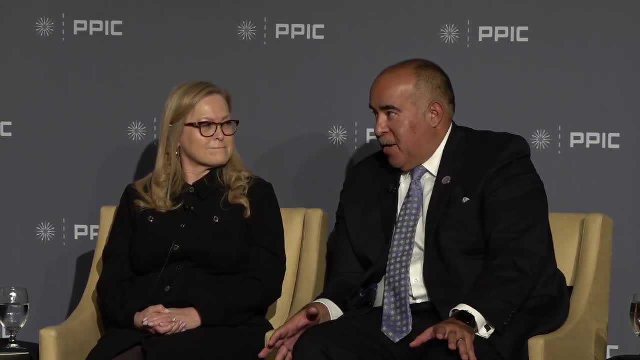 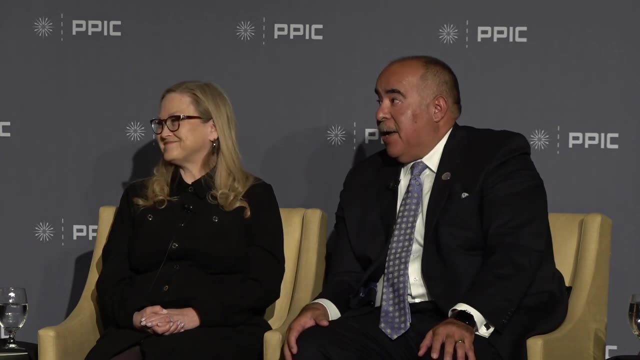 Well, first of all, you have to address housing costs, You also have to add in energy costs, And then you have to add in talent, right. And then I know we're going to get to the AI piece, right, But how is that going to change? 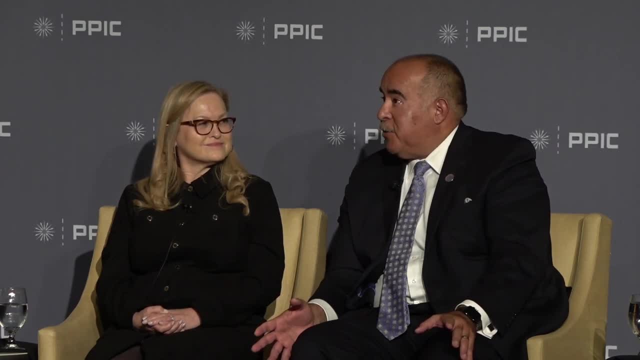 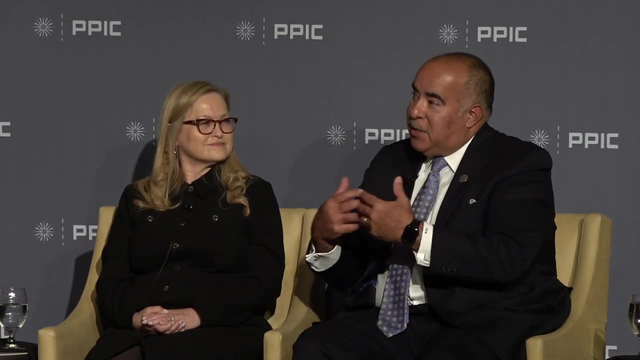 the workforce And give people opportunities, because perhaps they can do something that would be manual, but they'll be able to do it from an office location or even a home. So those things are going to change What California needs to do again. 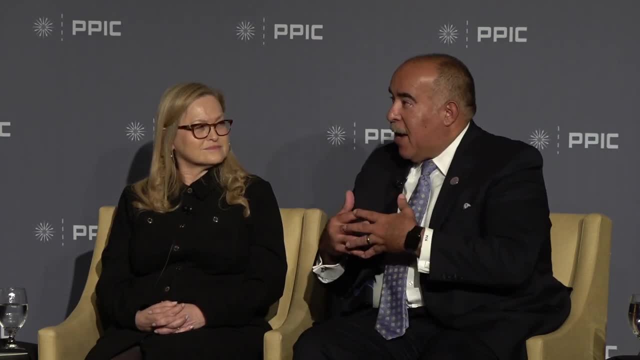 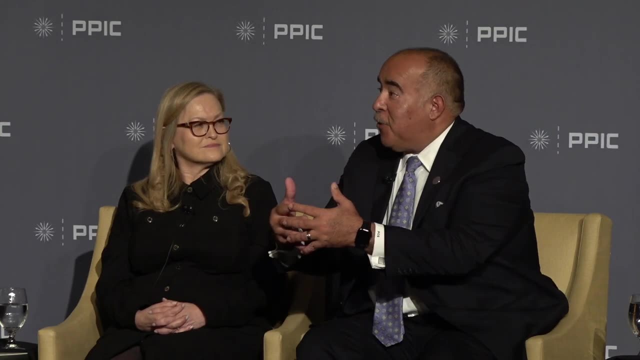 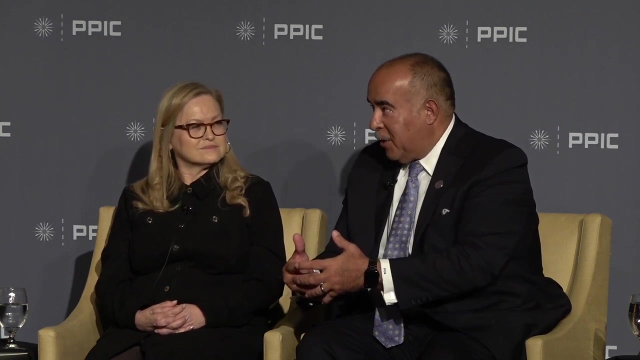 is double down. When I said education and workforce. I need to move a populace of 4.6 million from 21% baccalaureate to 35% And, at the same time, invest in those new technologies. What is augmented reality going to look like? 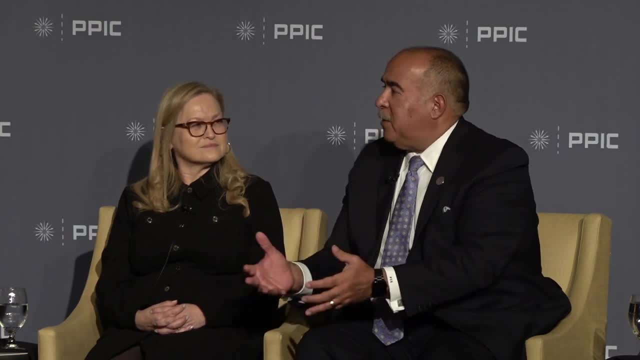 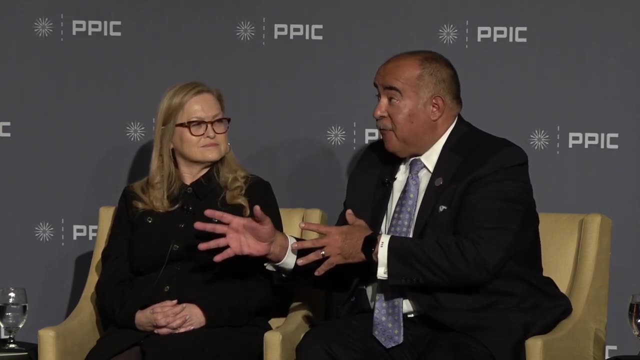 What is virtual reality going to do for our ability to lift things, move things? It's going to change the world in which we live. And, all of that said, if kids don't have the ability to get online, which many still don't- 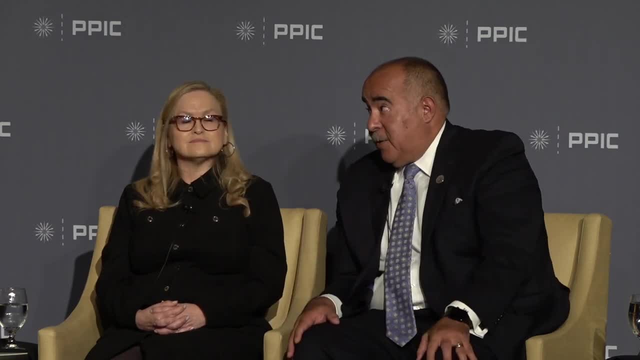 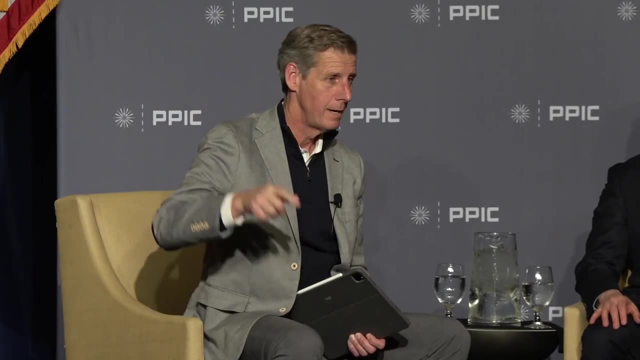 then that's inequitable. I'll ask this one from my colleague, Matt Levin, who covers AI for Marketplace: Raise your hand, Matt, so everybody can see you. There you go. So if you've got a question about AI, go to him. 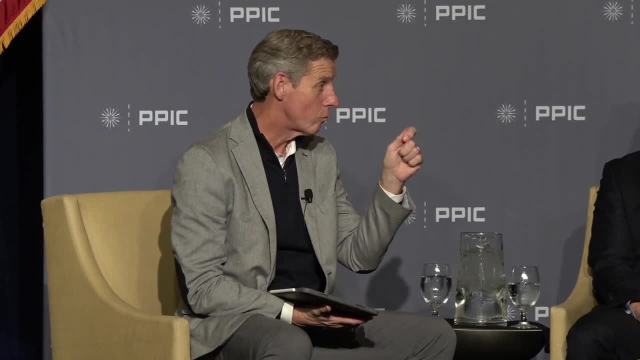 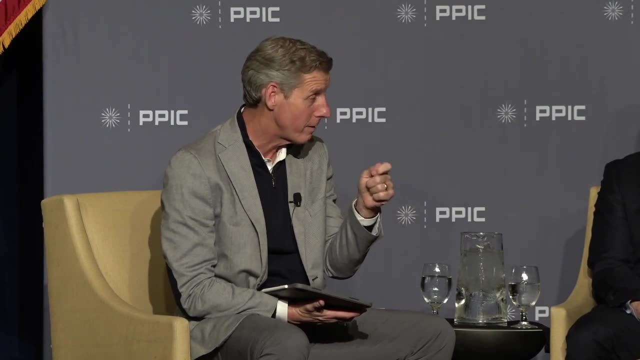 Here's the thing about technology. now, right, It's not robots replacing blue-collar workers in this economy, Ciara, It's white-collar workers being replaced, or the threat of them being replaced. What does that mean for the future of California's economy? 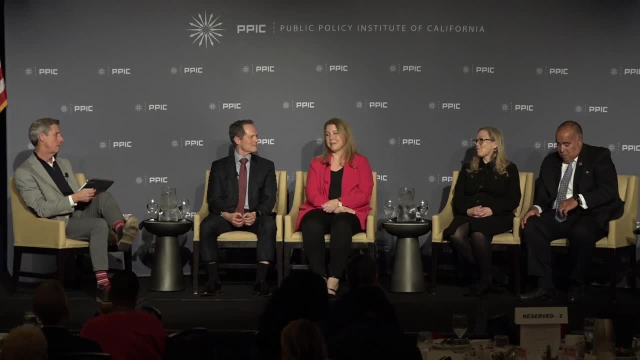 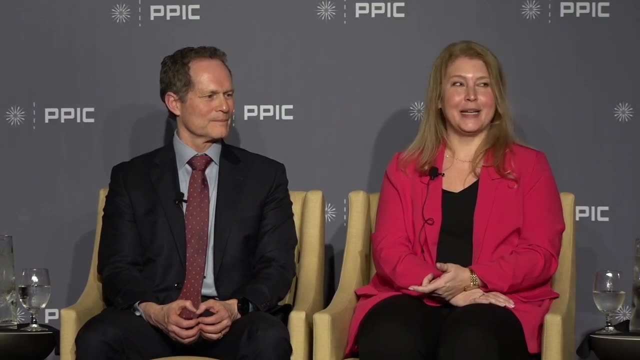 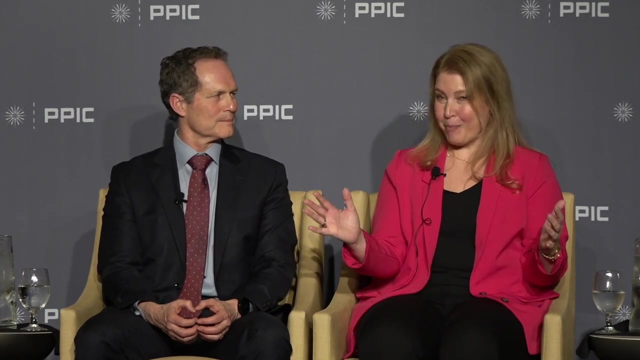 That is very interesting because we have been here before, but maybe we paid attention to it in a different way. As computers, as the information age also eliminated some jobs augmented, others created opportunities, moved them around. right, We're here again, but now there's like. 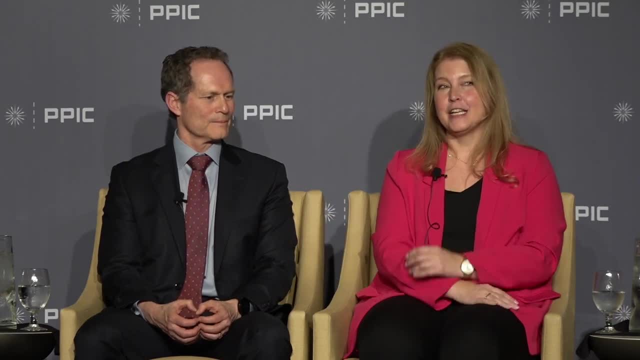 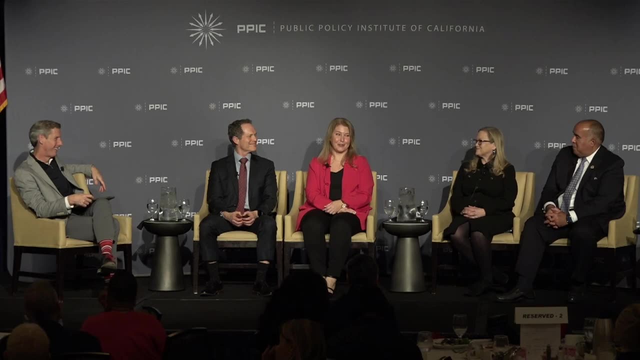 a broader scope of people and work and businesses. that might be affected Pretty much everybody in this room, by the way. just for the record, We do the numbers every day. people do that for us. So the question is, who are the winners and losers? 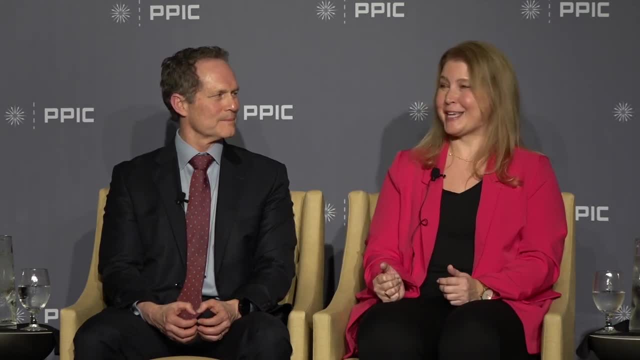 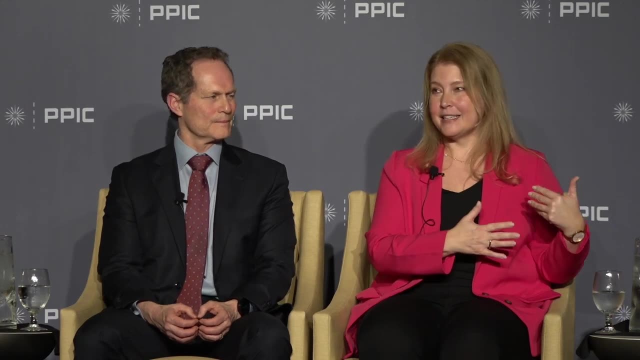 I think there's such a wide range of what this might look like, and maybe Matt has some scenarios we can run to think about. who potentially stands to gain and lose from this, What that then means for building into our educational systems, coordinating for us individually to know about. 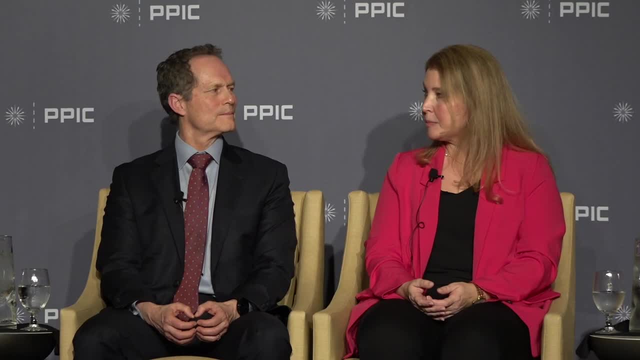 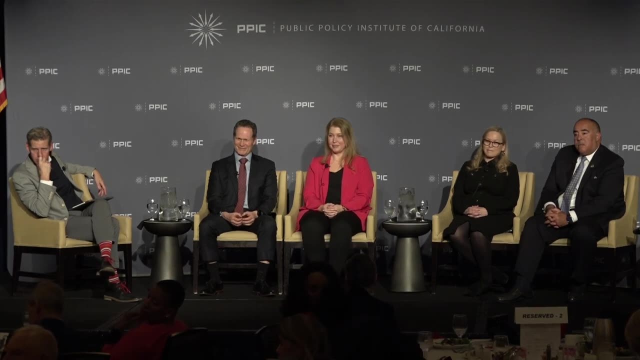 the future skills that will at least buffer us as much as possible In the middle Landa Ajose Waverly Street Foundation. The video package makes reference to climate change, and I think the energy transition that we're going to be experiencing is going to be as transformative. 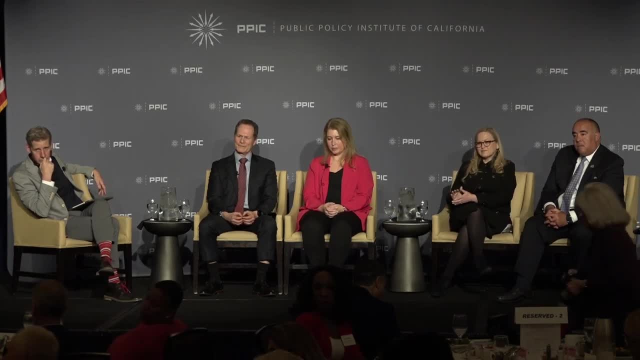 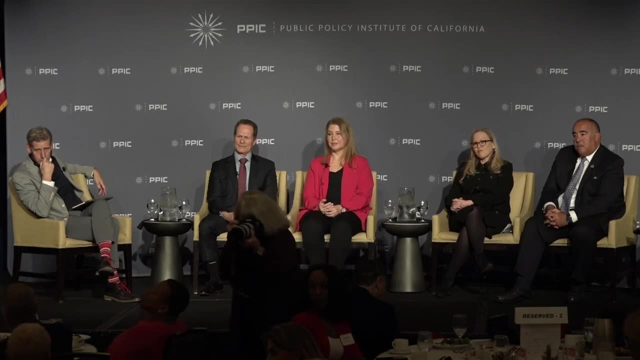 as the industrial revolution. I'm wondering if you can talk about what you think that means for the California's economy and particularly what that means for workers. I think about places like Richmond and I think about places like Kern County, And it's going to be transformative. 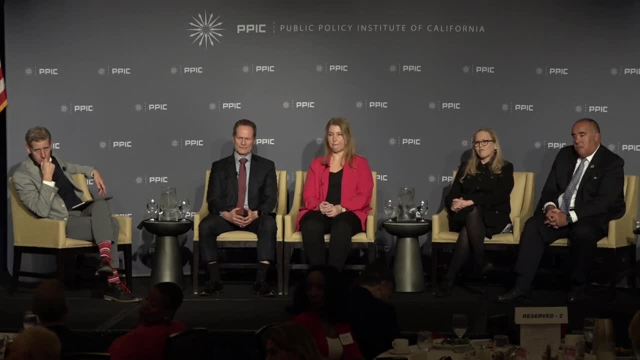 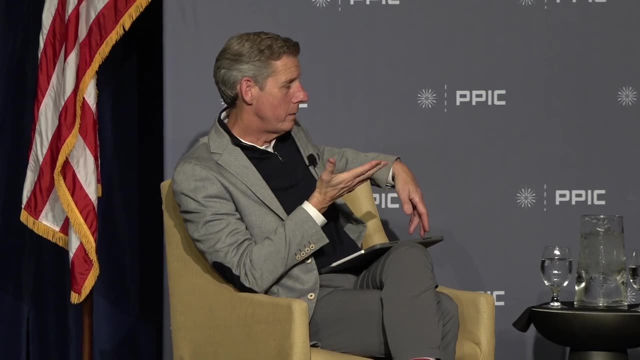 for workers, and I think that there we have the risk of elevating income inequality or solving it, and I wonder how you all would respond to that. Let's talk about it in Santa Clara County, shall we? So I think you raise a really powerful point. 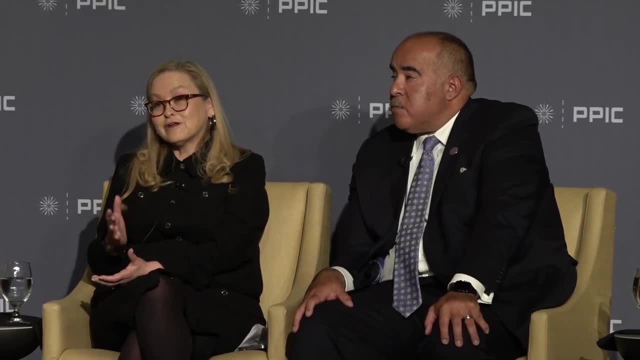 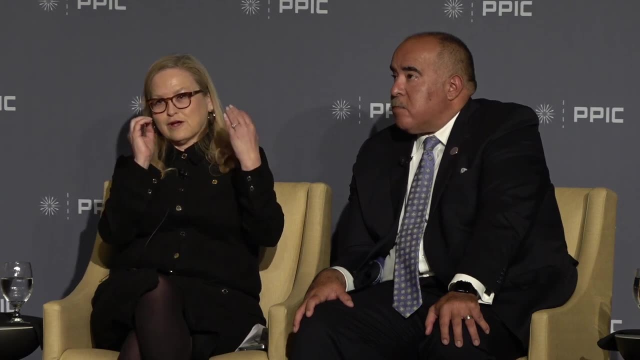 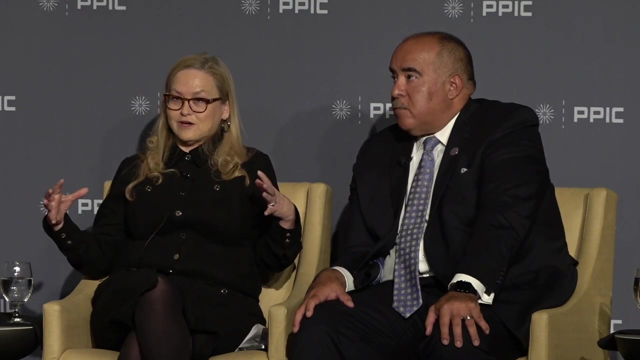 and this goes back to my goal of having a big plan, and one of them is that in California, if we go back to the days where Governor Brown I was building highways, if we are in the building infrastructure, there are many, many ways we can do that. 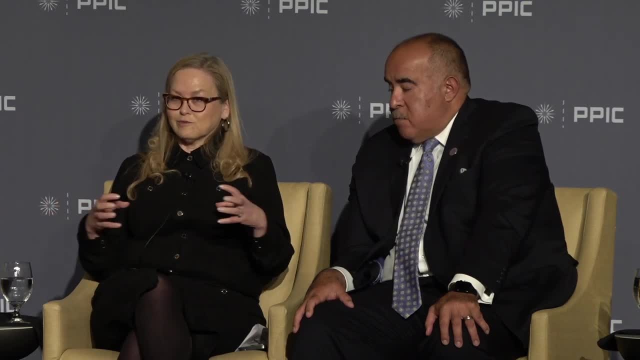 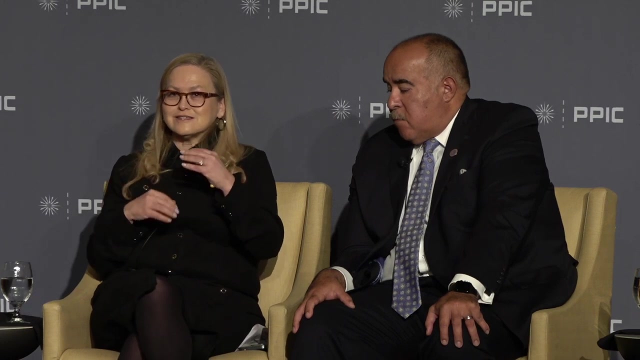 One is being the most connected state in the world. if we were really to invest, for example, in broadband. The second would be to recognize that we have green jobs coming online every day in the transportation sector, And so one of the challenges that I see is that 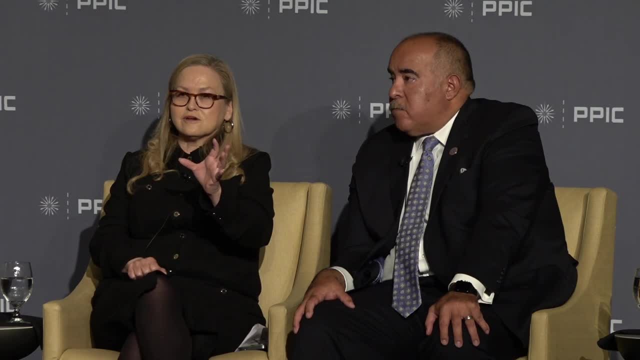 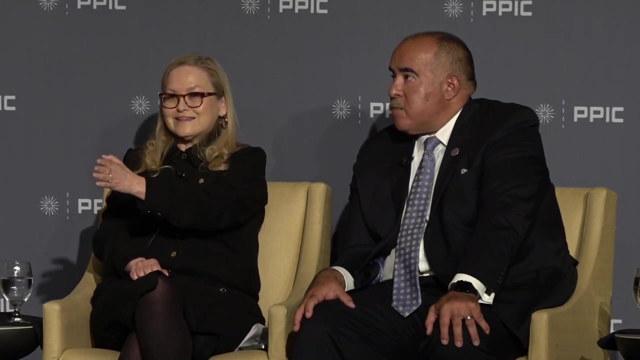 we- and this really goes back to the point that Sarah was raising- is that in real time, our ability to train people to do a good job where they make a high wage now and we're looking at high wage jobs in the future- that sector. 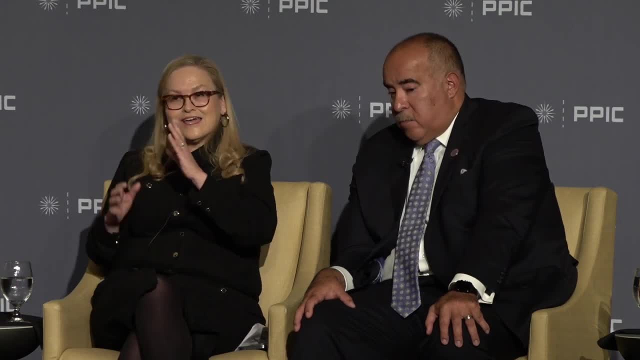 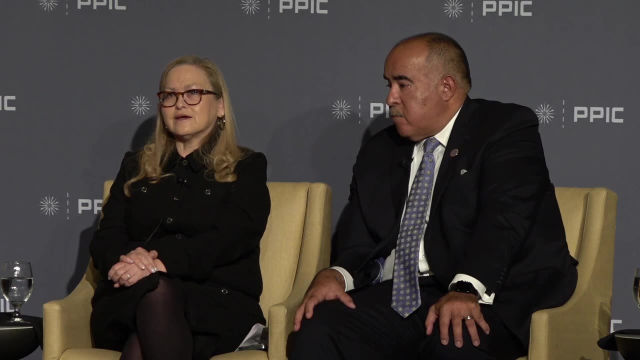 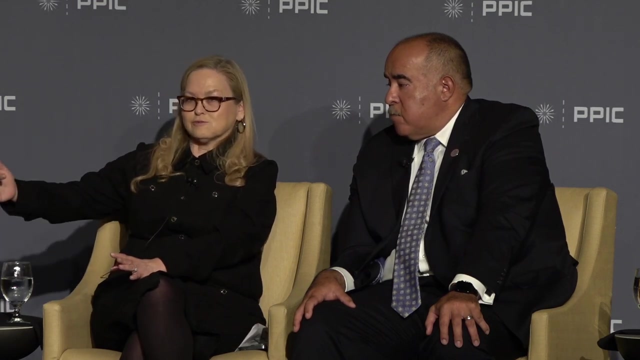 exists today It does, And again I'll just use transportation as one example. In the nine barrier counties where I am, we are looking at, I would say, maybe $20 billion a year in infrastructure development in transportation, And so some of this. 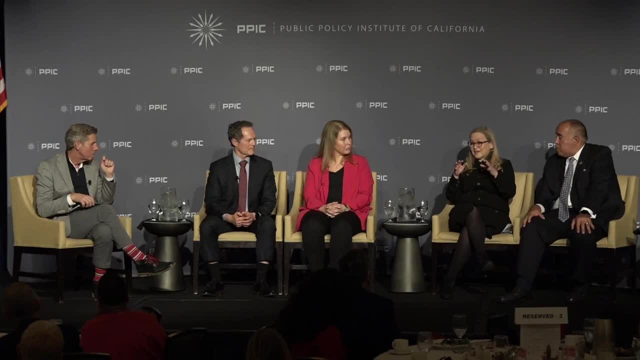 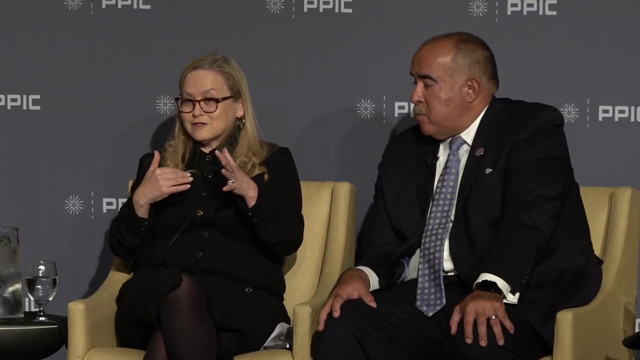 is us rethinking the structure of our environments and recognizing that. again, I'll tell you, the folks in Richmond get pretty hot at me because of some votes I took, but- and the reason is they understand this- that from an economic perspective, if we're 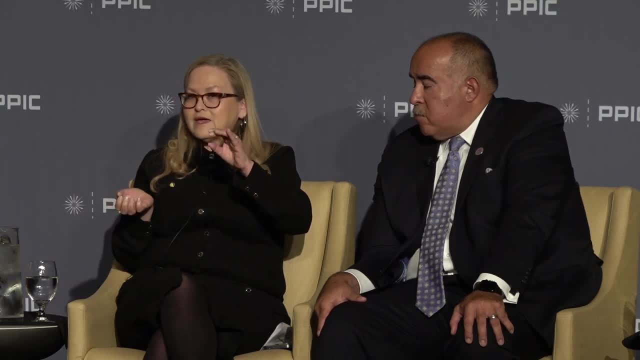 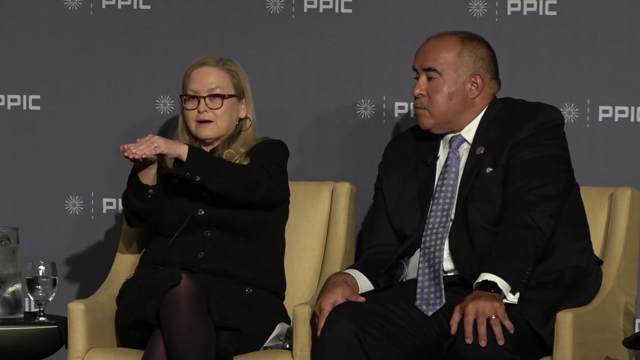 really thinking about protecting these communities, then we are making the to your point: the alignment, the policy alignments that allow one job to fade and a new job to come, online with the training and the support people need to get to the new job. 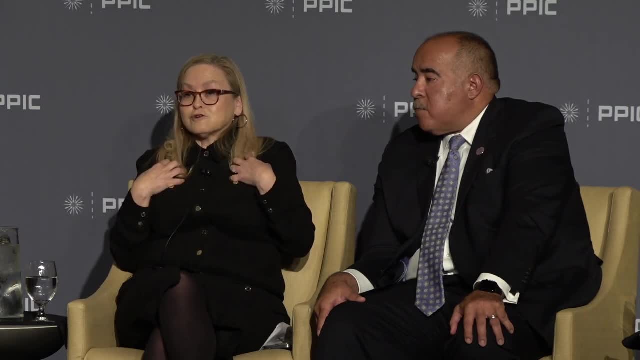 And we haven't done that in a way that the American worker trusts us. I don't mean just government, I mean trust the economy to do that, because we are punishing to people at the bottom rung. We just we are punishing to them. 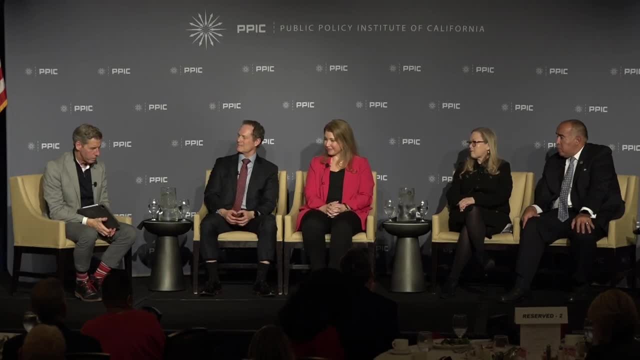 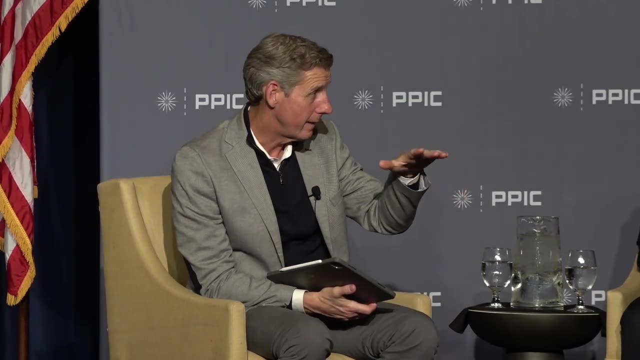 Sorry, Paul, moderator's prerogative here. just on a related question, I think no offense to any of the other three of you. you're probably the person closest to being actually on the ground and talking to people participating in this economy on a day in, day out basis. 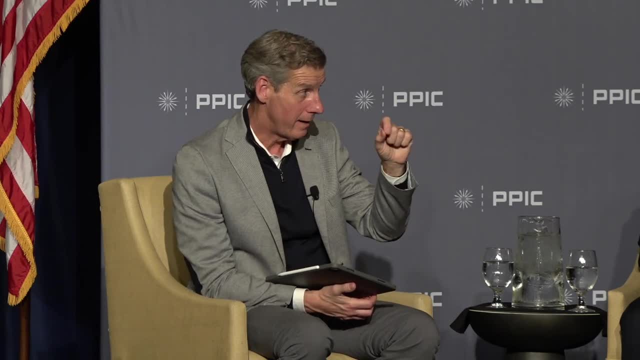 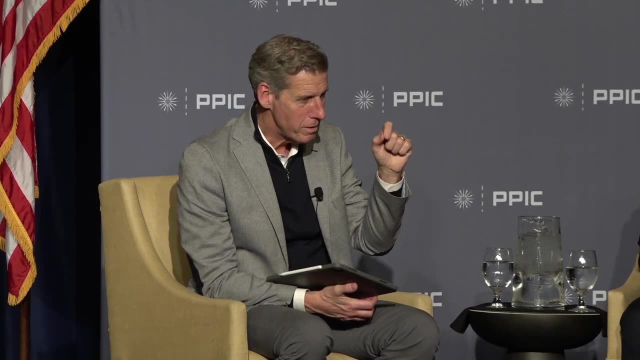 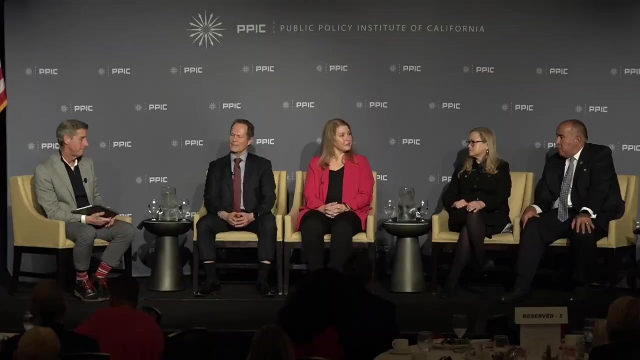 With what you said about people leaving and the average age of people- Latinos- in the empire being 17,. do you think it's not like the apocalypse is coming tomorrow, but do you think we have enough time to get this right? Well, we better. Otherwise, the apocalypse is possible. People need jobs, and we have to remember that an economy is a complex thing, Whether we like it or not. we need corporations that employ a lot of people, provide healthcare to a lot of people and give people. 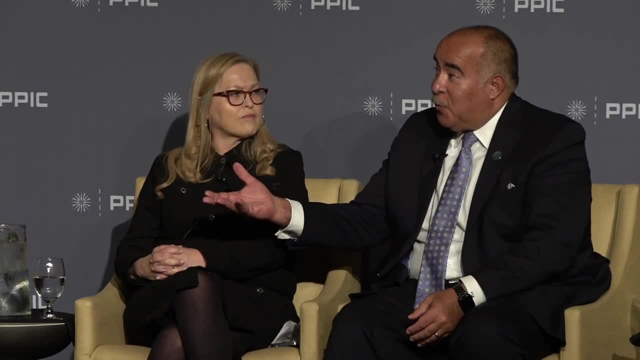 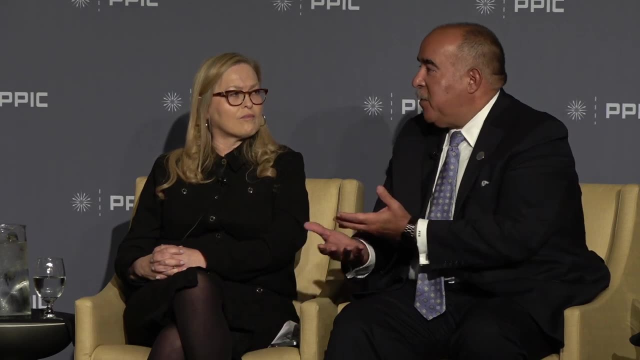 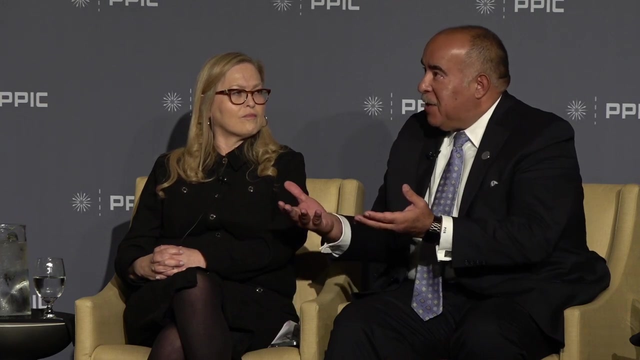 a path to the middle class and beyond, And so that voice is something that we need to have. we need to hear because of the tectonic plates underneath everything we're talking about And the people who just believe that this is the greatest country in the world and they should. 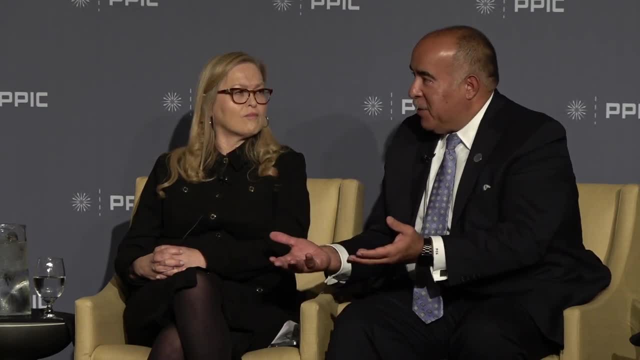 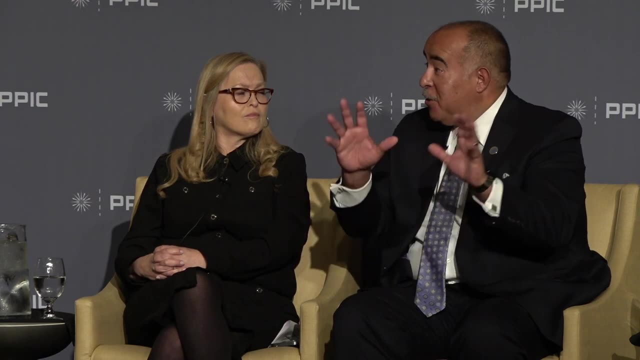 have an opportunity to do as well or better than their parents. they're worried. right now I've got a 12 year old daughter and I don't know. yesterday it was Disney characters on the wall, now it's K-pop boy bands. 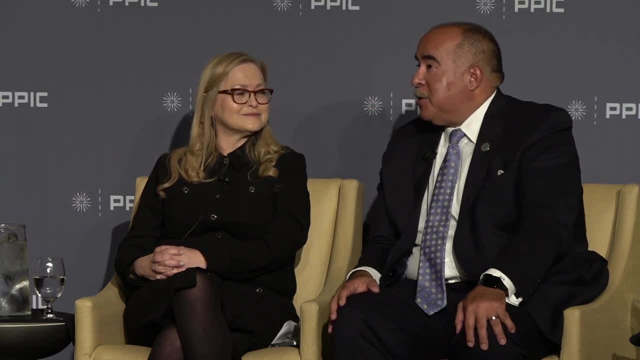 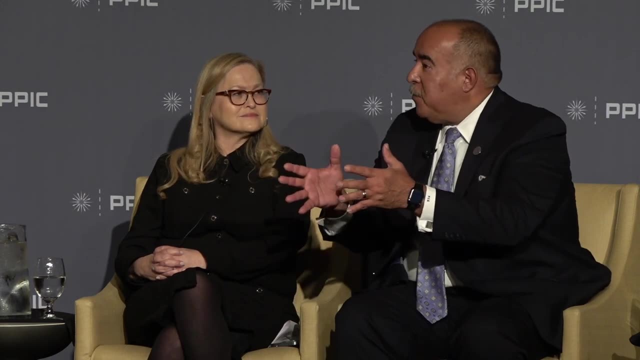 But I also know the things that she, the questions that she comes to me about news, right, And she's listening to you, right, But she's getting that from YouTube, right. She's getting it from different channels And there's got to be a way for us to. 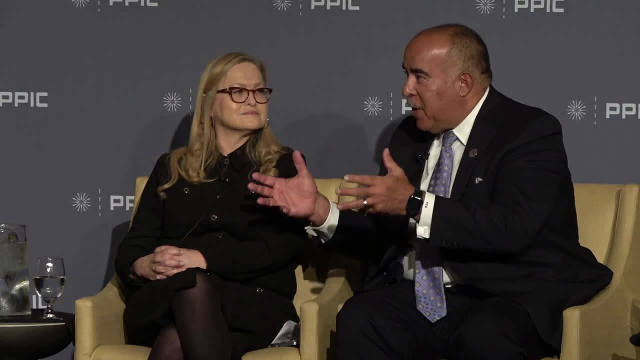 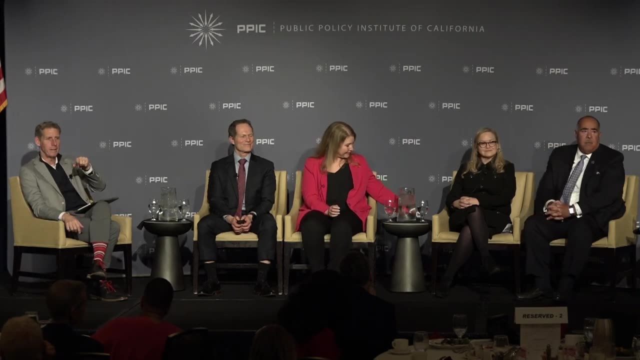 maximize that to make us smarter and better and more competitive. Good news is: the tectonic plates move slower right. Last one in the back there and then I think we have to be done. Thanks everyone for being here. I work for the State Assembly, so the PPIC. 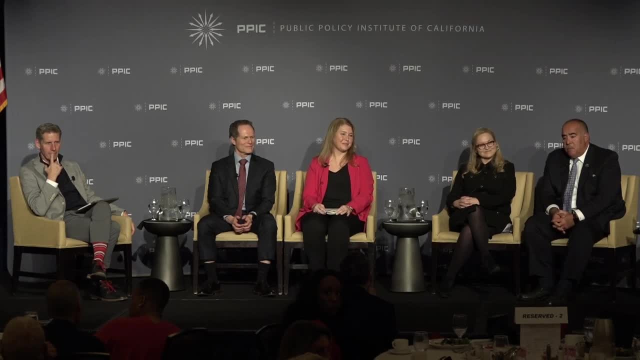 reports are a super great resource for us, Really excited about the new Economic Policy Center. My questions for Dr Bone mostly, but for the panel and I guess at large I think there's a lot of folks, especially my age and younger, who are skeptical of economics. 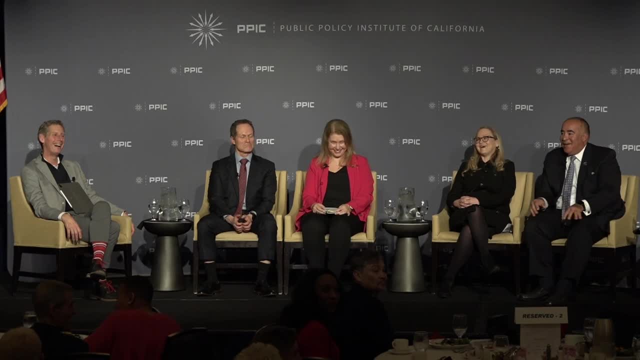 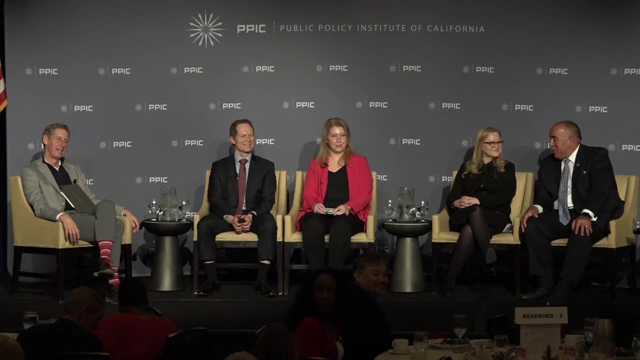 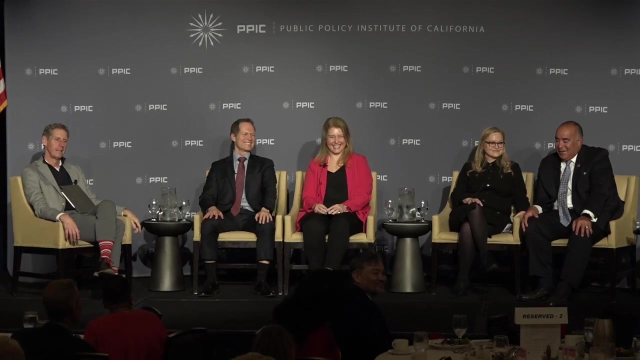 as a field and economists as a profession, Because they have these lived experiences that do not always mesh well with the kind of abstract charts and data that economists make their living with. She's one of the good ones. However, how will this new center try and 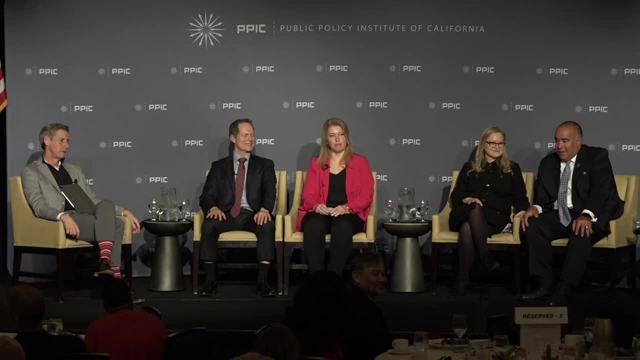 kind of bridge that gap for folks that are having real world experience in all of these different issues from housing to healthcare? How are you going to make sure that you're actually explaining some of the market forces at work to people in these fields and try and 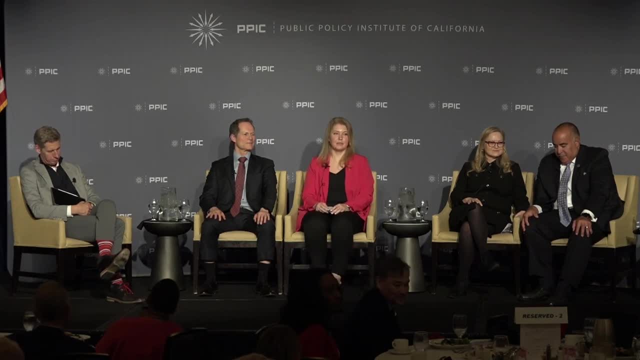 kind of bridge that understanding gap, Because I think that a lot of economists are actually trying to work and make these things better but aren't always kind of. they're kind of disregarded out of hand, just for what economics has been historically. I am 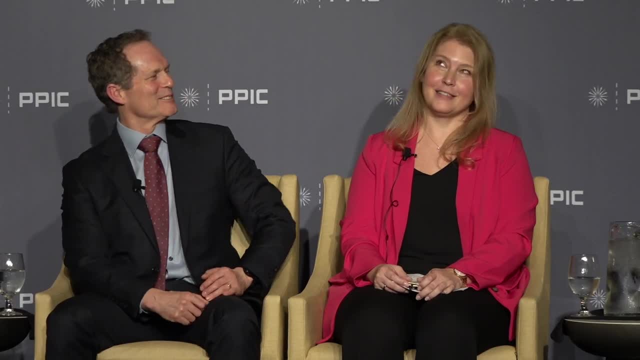 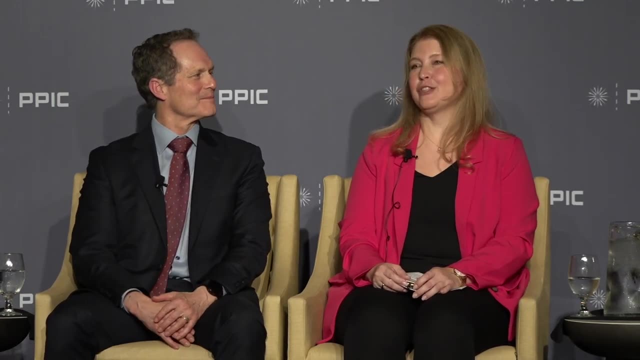 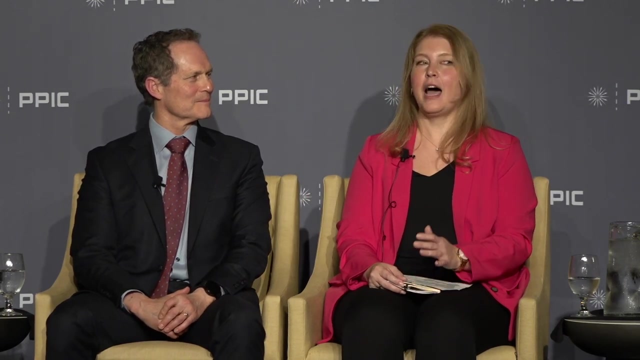 with you on that. honestly, I think we've had a few years of lots of forecasts that were not accurate And in general, when we look at kind of economic statistics and all the indicators that we talk about, that tells one story but it's not the whole story. 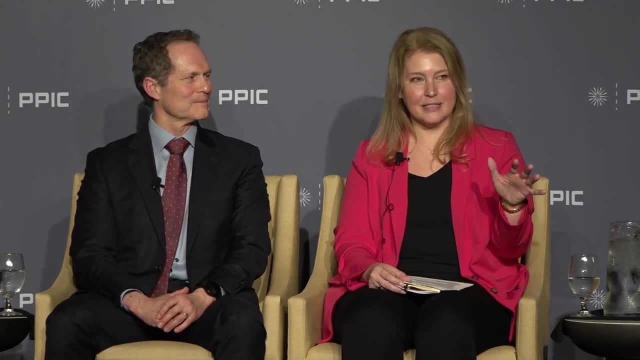 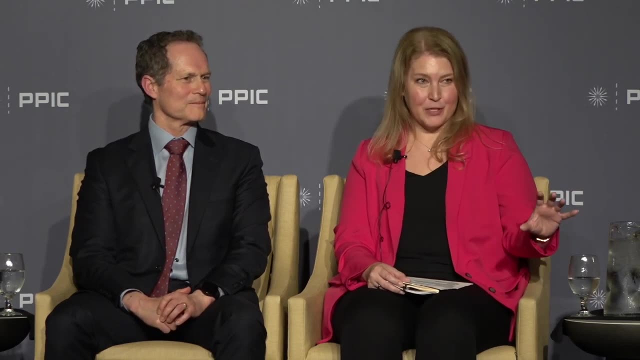 as I said earlier, We need to look at the resilience of the economy and performance of the economy overall, because that matters for how we can all do within it. But we need to look at how individuals, how businesses, how workers are doing, And so what we're. 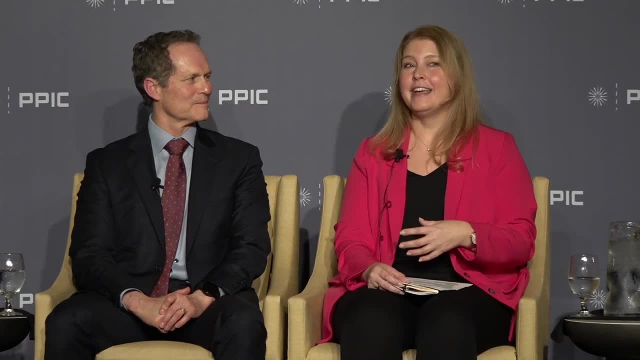 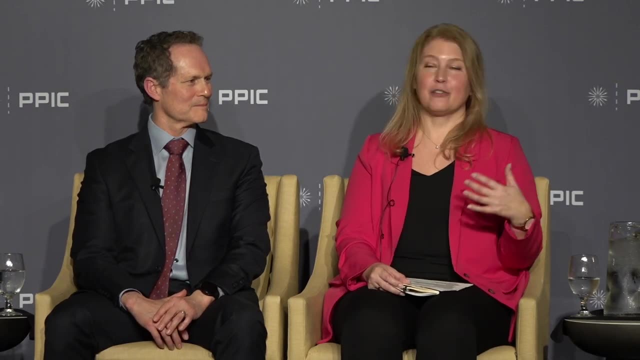 going to do at the center- and hopefully you see that in our materials already- is tell that broader story, to think about how it works for different people and how it doesn't, what barriers we face across the state, across the various regions In a 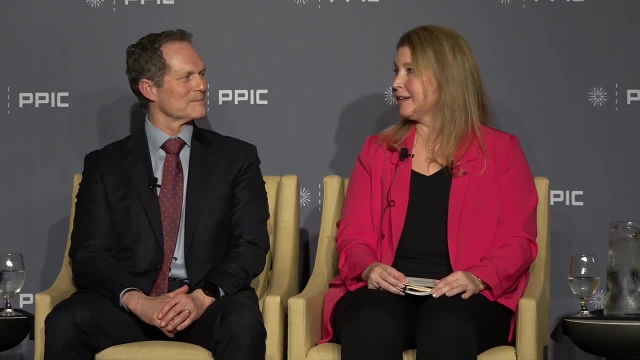 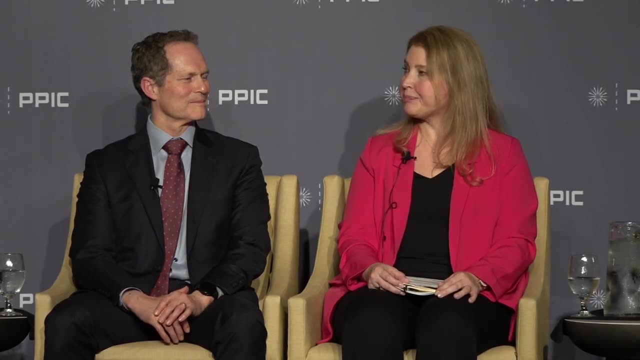 diverse place. that's a challenge, But we're feeling ambitious because we believe, along with you all, that this is critical for our future state. The floor is yours. You're in charge now. Thank you, Kai. I'm going to close this out in just a couple of minutes. 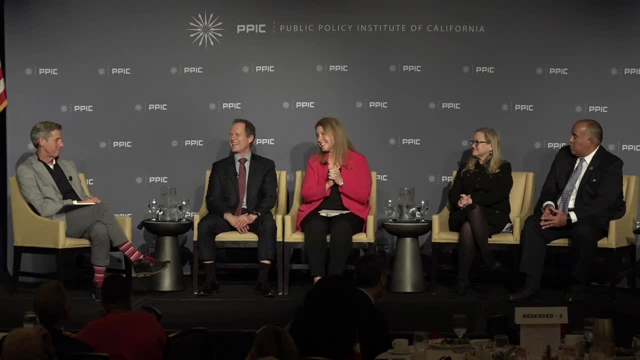 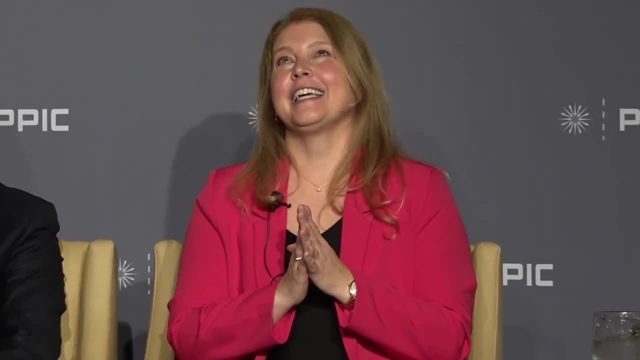 but I'm going to take the privilege to turn the tables on Kai first and ask him a question. see how he likes being in the hot seat. So the question that I have for you, Kai, is: we've talked about a lot of challenges. 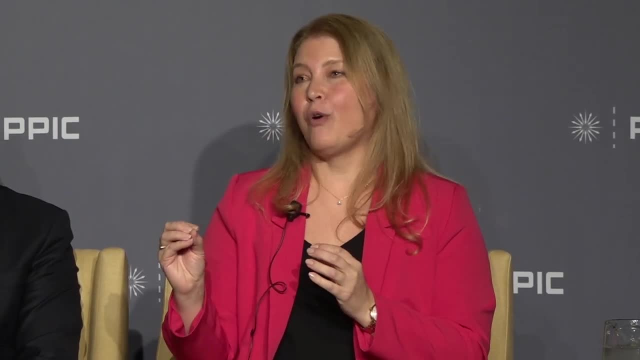 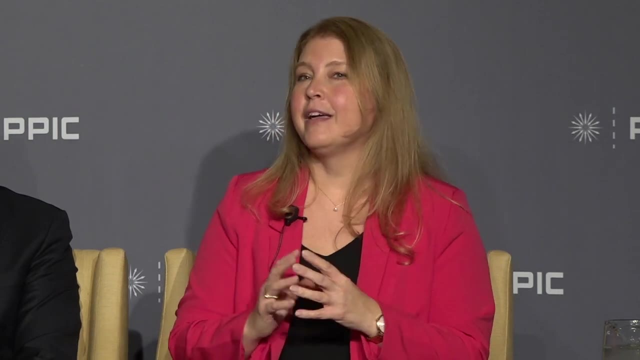 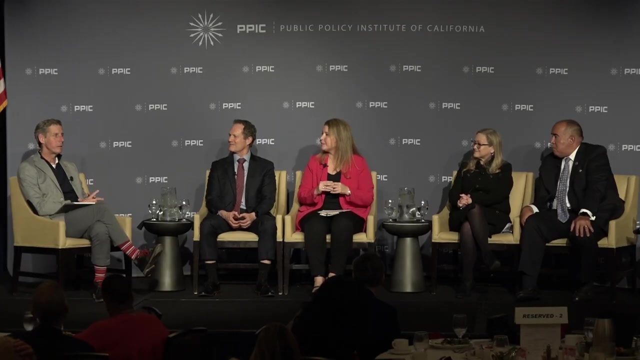 for California. What will you be looking for, given you have such a broad perspective on how the nation is doing, even economically, across the globe? What will you be watching for to know if California is headed in the right direction? Easy Narrowing of the wealth. 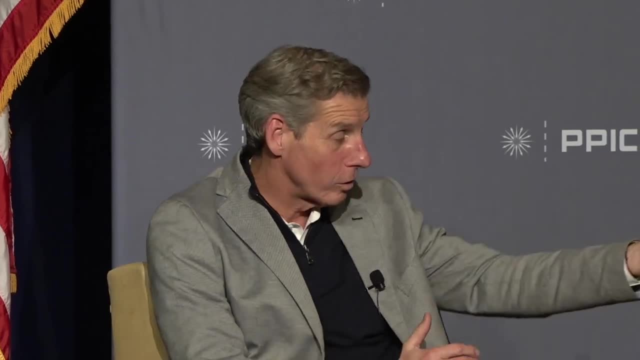 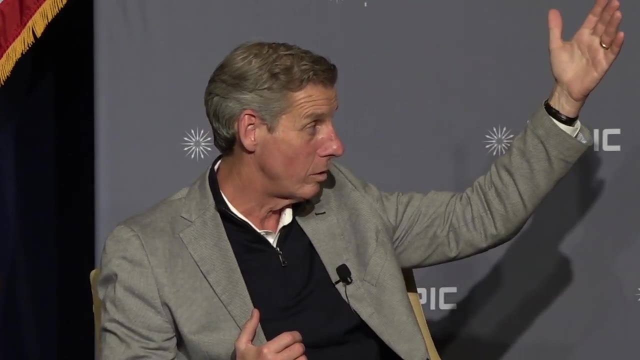 disparity. There's such wealth disparities. I mean, look at Cindy's Supervisorial District right, Or the Santa Clara County right, Stanford, with multi-gajillion dollar homes down to Gilroy, where you know agriculture workers who are the heart of this economy. 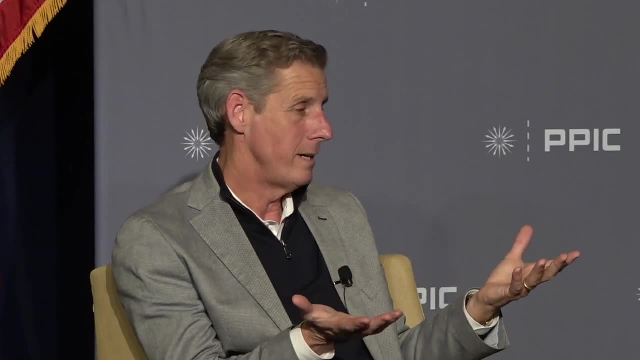 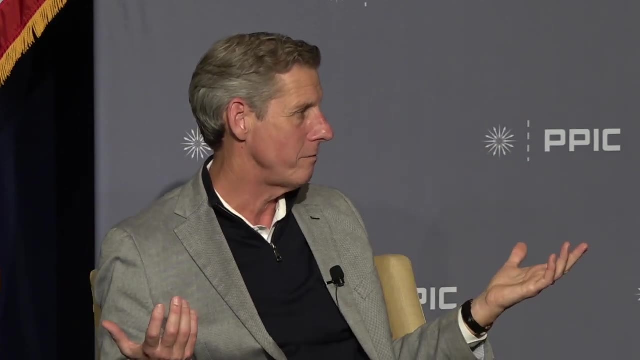 in many, many ways can barely afford to get by right. So if we can narrow that and we don't have to move the house from Riverside across county lines to gain a million dollars in value, then I think we're getting somewhere. The catch is: 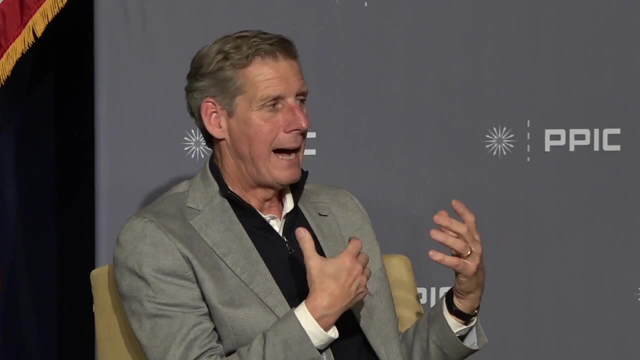 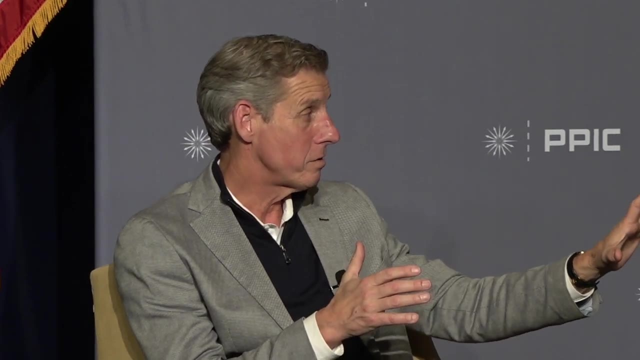 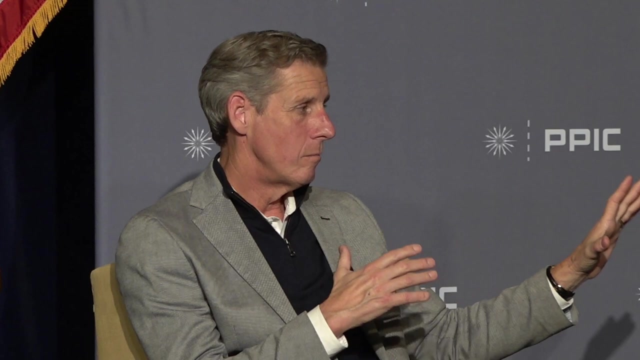 and I ask this question because I'm genuinely curious. I don't know how much time we have with younger people leaving, with all possible respect, politicians afraid to make many of the hard decisions that are required with corporate America. again, all respect, more interested. 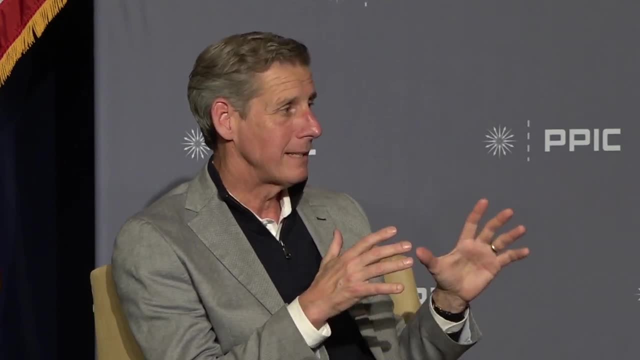 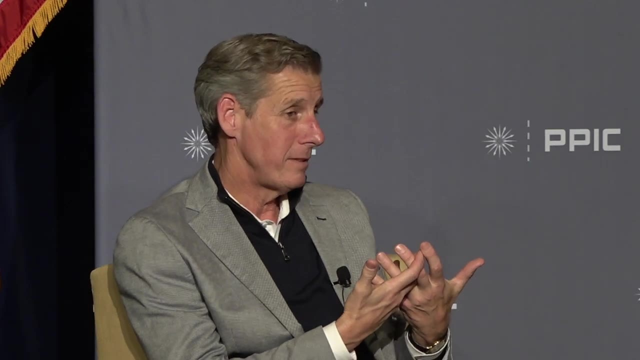 in the bottom line in many cases than actually getting the people who participate in the economy to be elevated. it's a real challenge. It's a real challenge. Look, I've been in this state now 25 years. I remember. sorry, I'll take 30. 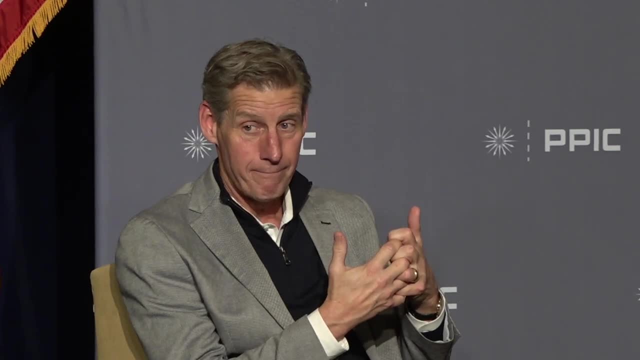 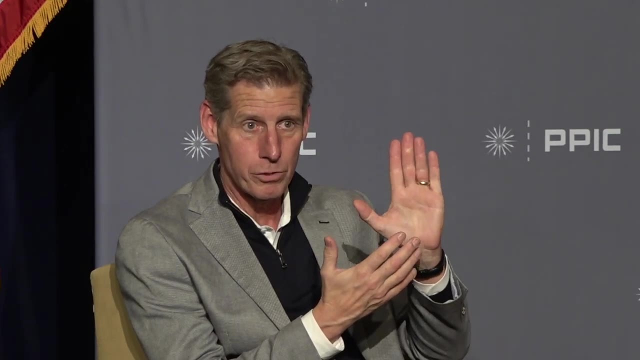 seconds here. When I was in sixth grade, I got detention after school. Phil Schatzel, the math teacher, gave me detention because I had done my homework. Swear to God, this is a true story. Hadn't done my homework. 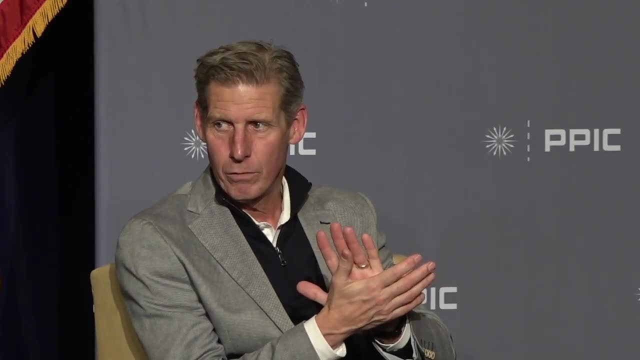 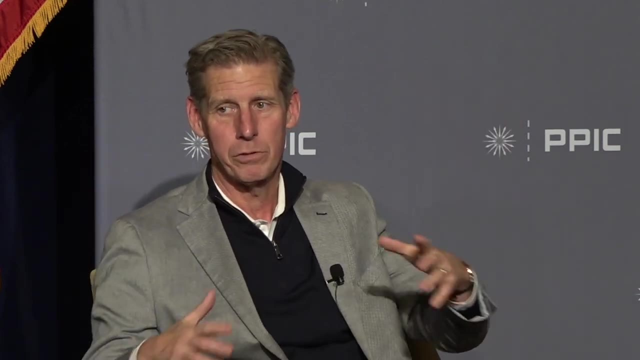 Mr Schatzel also was doing the eighth grade variety show that week, And so I had to do my detention in the auditorium where all the eighth graders were doing their song and dance routines and this and that And one of the eighth grade band. 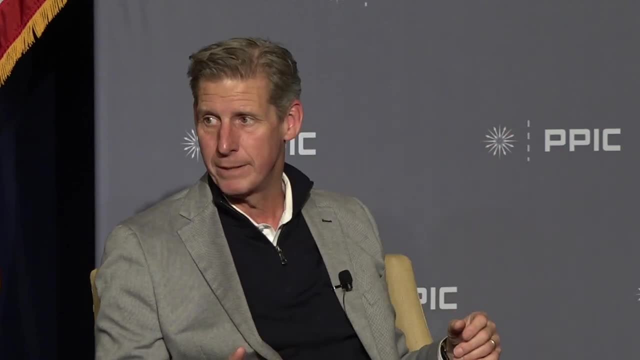 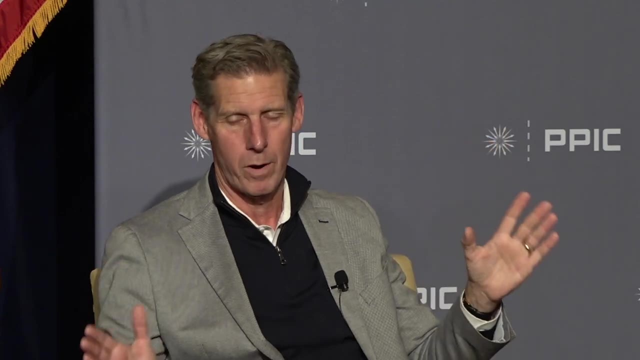 groups got up and did California Dreamin', right. And I'm like: this is Briarcliff Manor, New York, in freaking February. right, It's snowy, it's gross. the snow on the ground is mushy, no leaves, what have you? 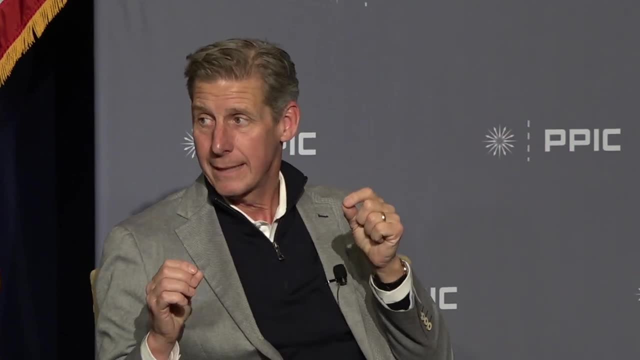 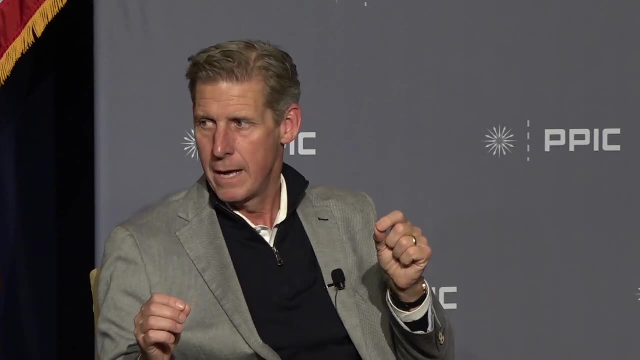 And all I could think of was: wow, California sounds amazing. If you had told me 40 years- okay, 50 years ago- that I'd have been sitting in Sacramento or living in Los Angeles having a conversation about the future of the state. 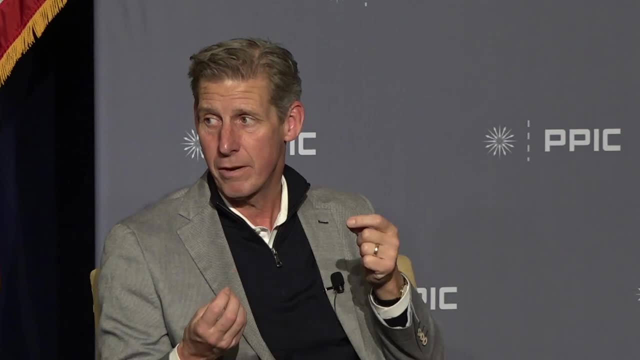 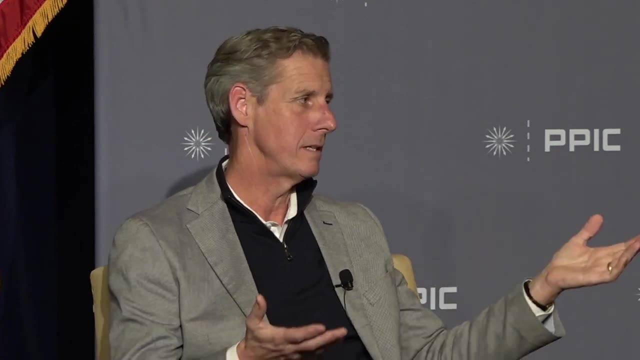 of California and what the potential is for this place. I'd have told you you're out of your mind, But you have to believe in it Because we've done it And the question is: can we do it again? That's the answer to the question. 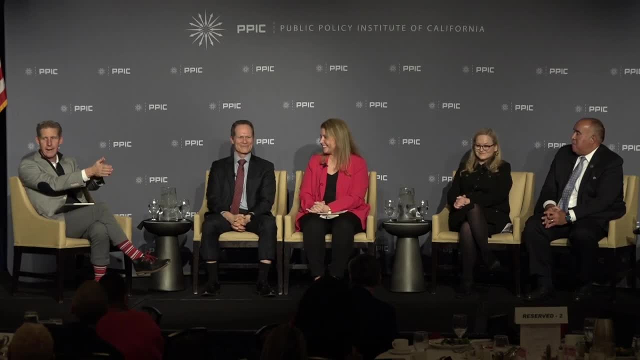 So my clock says 1 o'clock. I'm getting the. you gotta go sign. I thank you so much for your time. I thank the panel for your answers and for your perspectives, And I thank the Public Policy Institute for having me up today. I appreciate it.